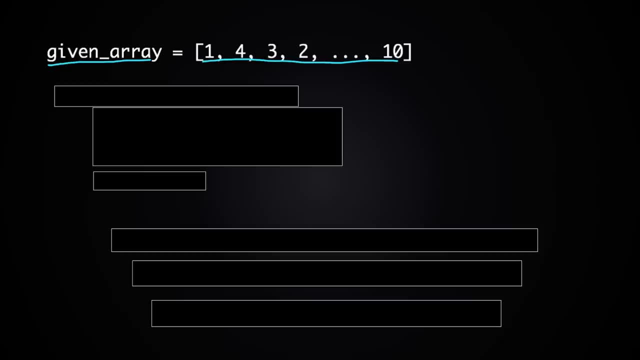 100,000 elements And let's say you want to write a function that takes this array and returns the sum of all the numbers in this array. So in your function you want to add up all the numbers in this array and return the sum, And that function might look like this function right here: 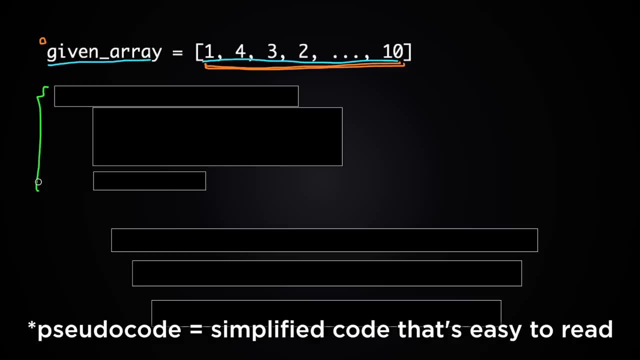 And I'm going to use pseudocode here to write this function. So first of all, let's define our function that's going to be called findSum, which is going to take given array as the input, And then inside this function, first of all, 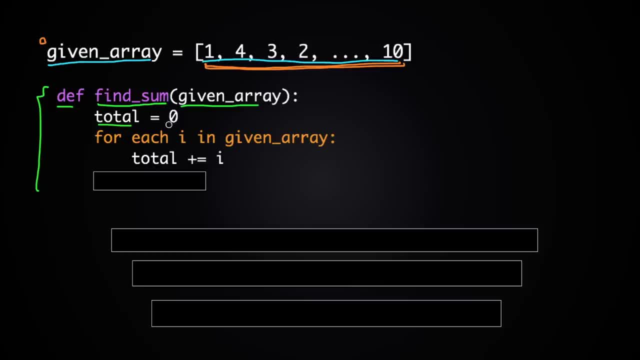 we're going to initialize a variable called total to zero And then, for each i in this given array, or for each number, each of these numbers in the given array, add that number i to total, And then at the end of this function we're just going to return total. 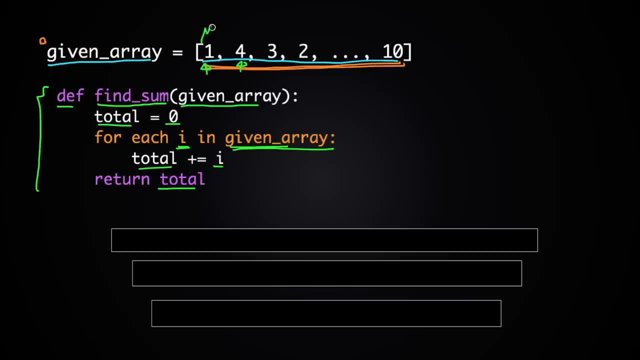 And that way we'll be able to find the sum of all the numbers in this array. Now, when you write this function, in whatever language you're using, whether it's Python, Java or anything else- you might ask yourself: well, how much time does it take to run this function? 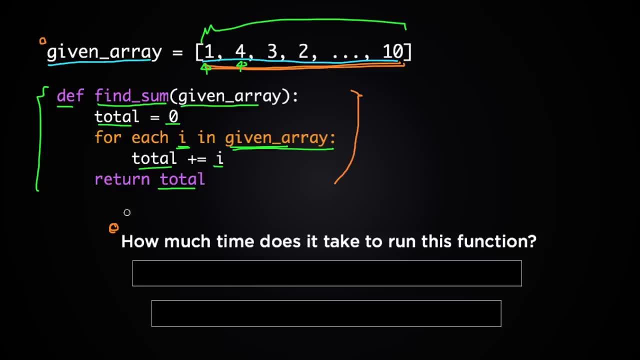 And that's actually a really hard question to answer because it depends on so many different factors, For example, how fast is your computer And when you run this function, are you running other programs at the same time, And also, which programming language are you using. 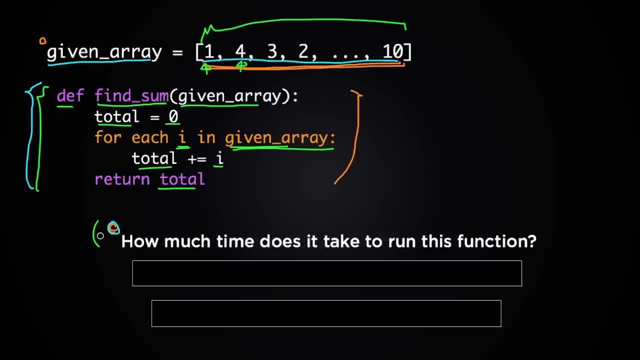 So, instead of asking this question directly, you might ask a related question instead, which is easier to answer actually, And that's: how does the runtime of this function grow as the size of the input grows? And this is a valid question to answer. 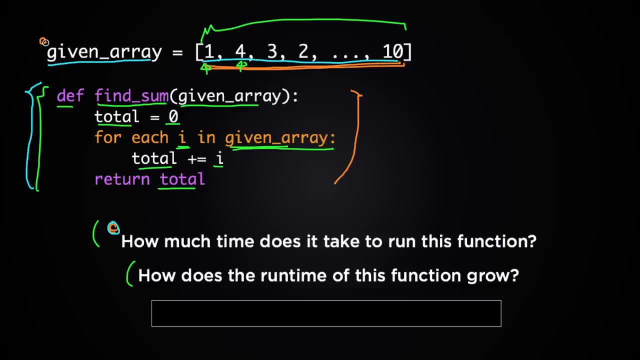 because, depending on the size of the input or depending on how many elements there are in the given array, it's going to take different amounts of time to execute this function, Because the more elements there are, the more time it takes to run this function. 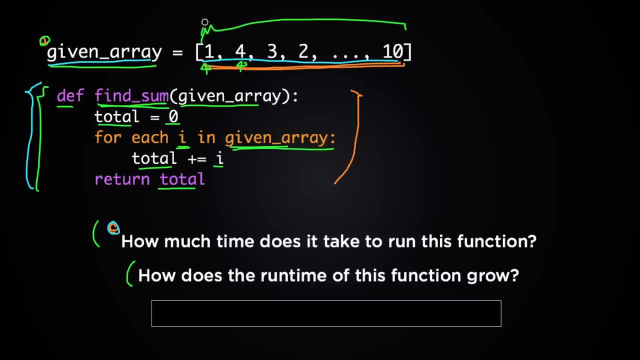 So the more elements there are in the given array, the more elements there are to add up and find the sum for. And to answer this second question you can use a pair of tools called Beagle Notation and Time Complexity. But before we get into that, I actually ended up running some experiments in Python to see how much time this function. 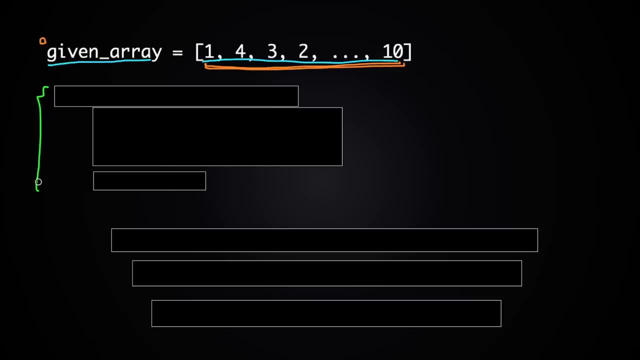 And that function might look like this function right here, and I'm going to use pseudocode here to write this function. So first of all, let's define our function that's going to be called findSum, which is going to take given array as the input, And then inside this function, first of all, 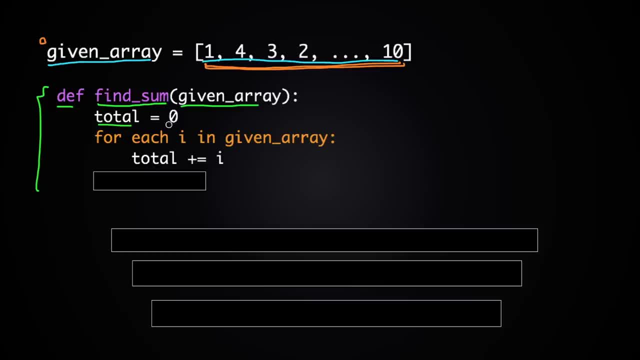 we're going to initialize a variable called total to 0, and then, for each i in this given array, or for each number, each of these numbers in the given array, add that number i to total, And then at the end of this function we're just going to return total. 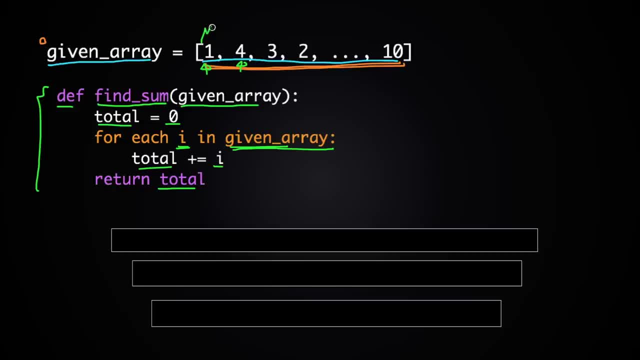 And that way we'll be able to find the sum of all the numbers in this array. Now, when you write this function, in whatever language you're using, whether it's Python, Java or anything else- you might ask yourself: well, how much time does it take to run this function? 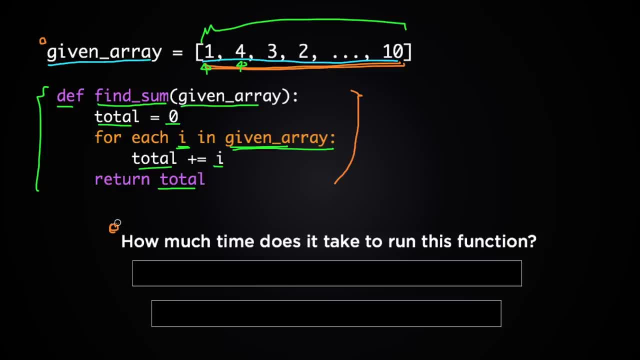 And that's actually a really hard question to answer because it depends on so many different factors, For example, how fast is your computer And when you run this function, are you running other programs at the same time, And also, which programming language are you using. 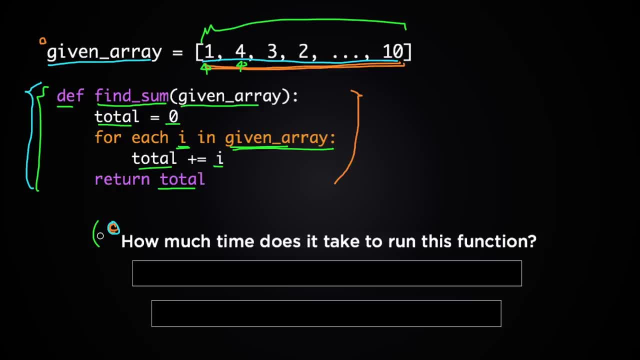 So, instead of asking this question directly, you might ask a related question instead, which is easier to answer actually, And that's: how does the runtime of this function grow as the size of the input grows? And this is a valid question to answer, because, depending on the size of the input, 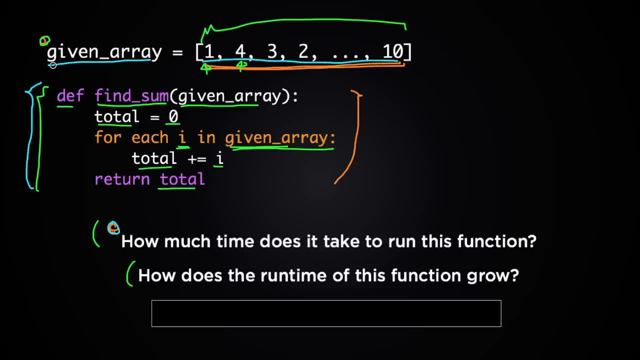 or depending on how many elements there are in the given array. it's going to take different amounts of time to execute this function because the more elements there are it will take more space to run. here are in the given array, the more elements there are to add up and find the sum for. 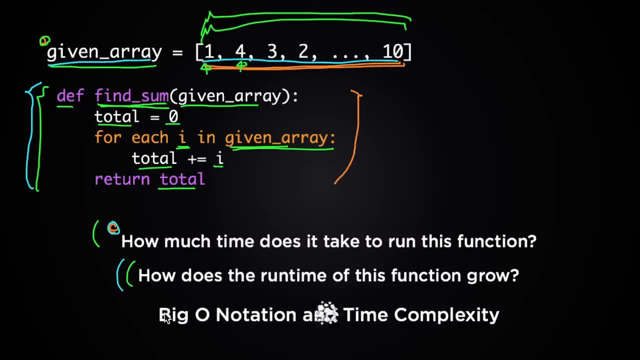 And to answer this second question, you can use a pair of tools called Beagle notation and time complexity. But before we get into that, I actually ended up running some experiments in Python to see how much time this function actually takes to complete for inputs of various sizes. 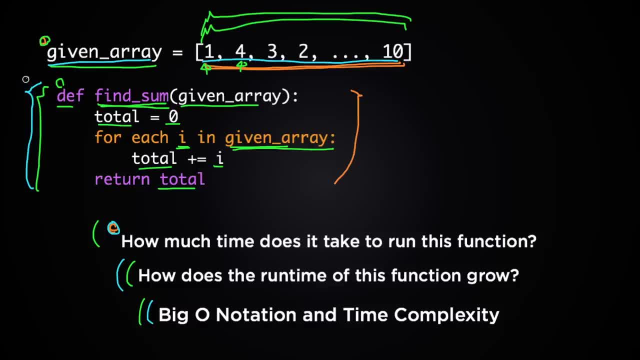 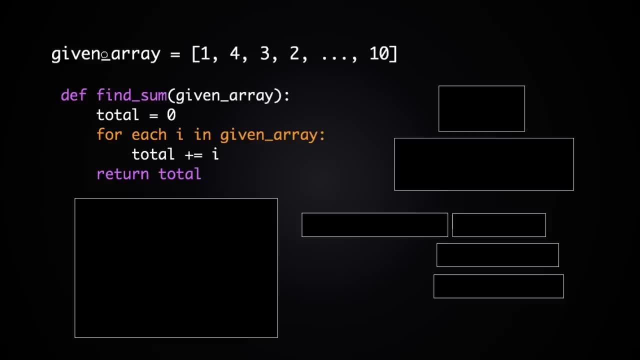 So let's take a look at the results of that first, because that's going to actually help us explain the concepts of Beagle, notation and time complexity. So here's what I did: I took this function and then implemented it in Python and then I generated a bunch. 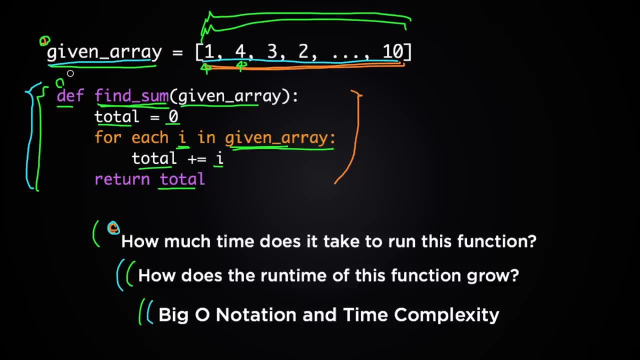 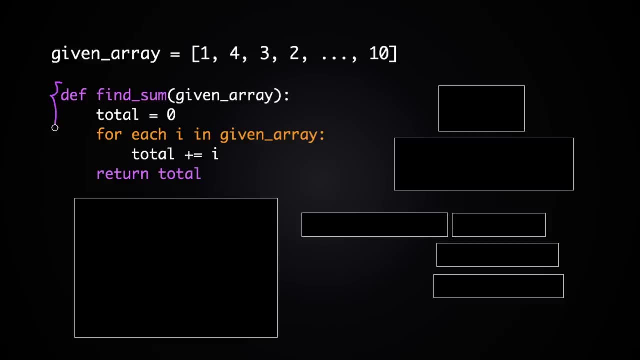 actually takes to complete for inputs of various sizes. So let's take a look at the results of that first, because that's going to actually help us explain the concepts of Beagle Notation and Time Complexity. So here's what I did: I took this function and then implemented it in Python. 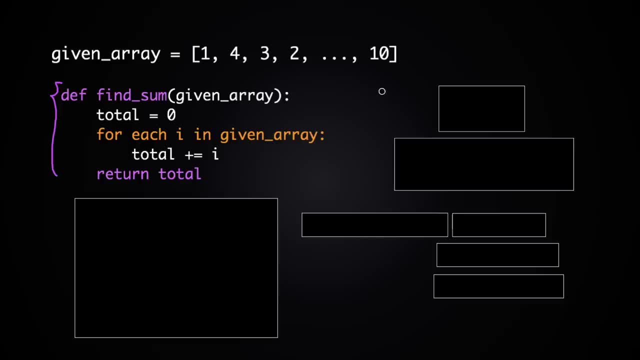 And then I generated a bunch of arrays with random elements with various sizes to use as input. So, for example, those arrays might look like these if the size is 5, or these if the number of elements in the array is 10.. And using these randomly generated arrays as input, 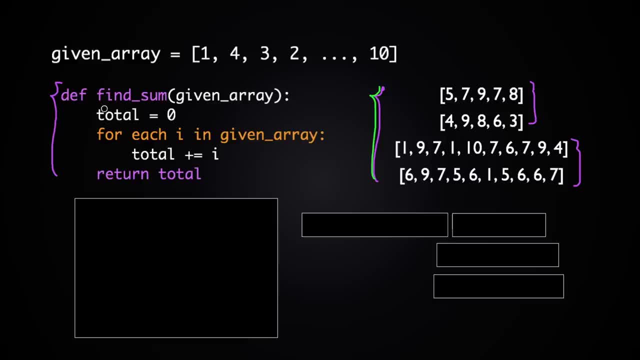 I ran this function findSum many, many times to find the average time it takes to run this function for each n, where n is the size of the given array or the number of elements in the given array. So if the given array is this one, n would be 5.. 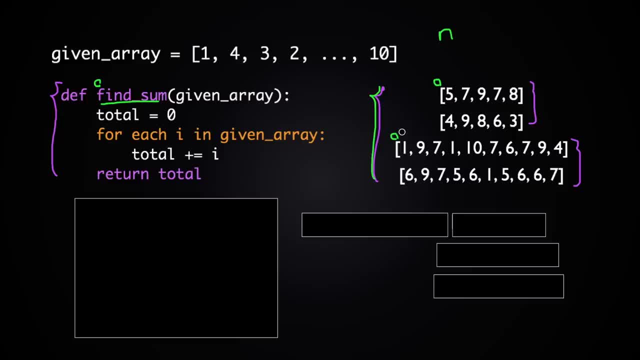 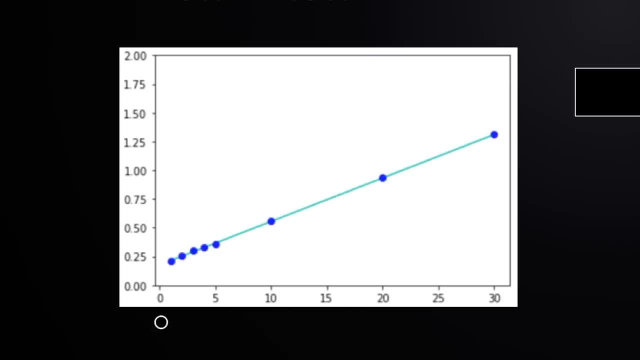 And if the given array is this one, n would be 10.. And here's the result I got. On the x-axis you see the size of the input or n, And on the bottom you see the size of the input. 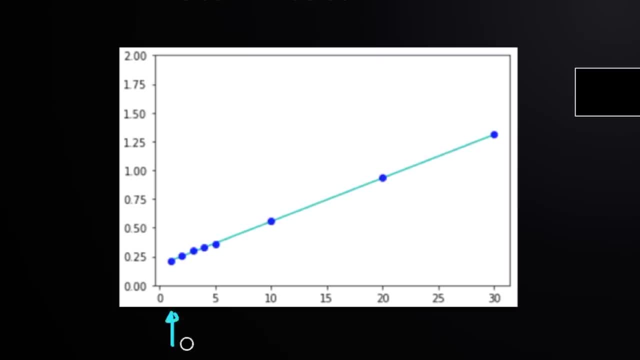 The size of the input ranges from one element, two elements and so on, up to 30 elements. And what you see on the y-axis is the time it takes. the time it took to run this function on average in microsecond. So, for example, with one element, 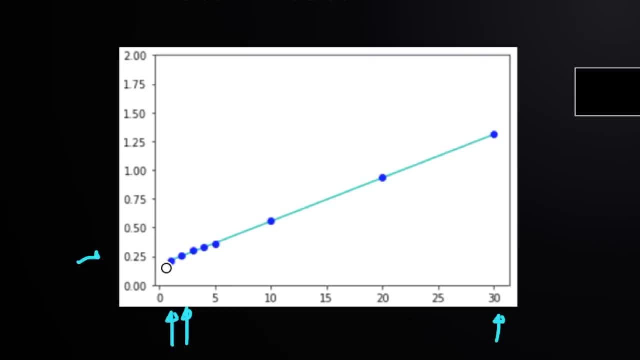 it took about 0.2 microseconds to run this function And then with 30 elements it takes about 1.25 microseconds on average And, as you can see, there's this straight line like pattern or a linear pattern here, or in other words, as the size or n increases. 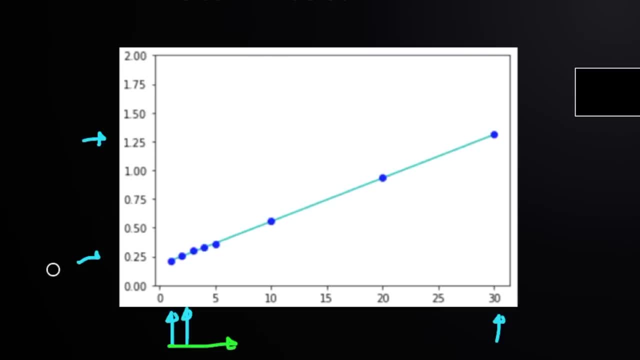 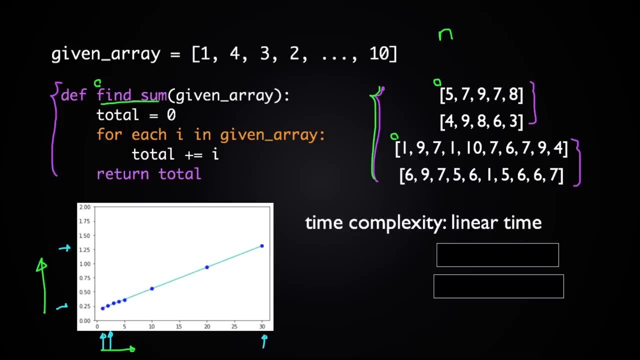 the amount of time it takes to complete this function increases linearly or like a straight line, And this pattern is called linear time complexity because, again, as the size of the input increases, the time increases linearly. So basically, time complexity is a way of showing 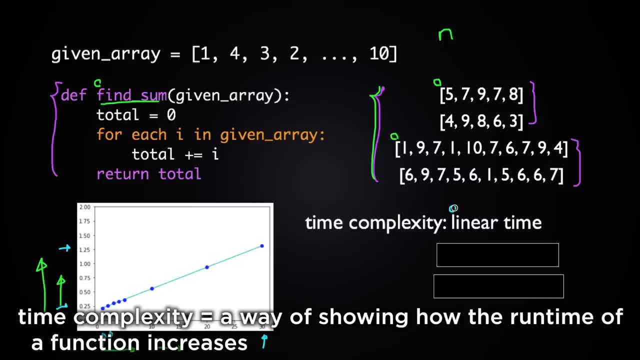 how the time it takes to complete a function or a particular piece of code increases as the size of the input increases. A linear time is just one type of time complexity and there are many different types, For example, constant time. This is when the time it takes to complete a function. 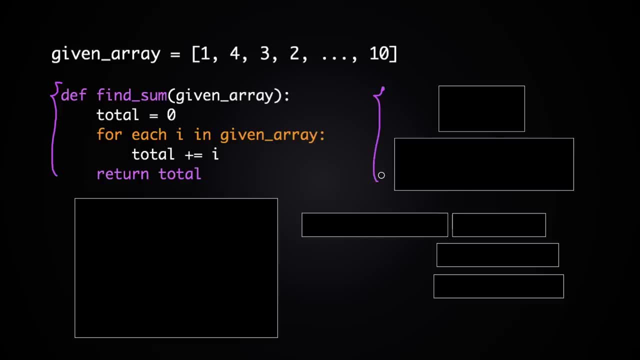 of arrays with random elements with various sizes to use as input. So, for example, those arrays might look like these if the size is five, or these if the number of elements in the array is 10.. And using these randomly generated arrays As input, I ran this function find some many, many times to find the average time it takes. 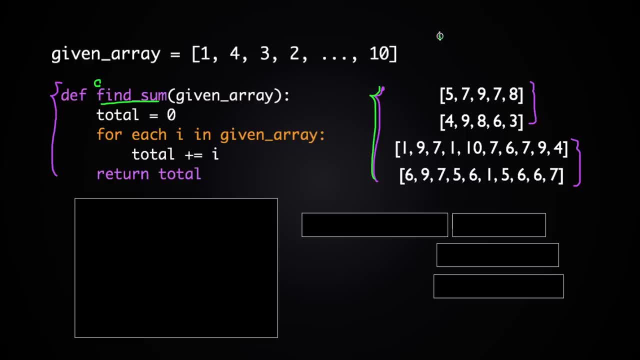 to run this function for each n, where n is the size of the given array or the number of elements in the given array. So if the given array is this one, n would be five, And if the given array is this one, n would be 10.. 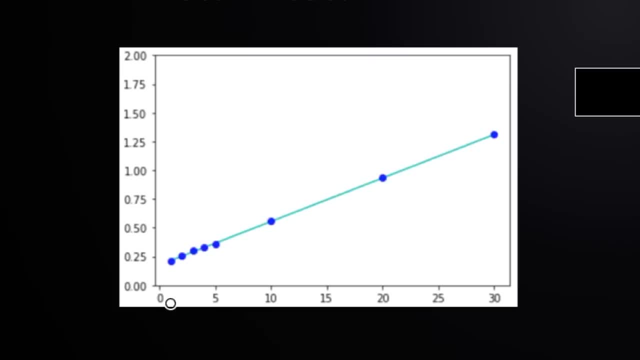 And here's the result I got. On the x axis you see the size of the input, or n, And the size of the input ranges from one element, two elements and so on, up to 30 elements. And what you see on the y axis is the time it takes, the time it took to run this function. 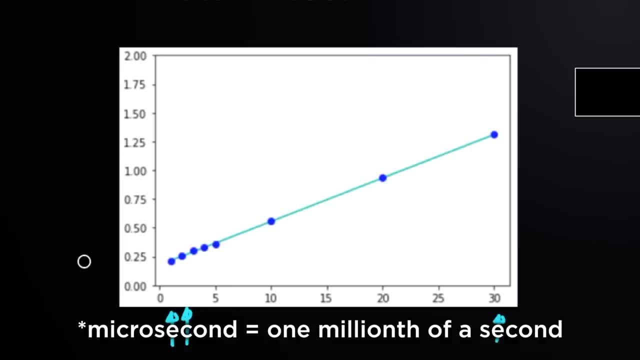 on average in microsecond. So, for example, with one element it took about 0.2 microseconds to run this function, And then with 30 elements it takes about 1.25 microseconds on average. And, as you can see, there's this straight line-like pattern or a linear pattern here. 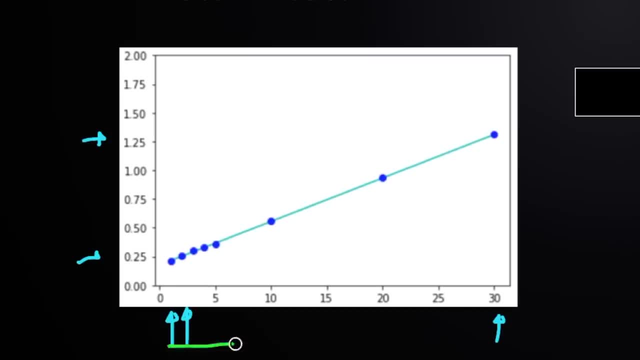 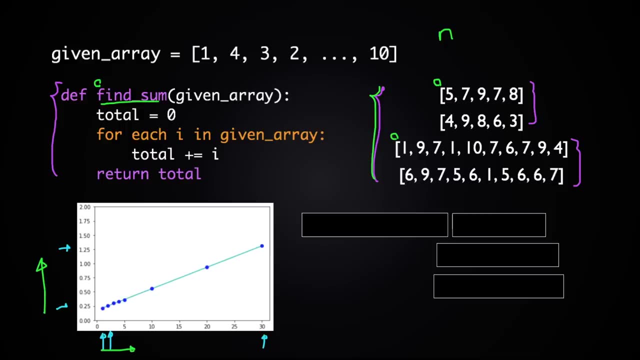 Or, in other words, as the size or n increases, the amount of time it takes to complete this function increases linearly or like a straight line. And this pattern is called linear time complexity Because, again, as the size of the input increases, the time increases linearly. 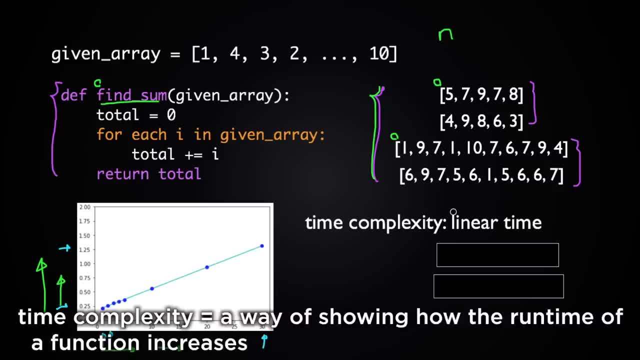 So basically, time complexity. Time complexity is a way of showing how the time it takes to complete a function or a particular piece of code increases as the size of the input increases, And linear time is just one type of time complexity and there are many different types. 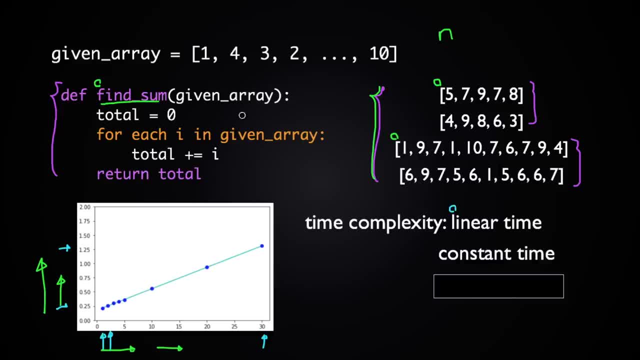 For example, constant time. This is when the time it takes to complete a function does not increase at all as the size of the input increases, or when the time stays at constant. So in that case, the graph- The graph might look like this: 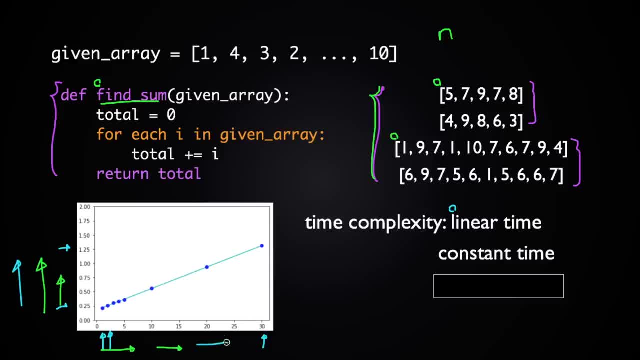 does not increase at all as the size of the input increases or when the time stays at constant. So in that case the graph might look like this: And there's also quadratic time complexity, And that's when the time it takes to complete a function. 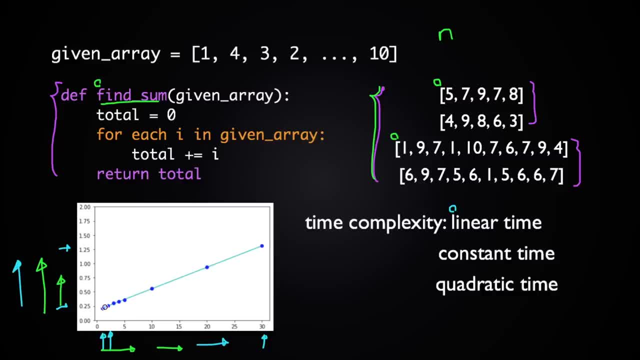 increases like a quadratic function, So that might look like this instead of the linear function that we saw earlier. Now, expressing different types of time complexity with words like linear, constant and quadratic is a little bit cumbersome, partly because you need to remember to use these different words. 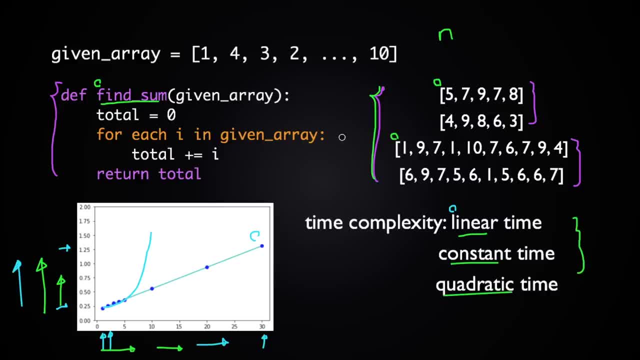 So you might say, is there any way to express different types of time complexity in a more mathematical, you know, systematic way? There is, and that's what Big O notation is. So, for example, linear time can be expressed as Big O of n. 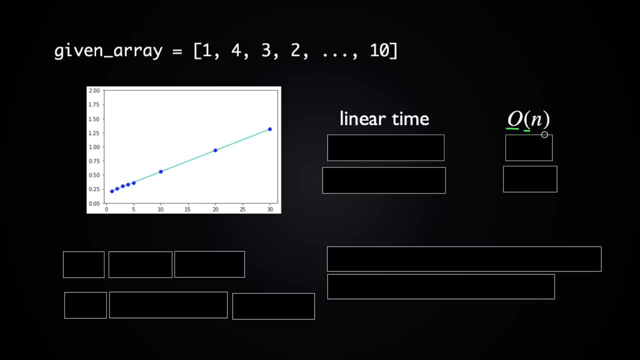 That's capital O, followed by parentheses with n inside, And n is usually the size of the input, And in this case this is an o. So in this case, this is a squared number. So in this case, this is a squared number. 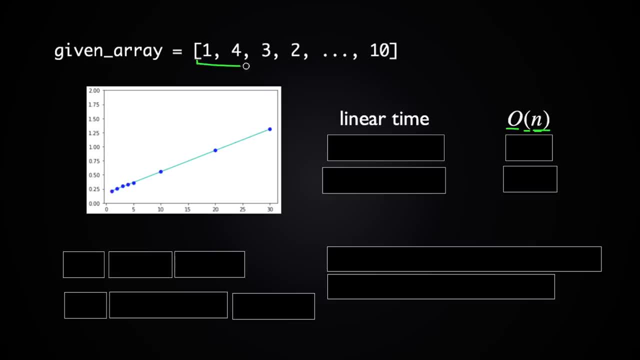 So in this case this is an o. So in this case this is a squared number. particular case: it's the number of elements in the given array, and this whole expression is usually read as either big O of n or simply O of n, and constant time can be expressed as big O of 1. 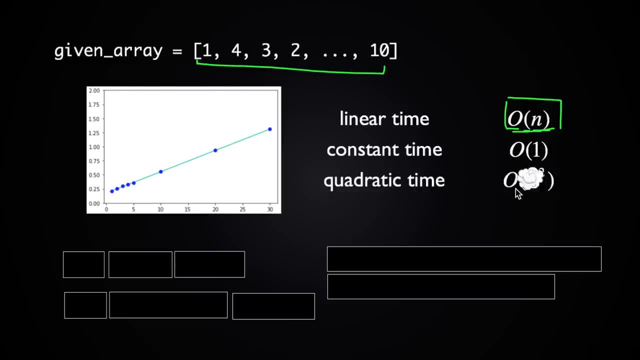 and quadratic time can be expressed as big O of n squared. So, as you can see, just by changing what's inside the big O expression you're able to express different types of time complexity. but how do we know that linear time should be big O of n and constant time is big O of 1, and so on? 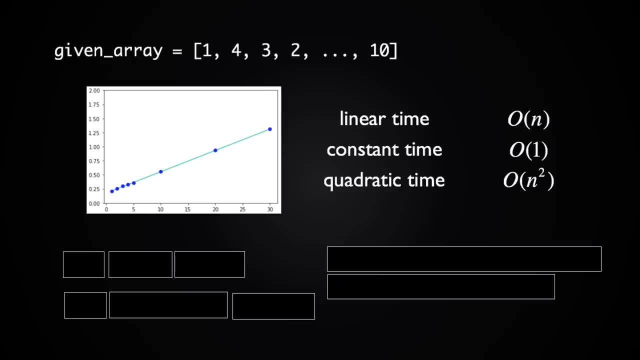 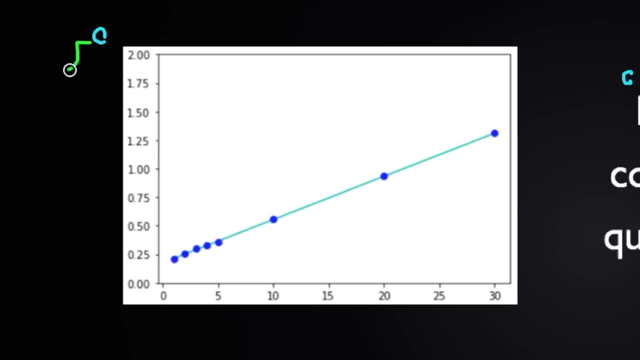 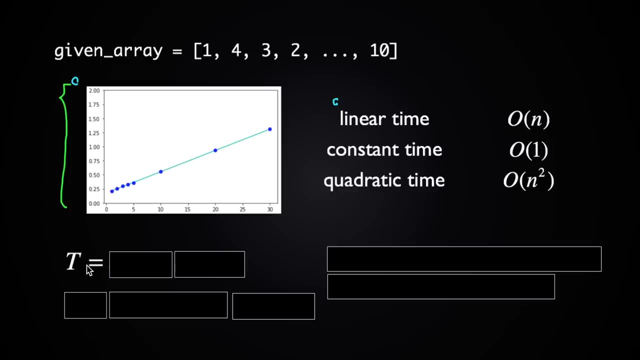 Well, to understand, let's take a look at the example we saw just earlier, where we had linear time or this graph right here Now. just by looking at this graph you can probably tell that the time it takes to run this function, or t, can be expressed as a linear function. so that should be in the form of. 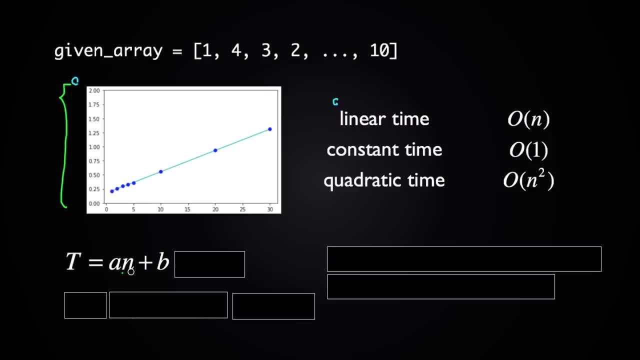 t equals n plus 1.. So we're given n plus b, where n is the size of the input, or the number of elements in the array, and a and b are two constants. and how do we know that this expression is big O of n? Well to find. 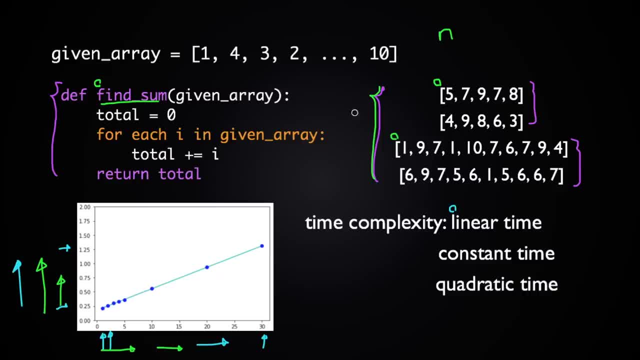 And there's also quadratic time complexity, And that's when the time it takes to complete a function increases like a quadratic function. So that might look like this instead of the linear function that we saw earlier, Now expressing different types of time complexity with words like linear, constant and quadratic. 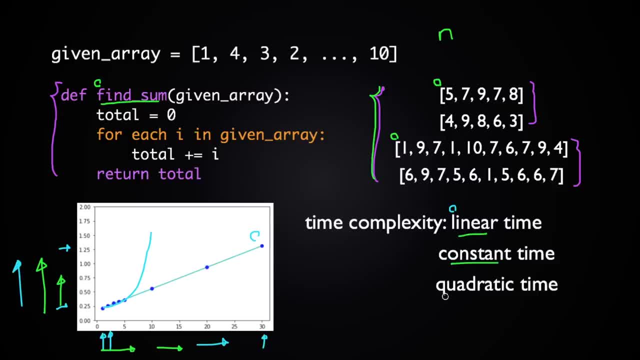 is a little bit cumbersome, partly because you need to remember to use these different words. So you might say: is there any way to express different types of time complexity in a more mathematical, you know, systematic way? There is, and that's what big O notation is. 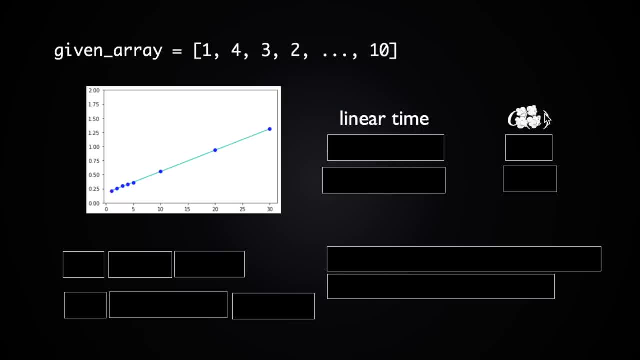 So, for example, linear time can be expressed as big O of n, That's capital O, followed by parentheses with n inside, And n is usually the size of the input and in this particular case, it's the number of elements in the given array. 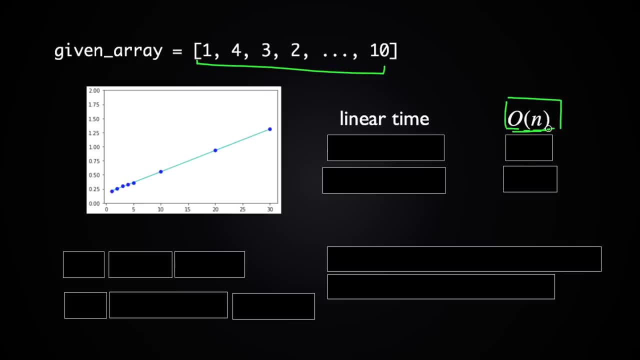 And this whole expression is usually read as either big O of n or simply O of n, And constant time can be expressed as big O of 1. And quadratic time can be expressed as big O of n squared. So, as you can see, just by changing what's inside the big O expression you're able to. 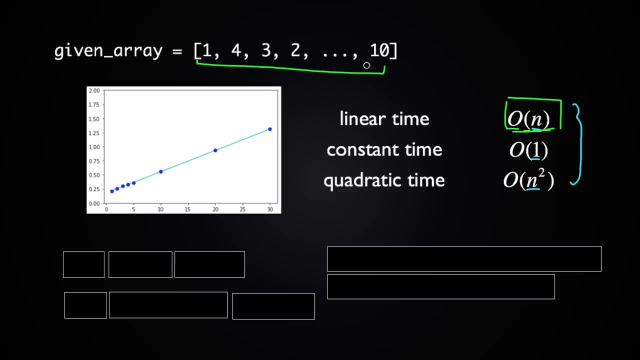 express different types of time complexity. But how do we know that linear time should be big O of n And constant time is n? Well, to understand, let's take a look at the example we saw just earlier where we had linear time, or this graph right here: 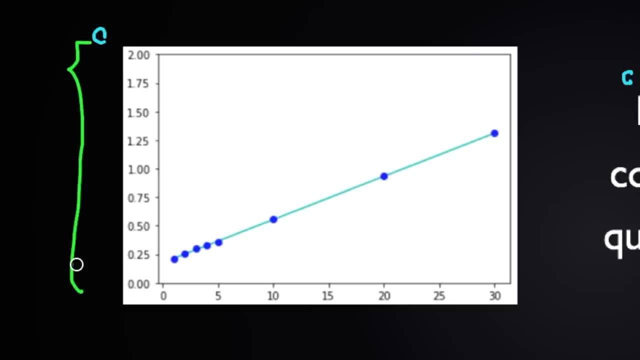 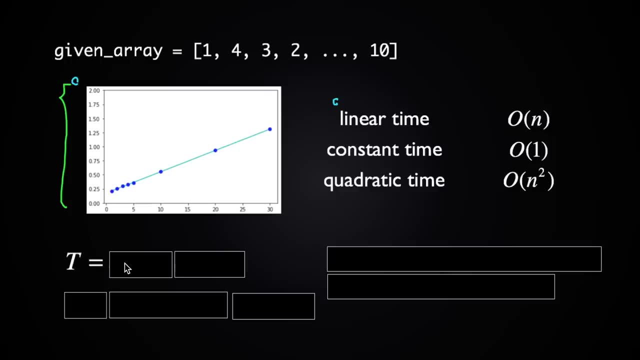 Now, just by looking at this graph you can probably tell that the time it takes to run this function, or t, can be expressed as a linear function, So that should be in the form of: t equals n plus b, where n is the size of the input. 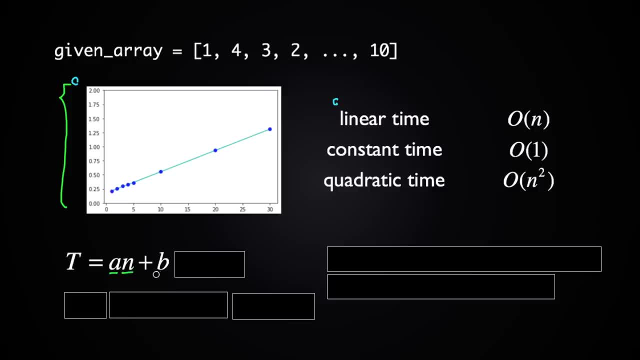 or the number of elements in the array, And a and b are two constants. And how do we know that this expression is big O of n? Well, to find that out, there's a simple trick for doing that, And there are two steps you need to follow. 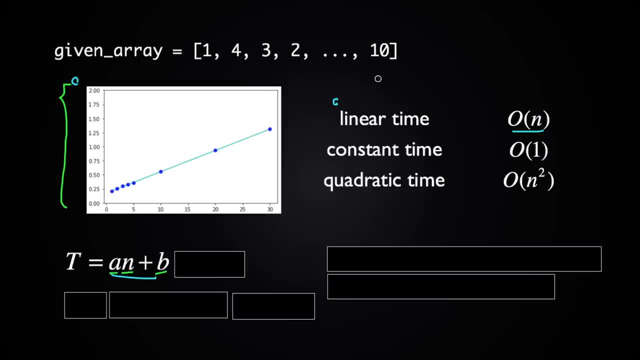 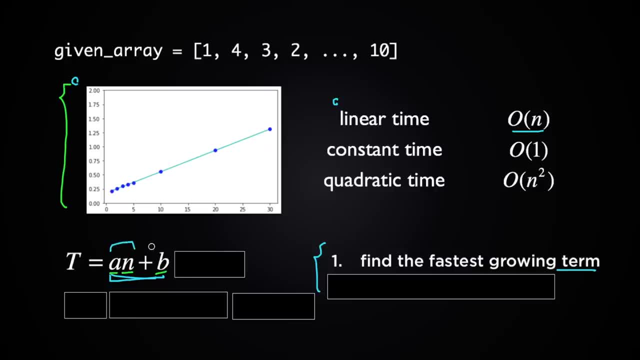 so you need to ask yourself which one is the fastest growing term. Well, b does not grow at all as n increases. so the fastest growing term here is an. And then the second step is to take out the coefficient out of that fastest growing term. So the coefficient here is a, because a is a constant. 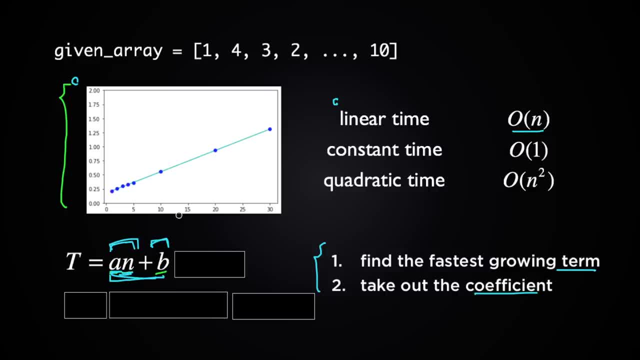 and n is not a constant. So if you take out the coefficient out of that fastest growing term, you're take out the coefficient out of this term an, you're left with just n and that's what should go inside the big o expression. okay, and a quick note here. this is actually not the most mathematically. 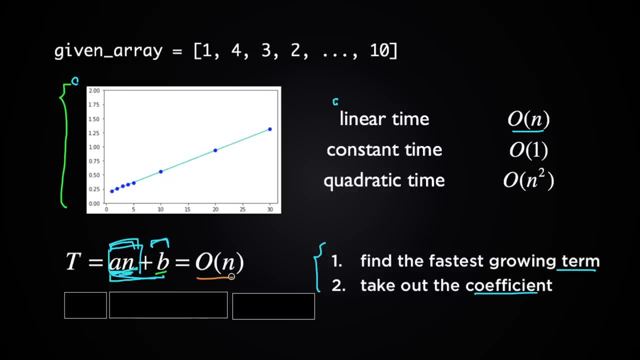 rigorous way of finding the big o expression, but it's actually good enough for all practical purposes. but if you want me to make a separate video about the formal mathematical definition of big o, let me know in a comment. anyway, let's take a look at another example here. what if the 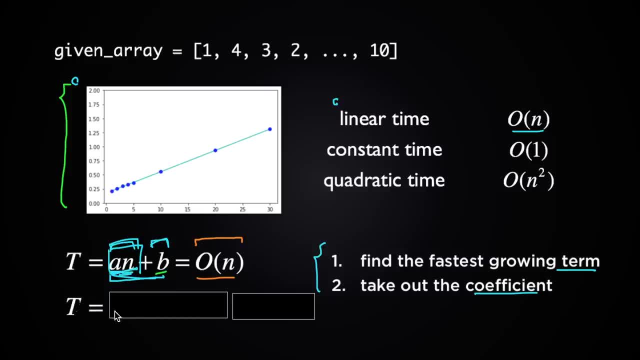 time it takes to run your function or t turns out to have this form: cn squared plus dn plus e, where c, d and e are constants, then you can follow the exactly the same steps. first of all, find the fastest growing term. there are three terms here: cn, squared, dn and e- and immediately you can tell. 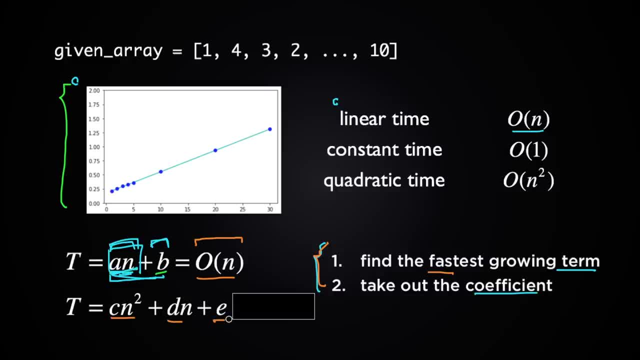 that you have a big o expression and you're left with just n, and that's what should go inside the. that e is not the fastest growing term because it's just a constant. so you need to compare cn squared and dn and find which one is the faster, faster growing term. one way to do that is by 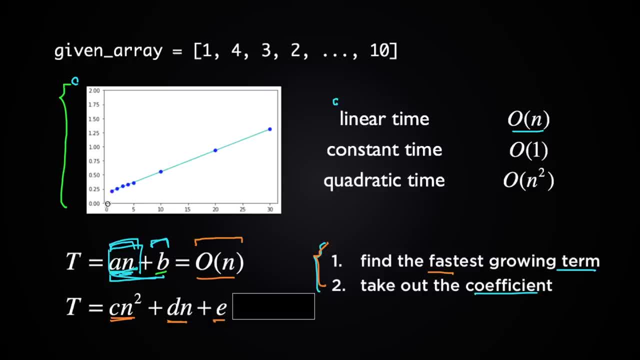 drawing them on a graph. so dn will look like this, or maybe this, depending on the value of d. it's just a straight line, and cn, squared, will look like this, or maybe this or maybe this, depending on the value of c. and as you examine these two expressions this way, you'll. 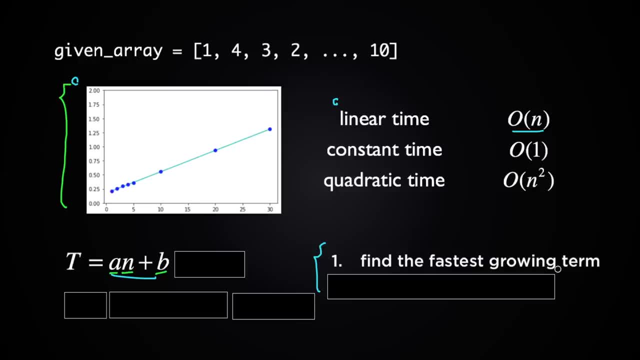 The first step is to find the fastest growing term in the given function. So we're given n plus b, And here we have two terms, a, n and b. So you need to ask yourself which one is the fastest growing term. Well, b does not grow at all as n increases. 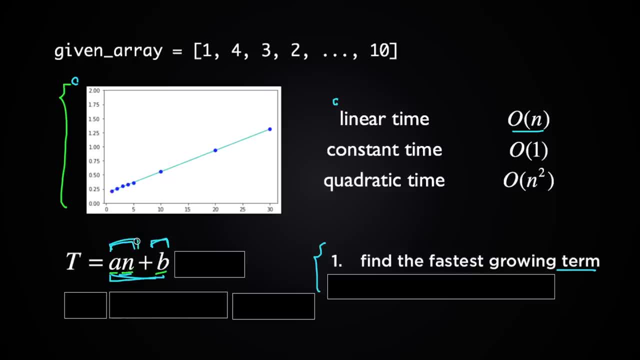 So the fastest growing term here is a- n. And then the second step is to take out the coefficient out of the fastest growing term. So the coefficient here is a, because a is a constant and n is not a constant. So if you take out the coefficient out of this term- a- n- you're left with the number. 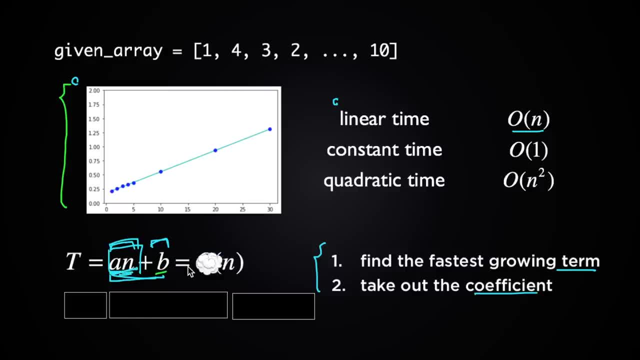 just n, and that's what should go inside the big o expression. okay, and a quick note here: this is actually not the most mathematically rigorous way of finding the big o expression, but it's actually good enough for all practical purposes. but if you want me to make a separate 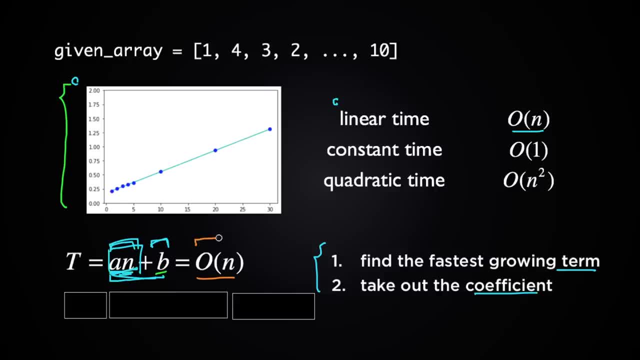 video about the formal mathematical definition of big o. let me know in a comment. anyway, let's take a look at another example here. what if the time it takes to run your function or t, turns out to have this form: c- n squared plus d, n plus e, where c, d and e are constants? then 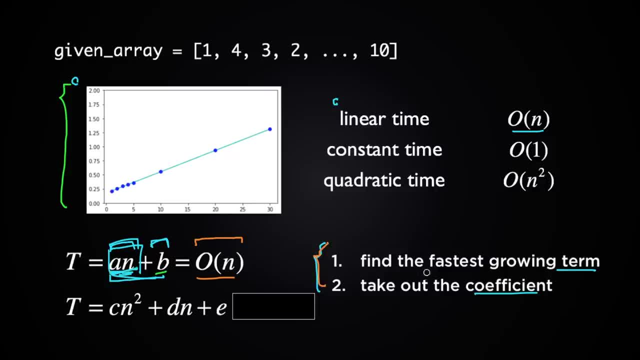 you can follow the exactly the same steps. first of all, find the fastest growing term. there are three terms here: cn, squared dn and e. and immediately you can tell that e is not the fastest growing term because it's just a constant, so you need to compare c. 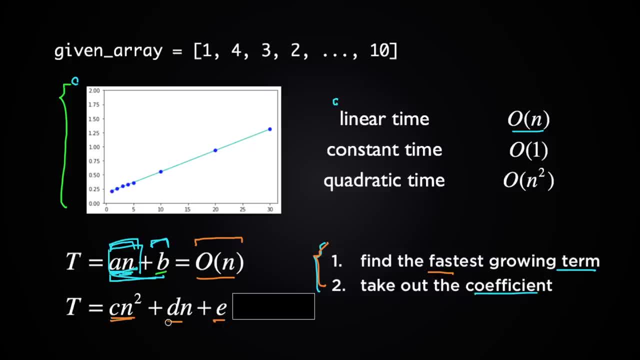 squared and dn and find which one is the fastest. as you'll probably notice that now is the fastest growing term in the citing integral of n: squared. squared is initially a faster growing term. One way to do that is by drawing them on a graph, So dn will look like: 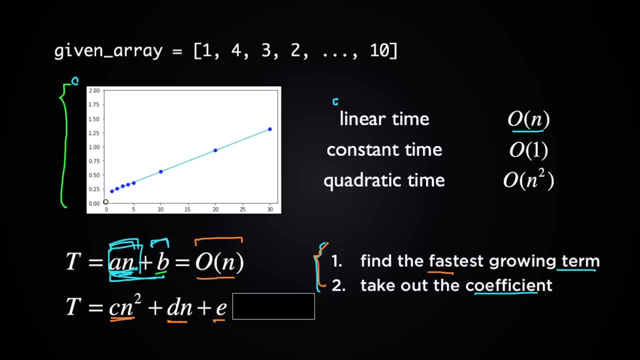 this or maybe this, depending on the value of d. It's just a straight line and cn, squared, will look like this, or maybe this, or maybe this, depending on the value of c. And as you're examining these two expressions this way, you'll notice that, no matter what the values of c and d are, eventually 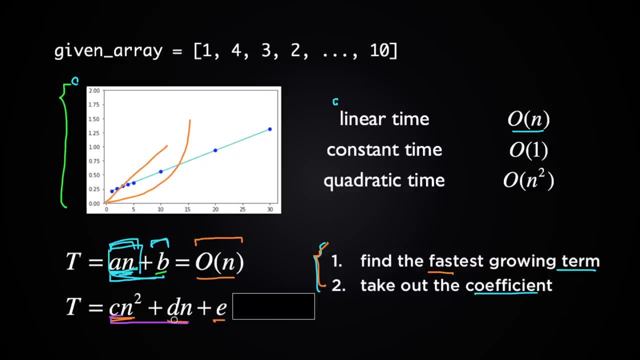 notice that, no matter what the values of c and d are, eventually, as n gets larger and larger, cn squared will be much bigger than dn and it'll keep getting bigger and bigger. and that's how we know that the first term, cn squared, is the fastest growing term here. so basically we're looking for 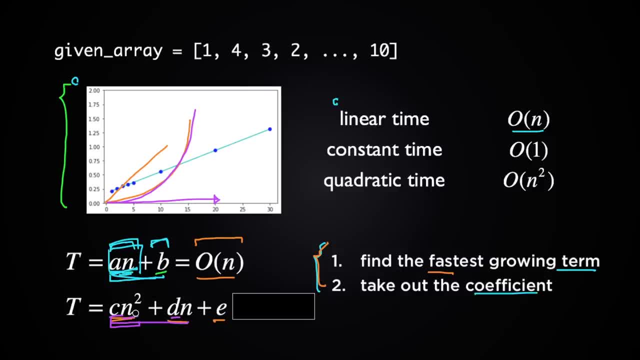 the fastest growing term when n is very, very large. so here, as long as c and d are both constants and positive, we'll know that cn squared is the fastest growing term when n is very large. so you can take cn squared as the fastest growing term out of step one and then go to step two, take out the. 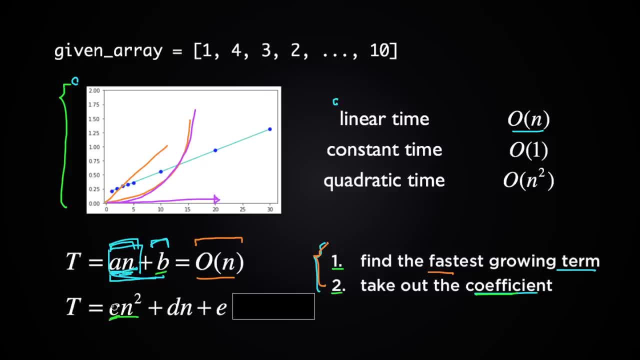 coefficient. the coefficient here is c, so take that out and what's left here is just n squared and that's what's gonna be inside the big O expression. So we have T is big O of N squared, and that's why we have here quadratic time. 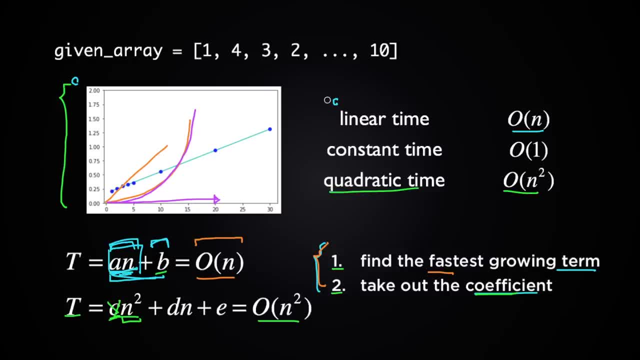 Okay. so one thing that's convenient about time, complexity and big O notation is that they give you a rough idea about how your function scales as the input to that function gets larger and larger, And in computer science you tend to care more about the larger input. 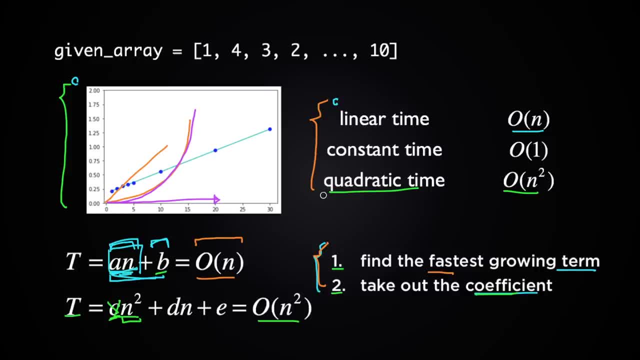 than smaller input, because when the input is small enough, your function is probably not gonna take that much time. And another convenient feature of time, complexity and big O notation is that it doesn't depend on your particular environment. So, for example, I ran this experiment on my new MacBook Pro. 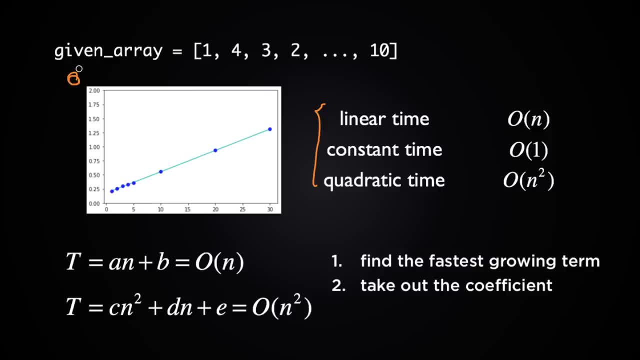 which is pretty fast, and this is the result I got. And actually I ended up running the same experiment on my older computer and the result looked like this instead. So, as you can see, for the same size of the input, 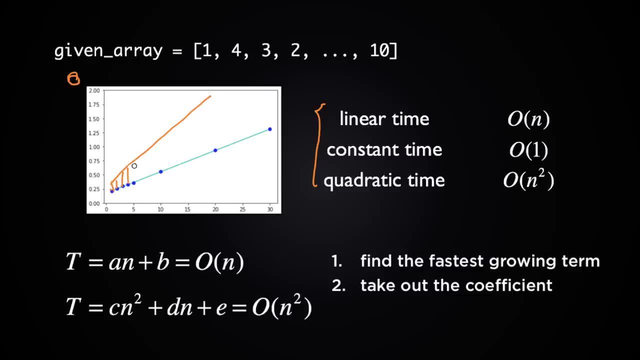 it took much more time on my older computer than my newer computer, which makes sense. But if you look at this new line, it's still a linear function, So it still has the form. T equals N plus B, although A and B the two constants. 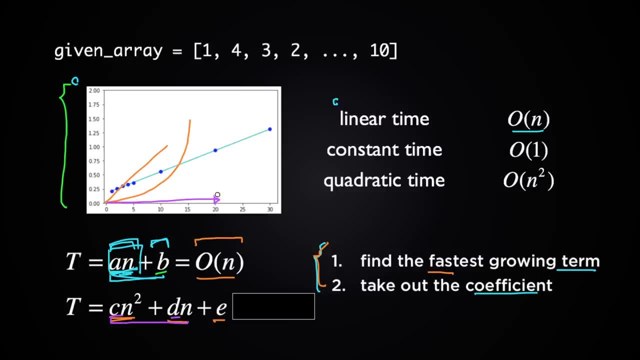 as n gets larger and larger, cn squared will be much bigger than dn and it'll keep getting bigger and bigger. And that's how we know that the first term, cn squared, is the fastest growing term here. So basically we're looking for the fastest growing term when n is very, very large. So here, as long 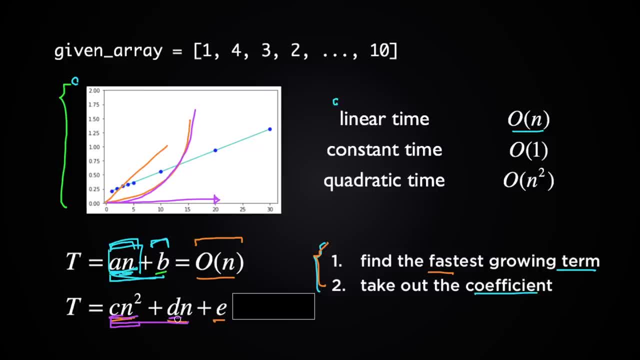 as c is the fastest growing term. we're looking for the fastest growing term when n is very, very and d are both constants and positive. we'll know that cn squared is the fastest growing term when n is very large. so you can take cn squared as the fastest growing term out of step one and then go. 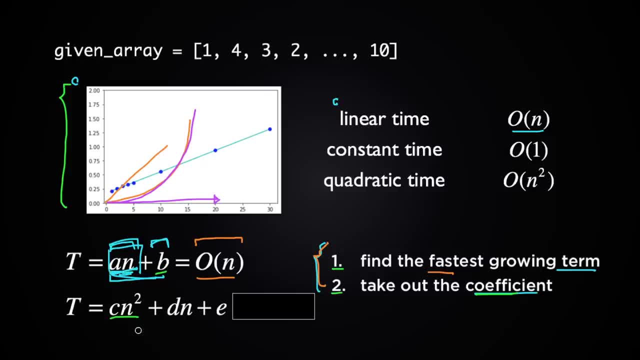 to step two: take out the coefficient. the coefficient here is c, so take that out and what's left here is just n? squared, and that's what's going to be inside the big o expression. so we have t is big o of n squared, and that's why we have here quadratic time, okay, so one thing that's. 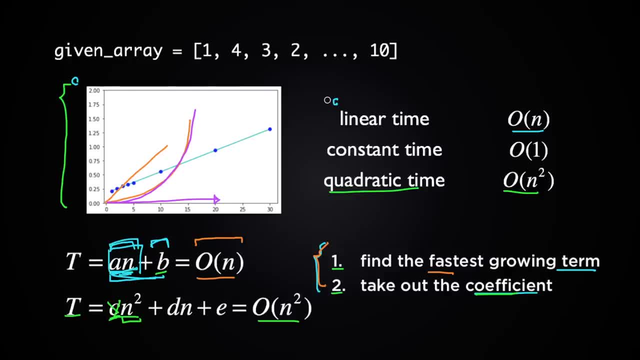 convenient about time. complexity and big o notation is that they give you a rough idea about how your function scales as the input to that function gets larger and larger. and in computer science you tend to care more about the larger input than smaller input. because when the input 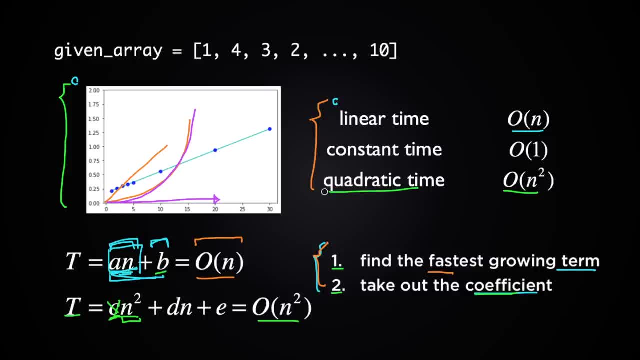 is small enough, your function is probably not going to take that much time, and another convenient feature of time, complexity and bigger notation is that it doesn't depend on your particular environment. so, for example, i ran this experiment on my new macbook pro, which is pretty fast, and this is the result i got, and actually i ended up running the same. 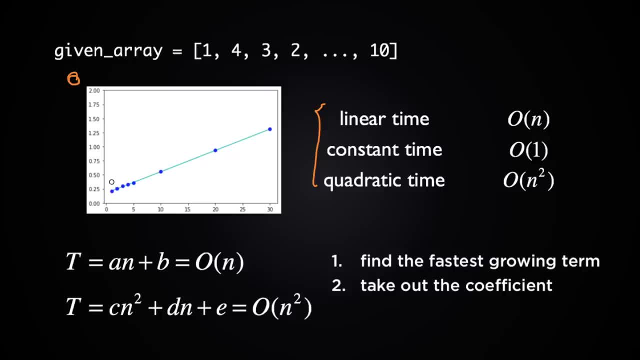 experiment on my older computer and the result looked like this instead. so, as you can see, for the same size of the input, it took me about 10 minutes to do this experiment and i ended up doing much more time on my older computer than my newer computer, which makes sense. but if you look at this, 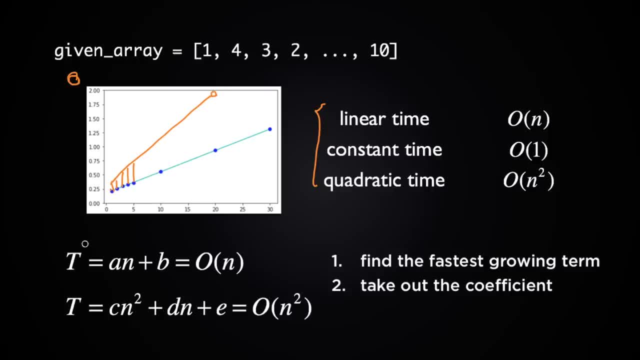 new line. it's still a linear function, so it still has the form: t equals n plus b, although a and b- the two constants- will be probably larger than my newer computer. but if you go through the same steps that we went through earlier- finding the fastest growing term and taking out the 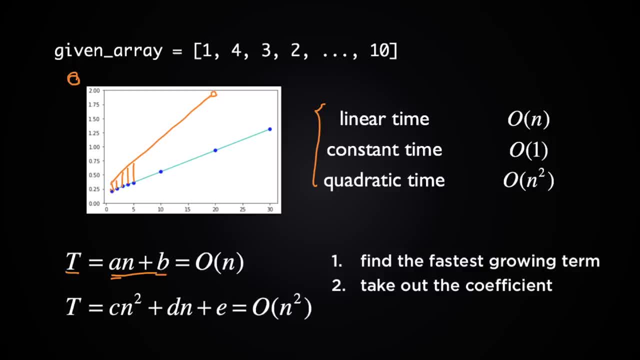 will be probably larger than my newer computer. But if you go through the same steps that we went through earlier- finding the fastest and taking out the coefficient of that term, this term, right here- you'll find that this is still big O of N. 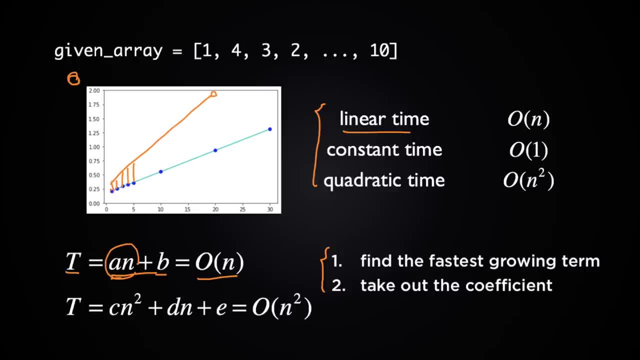 and this is still linear time. So, in general, no matter how fast or slow your computer is and pretty much no matter what programming language you use, as long as you use the same algorithm or the same steps for solving the problem, you'll still get the same time complexity. 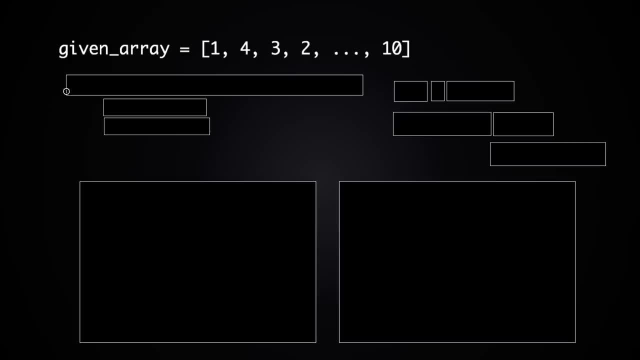 and the same big O. Okay for more practice. let's take a look at another example. Okay, for more practice. let's take a look at another example. Okay, for more practice, let's take a look at another example. 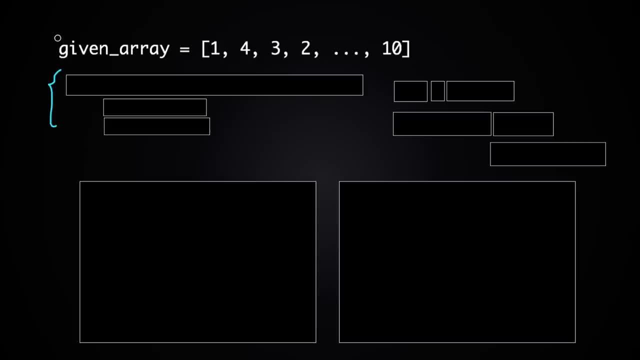 Here, just like the previous example, we're given an array of numbers, and this could be any size, And here we have a function called stupid function, which takes the given array. and this function is stupid because this is all it does. 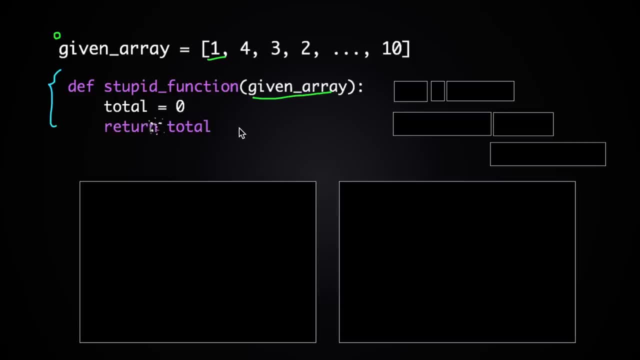 It initializes a new variable called total and then it returns it. So it doesn't really do anything with the given input, And I ran the same experiment as the previous example using this function. I took this function, implemented it in Python. 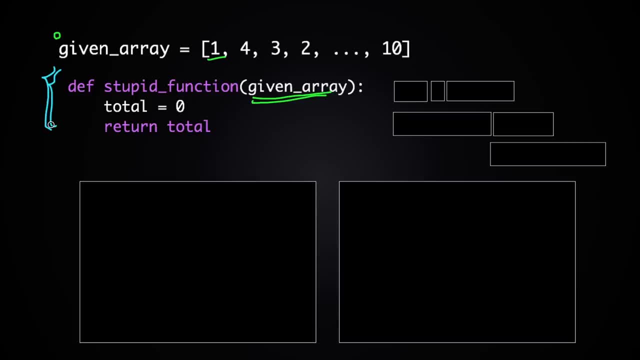 and then run this function for arrays of various sizes and found the average time it took to execute this function for each of those inputs. And here's the result I got. And just like before, we have n or the number of items. 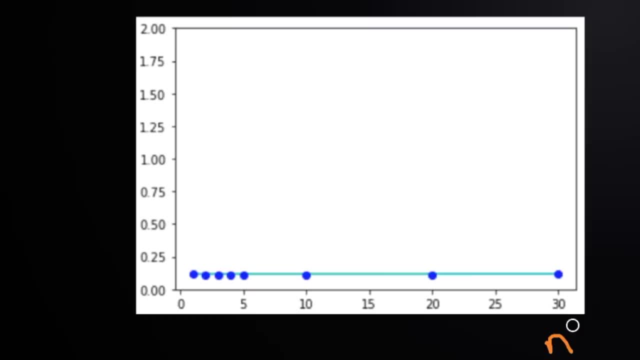 the number of elements in the given array on the x-axis and on the y-axis we have t, or the average time it took to run this function, And, as you can see, the time it took to run this function doesn't increase at all. 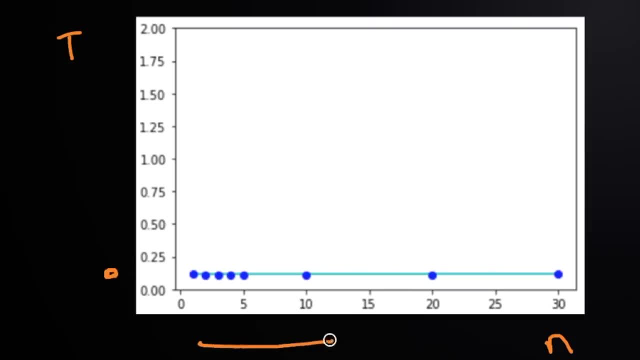 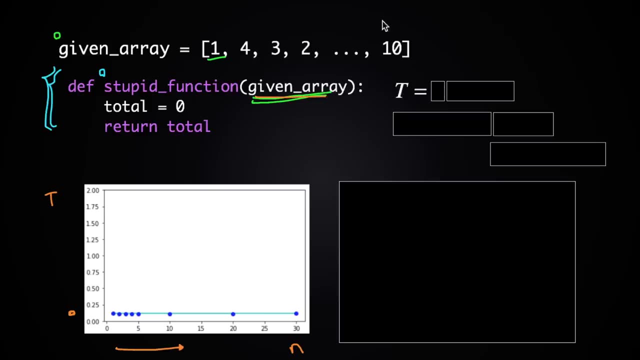 as the number of elements in the array increases, which makes sense because this function doesn't do anything with the given array. Okay, so you can express t here, the time it takes to run this function as a constant. Let's call that constant c for now. 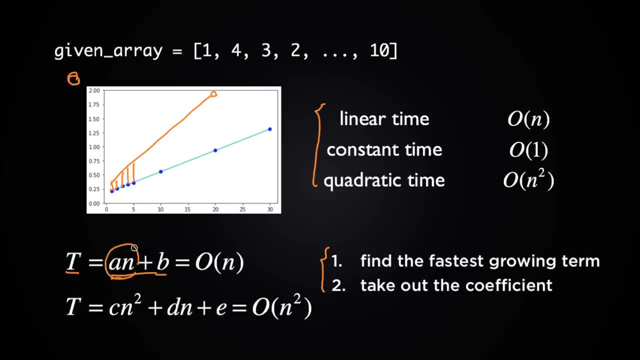 coefficient of that term, this term. right here you'll find that this is still a linear function and this is still linear time. so, in general, no matter how fast or slow your computer is and pretty much no matter what programming language you use, as long as you use the same algorithm or 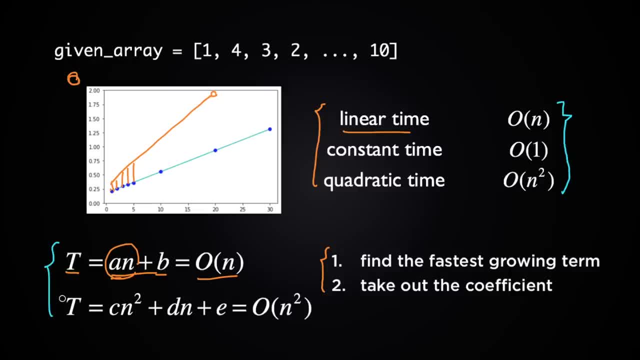 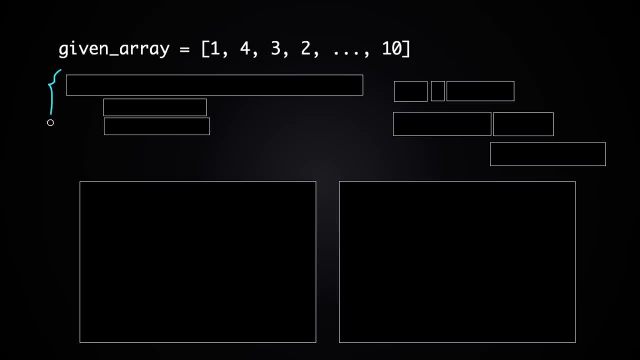 the same steps for solving the problem, you'll still get the same time, complexity and the same big o. okay, for more practice, let's take a look at another example here. here, just like the previous example, we're given an array of numbers, and this could be any size, and here we have a function called stupid function, which takes 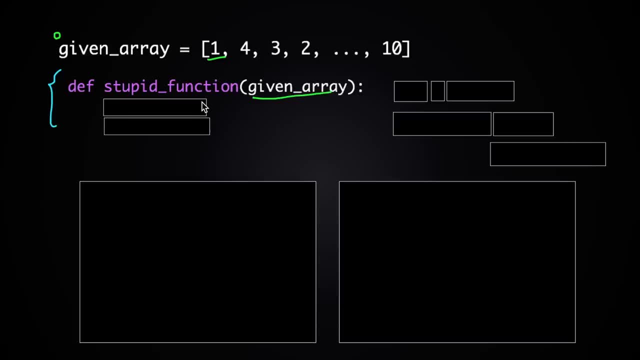 the given array. and this function is stupid because this is all it does: it initializes a new variable called total and then it returns it, so it doesn't really do anything with the given input, and i ran the same experiment as the previous example using this function. i took this function implemented in python and then ran this function for. 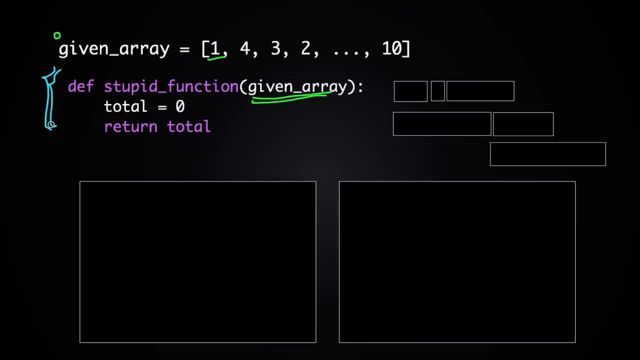 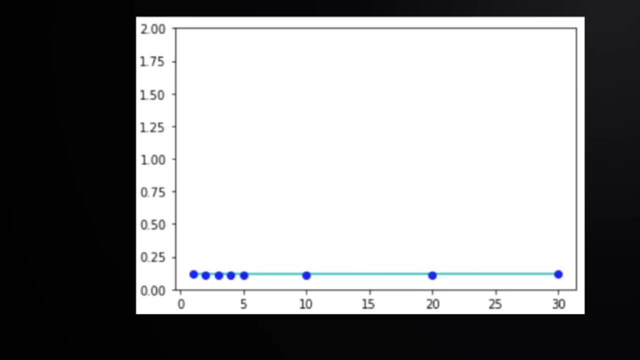 arrays of various sizes and found the average time it took to execute this function for each of those inputs. And here's the result I got. And, just like before, we have n, or the number of items, the number of elements in the given array, on the x-axis And on the y-axis we have t. 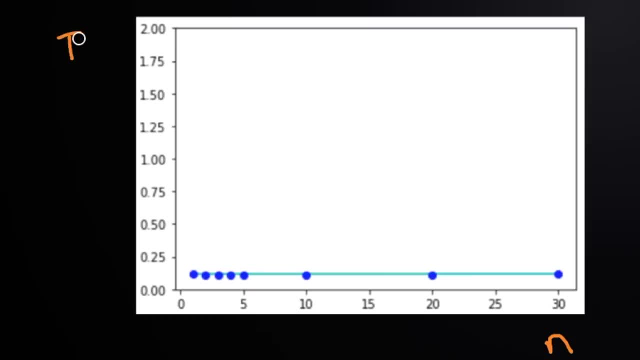 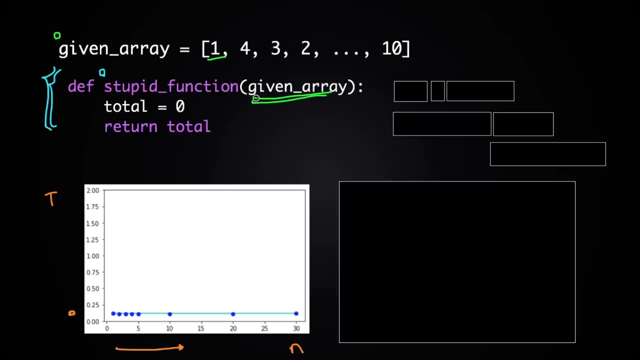 or the average time it took to run this function for each n. And, as you can see, the time it took to run this function doesn't increase at all as the number of elements in the array increases, which makes sense because this function doesn't do anything with the given array. Okay, so you can. 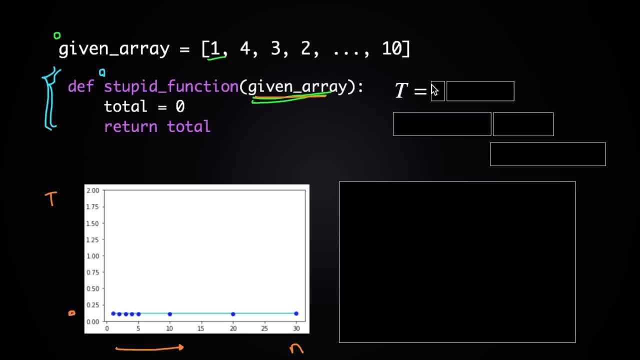 express t here, the time it takes to run this function as a constant. Let's call that constant c for now, And in this particular case c here is about 0.115 microseconds. And here you might say: how can we? 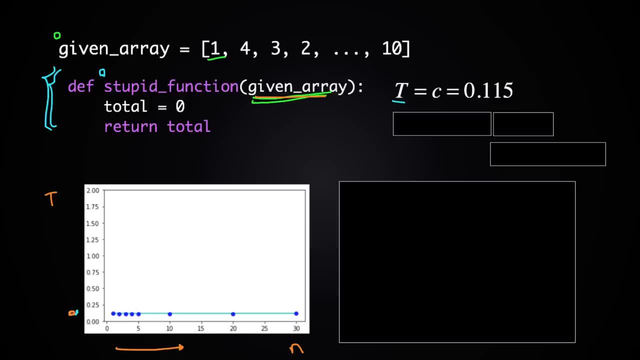 express this with big O- To find that you can basically follow the same two steps that we saw earlier. So, first of all, find the fastest growing term out of this expression. We only have one term here, 0.115, so that's automatically the fastest growing term here. And the second step is to take. 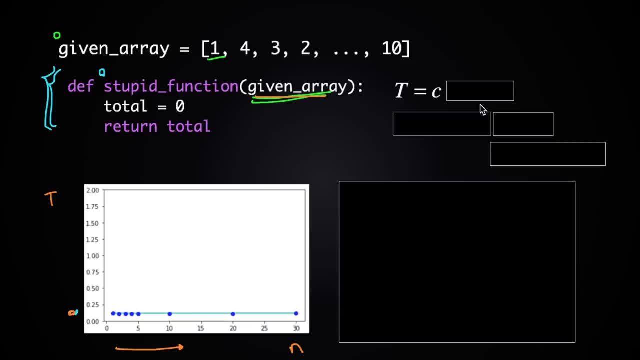 And in this particular case, c, here is about 0.11.. 0.115 microseconds. And here you might say: how can we express this with big O? To find that you can basically follow the same two steps that we saw earlier. 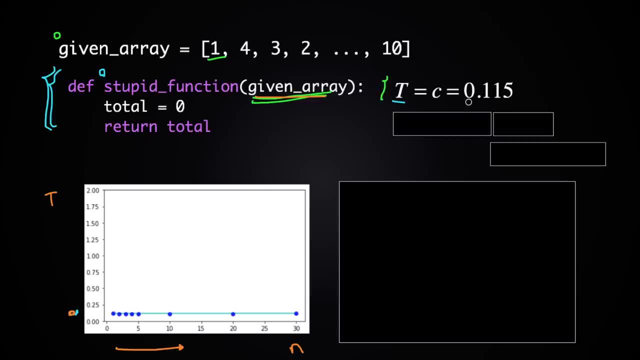 So first of all, find the fastest growing term out of this expression. We only have one term here, 0.115, so that's automatically the fastest growing term here. And the second step is to take out the coefficient. But this whole thing is a coefficient. 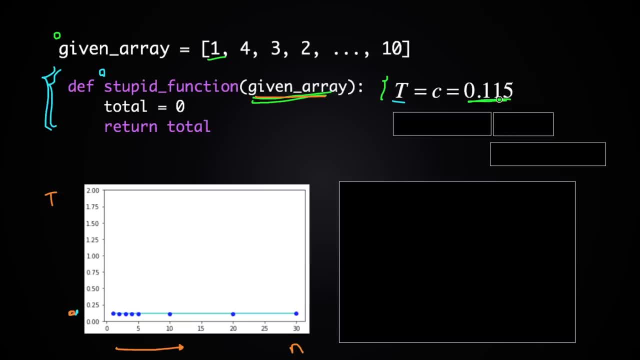 so how should we think about it? One way to think about it is that 0.115 can be rewritten as 0.115 times one, So when you take out 0.115 out of this expression, you're left with one. 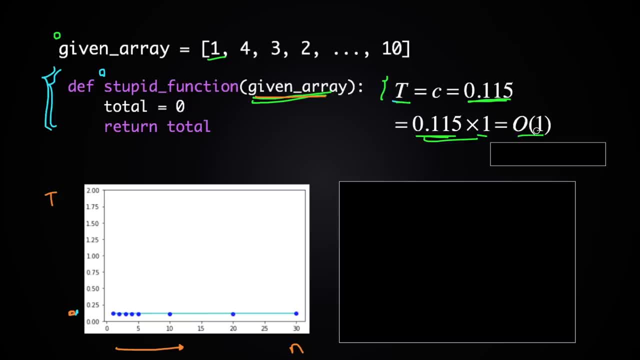 So you get: t is big O of one. This is actually equivalent to big O of two, big O of three, big O of 0.115, and so on. And you can technically choose any of those numbers, but by convention we usually use one here. So you can actually choose any of those numbers, but by convention we usually use one here. So you can technically choose any of those numbers, but by convention we usually use one here. So you can technically choose any of those numbers, but by convention we usually use one here. 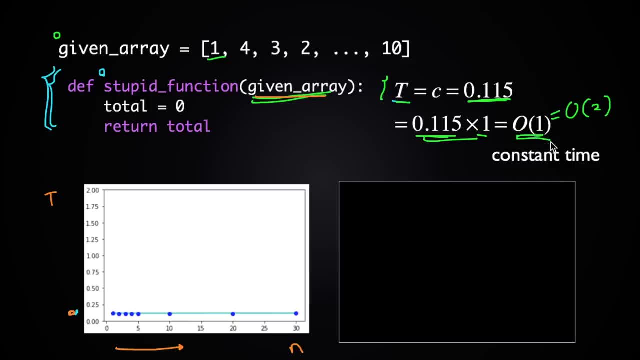 inside the big O expression, And this is, of course, constant time, because the time here is constant. Now let's say you have two functions solving the same problem, Not necessarily something stupid like this, but you know a problem that's more meaningful. 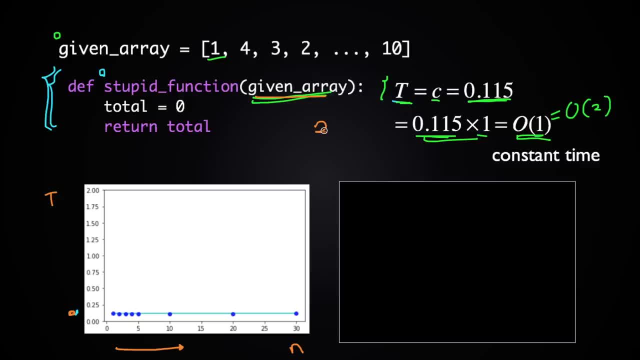 something that you actually want to solve, And let's say, you wrote two functions for solving that problem, And one of them happens to take only constant time, so the graph looks like this, And the other one takes linear time, so the graph might look like this that we saw earlier. 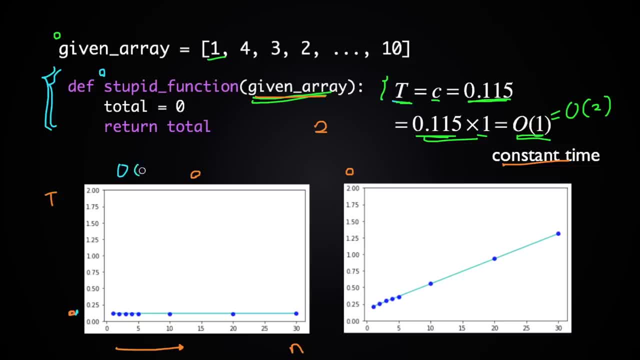 And so the first function takes big O of one in time, and the second function takes big O of n in time, where n is the size of the input. And they solve the same problem, And once you compare these two functions it'll be clear that the second function will take more time. 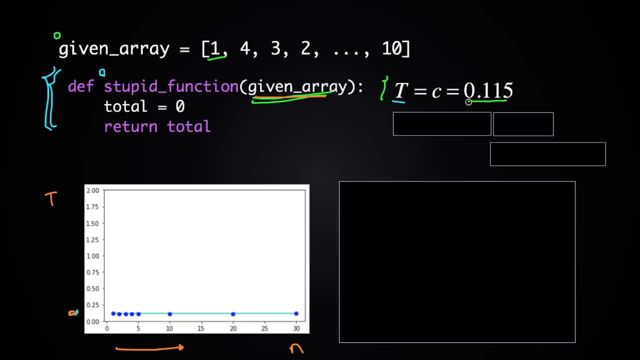 out the coefficient. But this whole thing is a coefficient, So how should we think about it? One way to think about it is that 0.115 can be rewritten as 0.115 times one. So when you take out 0.115 out of this expression, you're left with 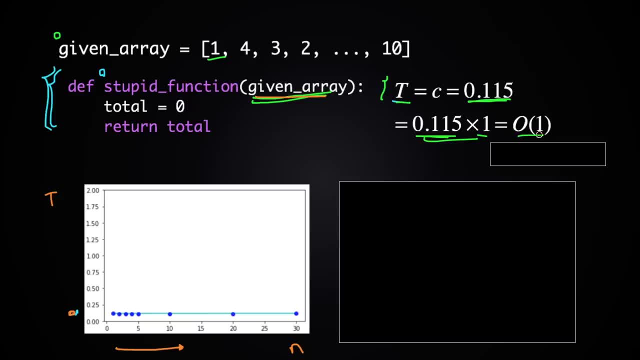 one. So you get t is big O of one. This is actually equivalent to big O of two, big O of three, big O of 0.115, and so on. And you can technically choose any of those numbers, But by convention we usually use one here inside the big O expression, And this is of course. 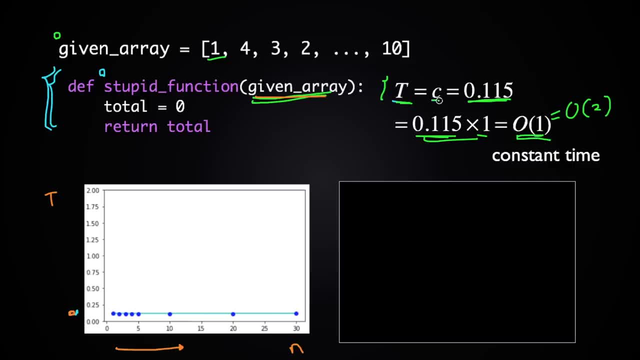 constant time, Because the time here is constant. Now let's say you have two functions solving the same problem, not necessarily something stupid like this, But you know a problem that's more meaningful, something that you actually want to solve. And let's say you wrote two functions. 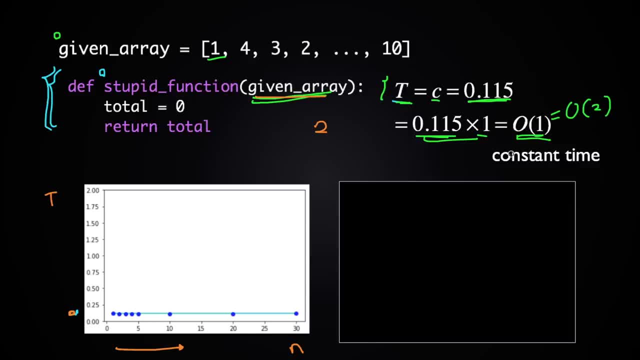 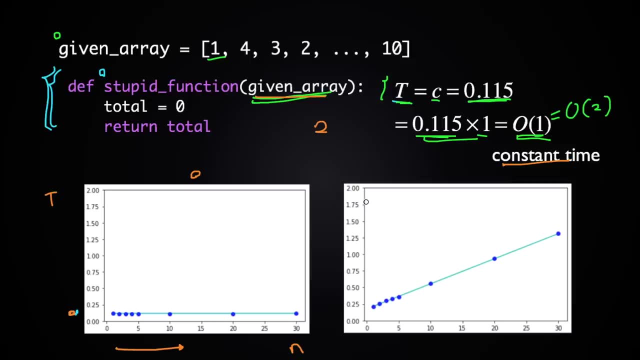 for solving that problem, And one of them happens to take only constant time, So the graph looks like this, And the other one takes linear time, So the graph might look like this that we saw earlier, And so it takes. the first function takes Big O of one in time, And the second function takes: 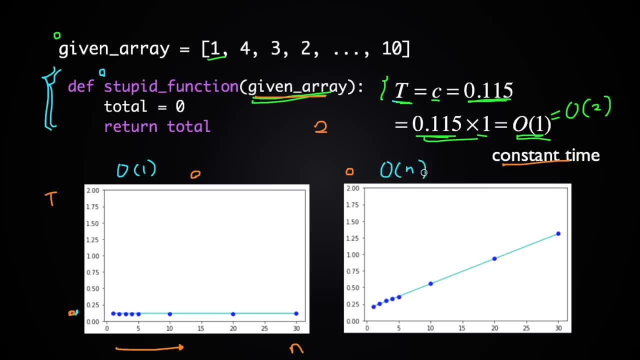 big O of n in time, where n is the size of the input, and they solve the same problem. And once you compare these two functions, you'll be clear that the second function will take more time when n is large enough, regardless of where the constant is. So if the constant is here, as in the grid. you can follow this line of numbers. You can clearly visualize what these based on, because it's this informal planning of the complex x. We are free from the large function. We are free from the consortium option. However, this is clearly driven by two functions And if some, 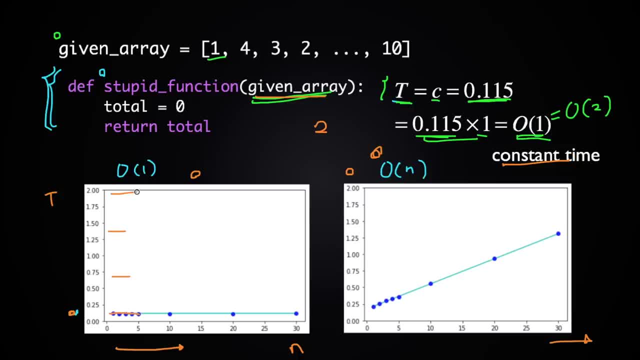 graph, or here, here, or here, when n is large enough, the second function takes more time. So, as you can see from that example, another benefit of using Big O notation and time complexity is that they allow you to quickly compare multiple functions in terms of their performance. 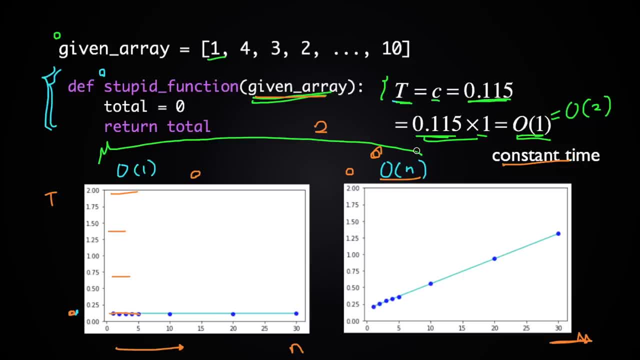 In this particular example, if you can achieve the same thing, constant time is probably better than linear time, or O of 1 is better than O of n. Now, time complexity is not the only factor that you should consider when you're trying to decide between multiple potential solutions for. 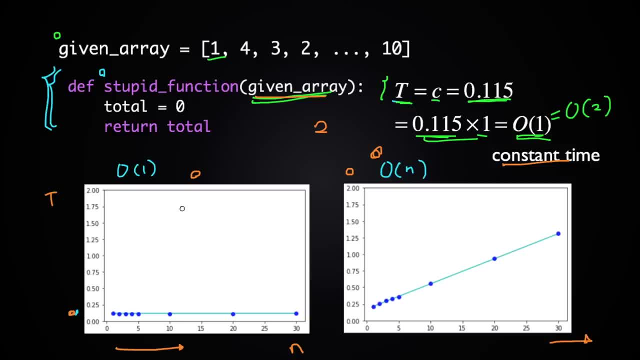 when n is large enough, regardless of where the constant is. So if the constant is here, as in the graph, or here, here, or here, when n is large enough, the second function takes more time. So, as you can see from that example, 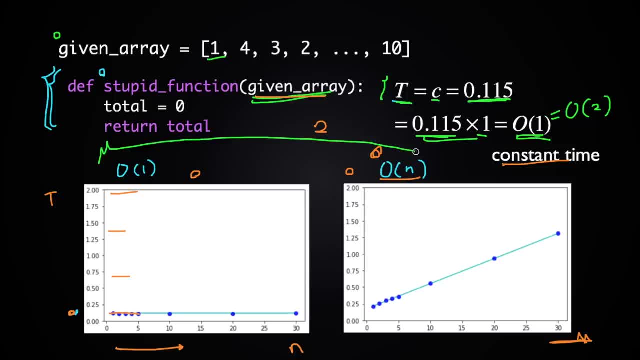 another benefit of using big O notation and time complexity is that they allow you to quickly compare multiple functions in terms of their performance. In this particular example, if you can achieve the same thing, constant time is probably better than linear time, or O of one is better than O of n. 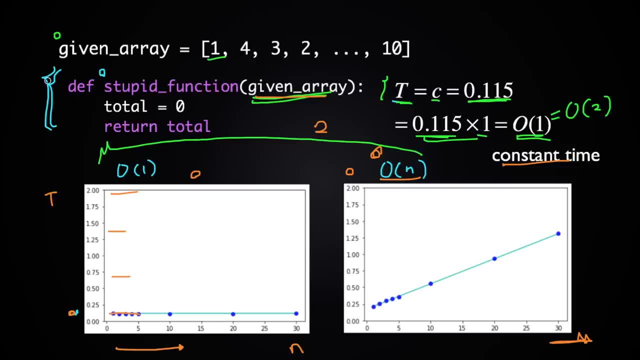 Now time. complexity is not the only factor that you should consider when you're trying to decide between multiple potential solutions for a single problem. For example, you should consider how easy it is to read your code and how much memory each of your potential functions consumes. 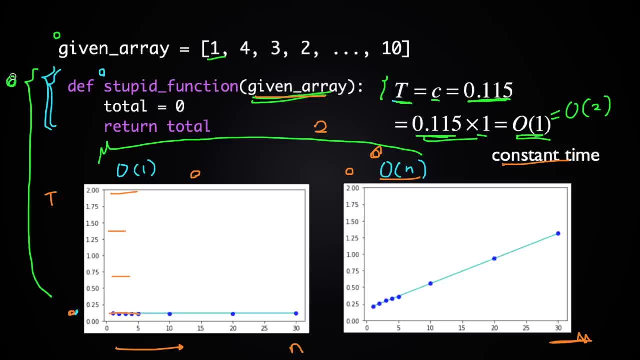 But time complexity is definitely one of the factors that you should consider. Okay, so so far, what we've done to find the time, complexity and the big O of a given function is that we run this function many, many times for many, many different inputs. 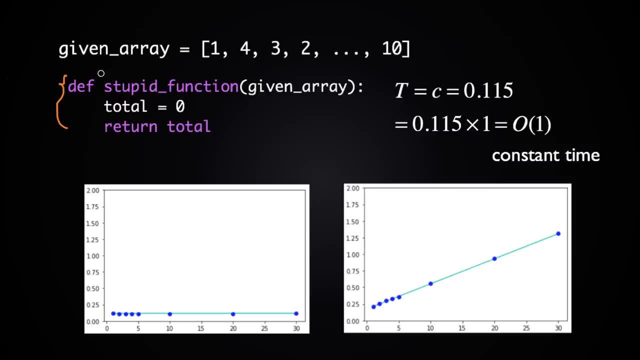 and then we found the average time it takes to run this function for each size of the input. We plotted the results on the graph and then, using those graphs, we found the time, complexity and big O. But that's actually a lot of work to you know. 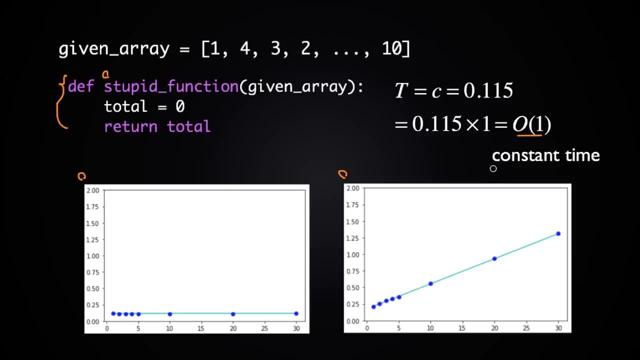 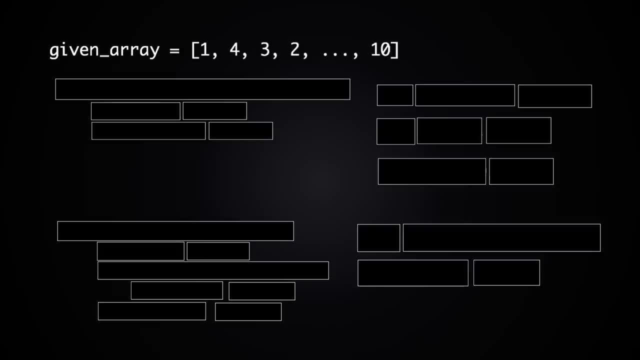 conduct an experiment every time we have a function, So is there any way to find the time, complexity and big O without running an experiment? There is, so let's take a look Here, just like before, we have the stupid function which takes the given array. 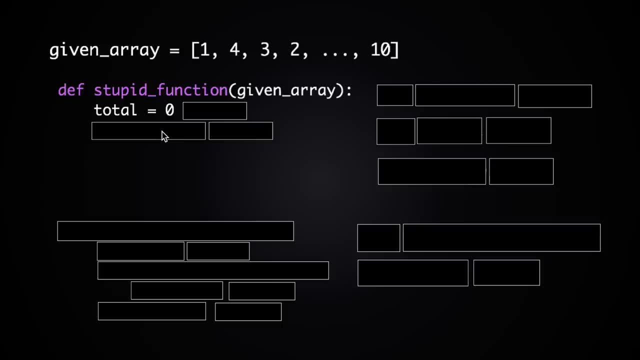 and in this function we initialize the total variable to zero and then we return that variable. Now, what if we didn't know the time complexity of this function yet and we wanted to find it without running any experiments? Well, the first step for doing that, 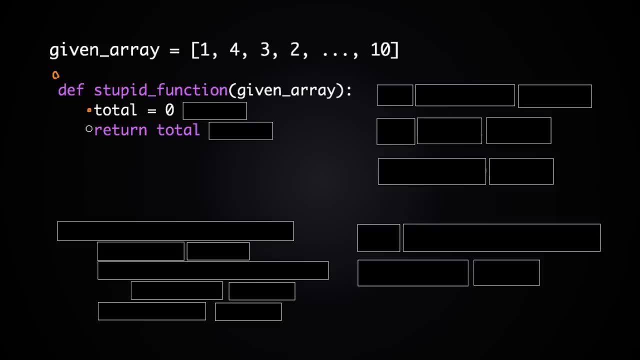 would be to consider each of these lines and then ask yourself: how much time does it take to execute each of these lines? Well, let's take a look at the first line. This line initializes a variable called Total, and the assigns the number zero to that variable. 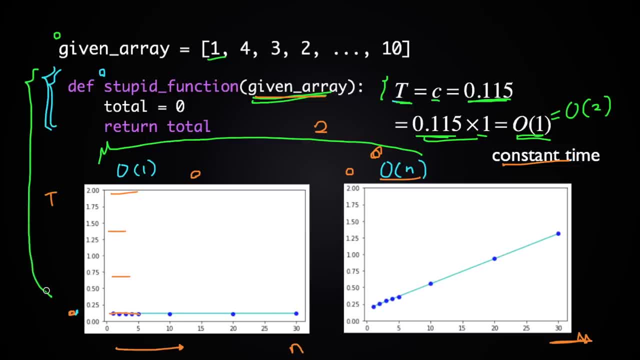 a single problem. For example, you should consider how easy it is to read your code and how much memory each of your potential functions consumes, But time complexity is definitely one of the factors that you should consider. Okay, so so far, what we've done to find the time complexity. 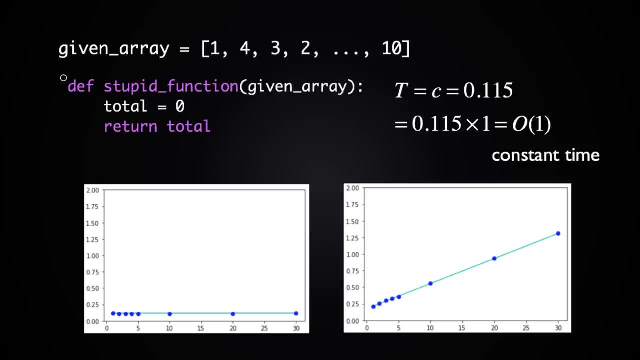 and time complexity is that we've found that time complexity is better than linear time, and the Big O of a given function is that we run this function many, many times for many, many different inputs and then we found the average time it takes to run this function for each size. 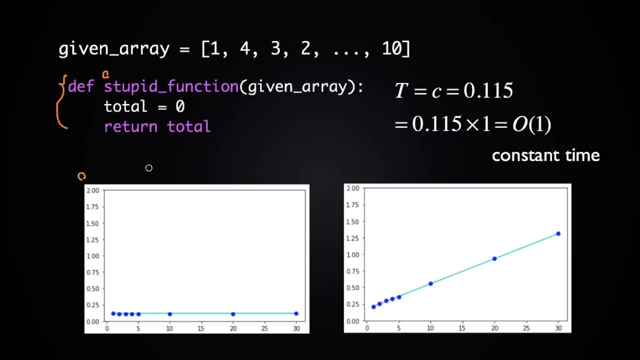 of the input. We plotted the results on the graph and then, using those graphs, we found the time, complexity and Big O. But that's actually a lot of work to you know, conduct an experiment. every time we have a function. So is there any way to find the time, complexity and Big O without running an? 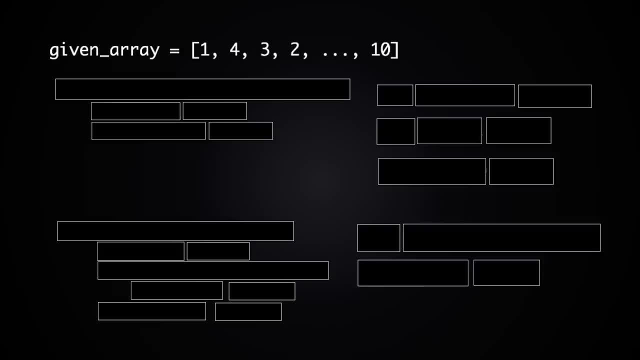 experiment. Well, there's a way to do that. So let's take a look at the time, complexity and Big O There is. so let's take a look Here, just like before, we have the stupid function which takes the given array, And in this function we initialize the total variable to zero, and then we 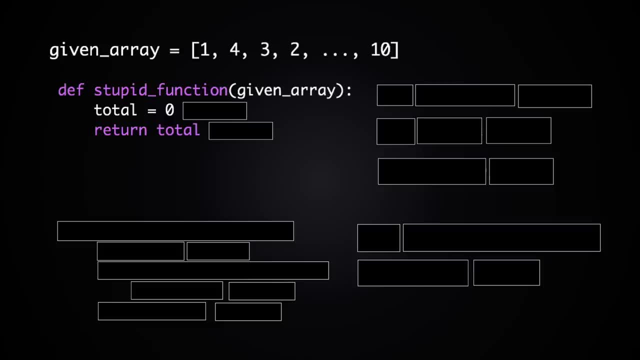 return that variable. Now, what if we didn't know the time complexity of this function yet and we wanted to find it without running any experiments? Well, the first step for doing that would be to consider each of these lines and then ask yourself: how much time does it take to? 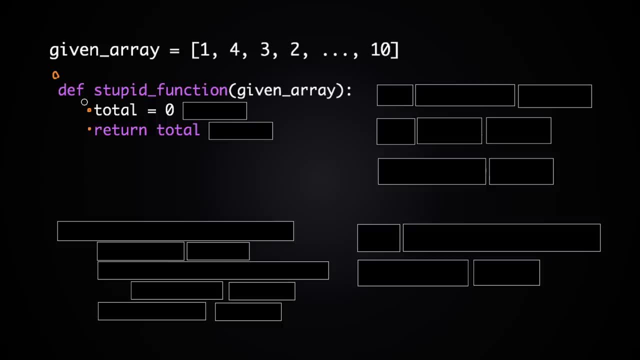 execute each of these lines. Well, let's take a look at the first line. This line initializes a variable called total and then assigns the number zero to that variable. If you think about it, it doesn't depend on the given array at all, because we're just assigning the same number. 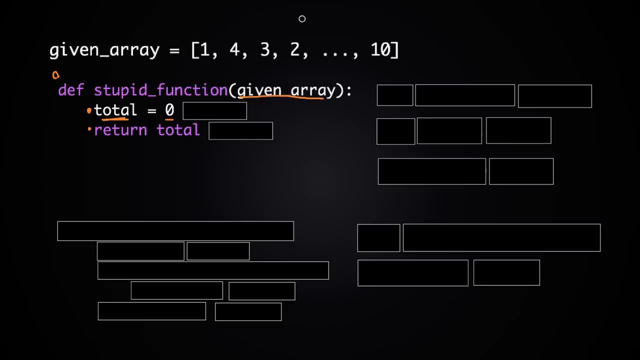 every time. So no matter how big or small the given array is, this line should take pretty much the same amount of time every time. So it should take a constant amount of time every time, Or in other words, the time it takes to execute this line is big O of one, And similarly for the second line. 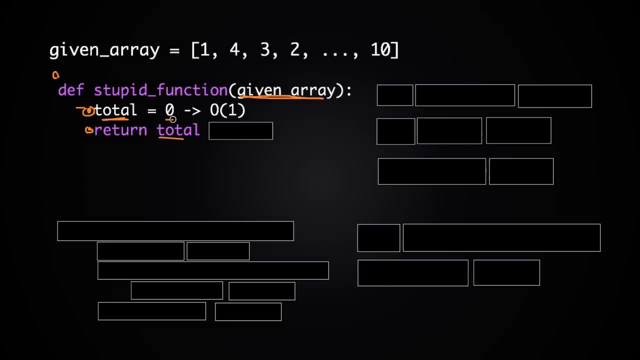 we're returning the same number every time, which is zero in this case, So it should take a constant amount of time every time as well, no matter how big or small the given array is. So the runtime of the second line is also O of one. And here what's nice about big O is that once you have 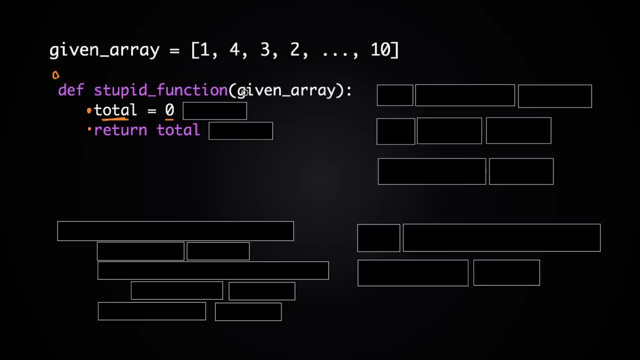 If you think about it, it doesn't depend on the given array at all, because we're just assigning the same number every time. So no matter how big or small the given array is, this line should take pretty much the same amount of time every time. 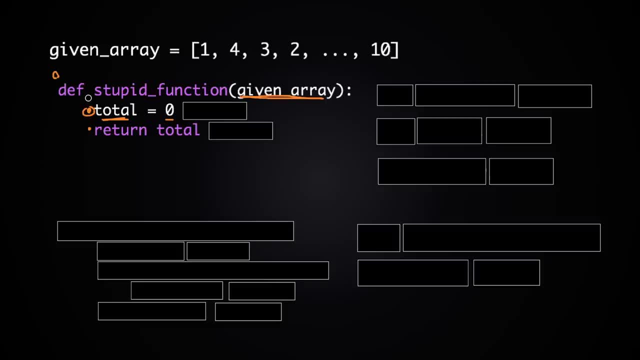 so it should take a constant amount of time every time, Or in other words, the time it takes to execute this line is big O of one, And similarly for the second line, we're returning the same number every time, which is zero in this case. 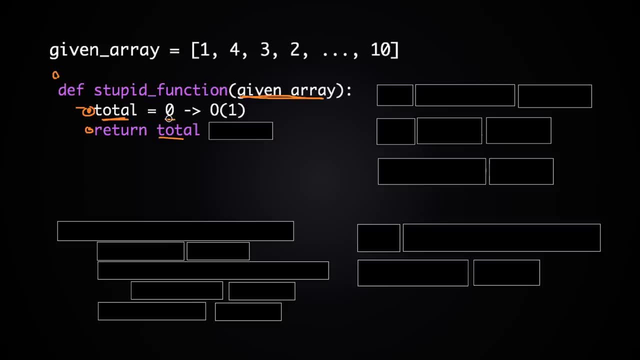 So it should take a constant amount of time every time as well, no matter how big or small the given array is. So the runtime of the second line is also O of one. And here, what's nice about big O is that once you have these big O expressions, 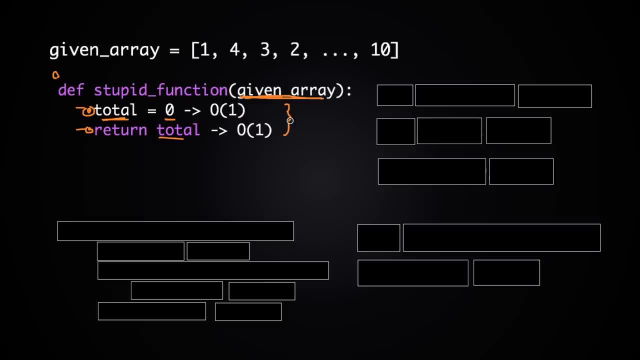 for each of these lines in a function. you can just add all of them up to find the total amount of time it takes to run this entire function. So let's do that right here. Let's call T the time it takes to run this entire function. 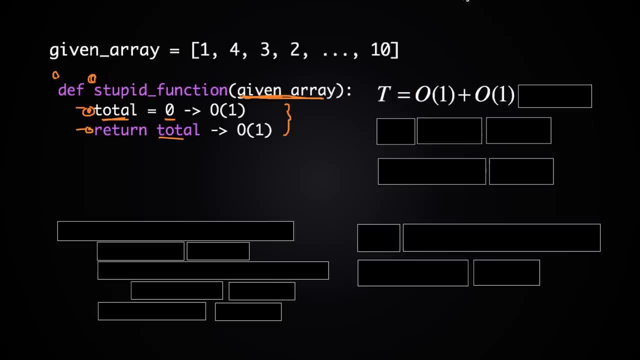 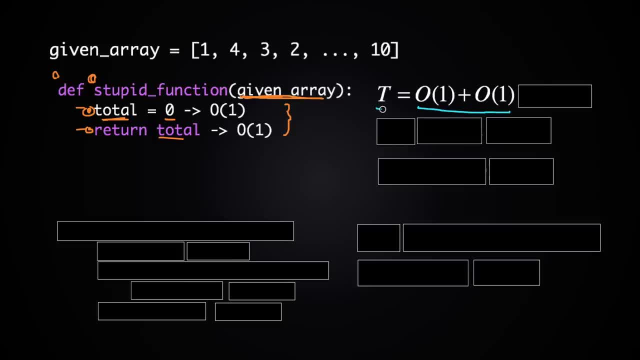 O of one is just a constant. So this is just saying T is the sum of two constants, whatever those constants are. So you can, for example, rewrite this as C one plus C two, by calling the first constant C one and the second constant C two. 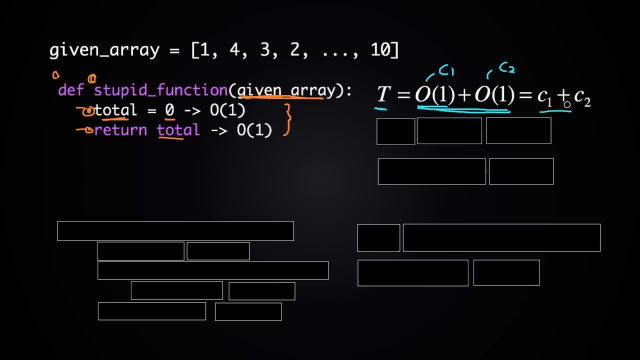 So I just rewrote T as C one plus C two, And then, once you add up two constants, you get another constant. Let's just call that C three. And so what we found just here is that T is just a constant which we're calling C three here. 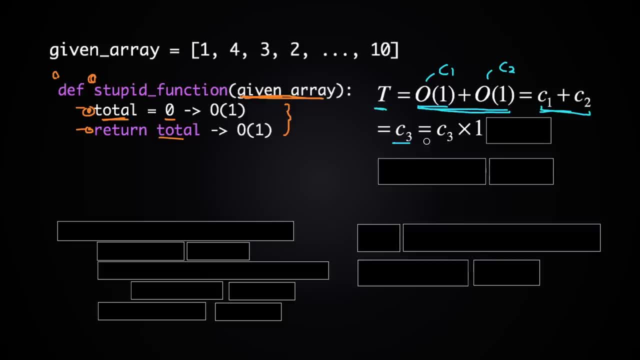 And then, as we saw earlier, we can rewrite C three, a constant, as C three times one, And then we have only one term here. So this is the fastest growing term out of this time: T. So we can just take out the coefficient C three. 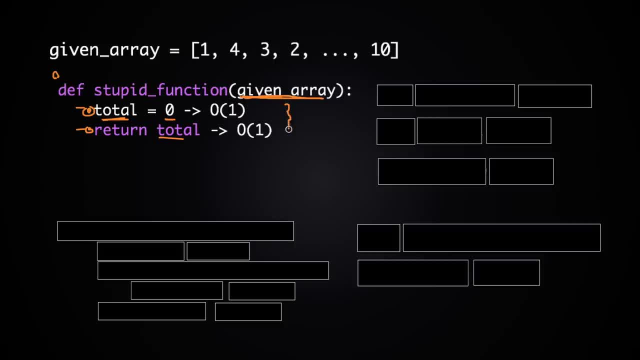 these, you know big O expressions. for each of these lines in a function, you can just add all of them up to find the total amount of time it takes to run this entire function. So let's do that right here. Let's call T the time it takes to run this entire function. stupid function. 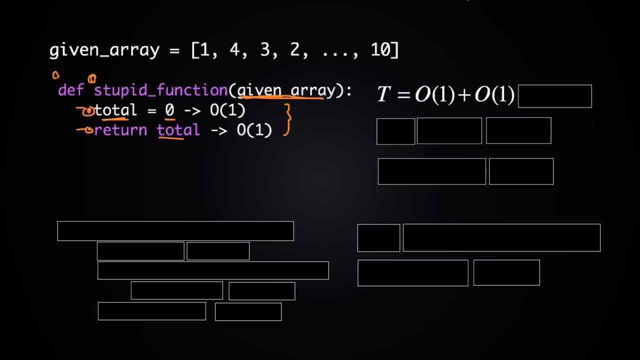 and that's going to be O of one plus O of one. And to find the sum of these two big O expressions you can just go back to what O of one is. And if we remember from the previous section, O of one is just a constant. So this is just saying T is the sum of 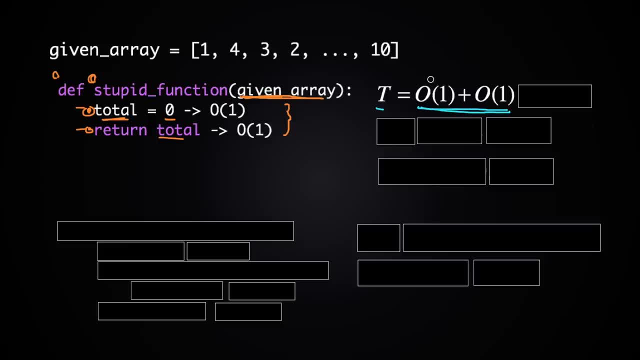 two constants, whatever those constants are. So you can, for example, rewrite this as C one plus C two by calling the first constant C one and the second constant C two. So I just rewrote T as C one plus C two, And then, once you add up two constants, you get another constant. 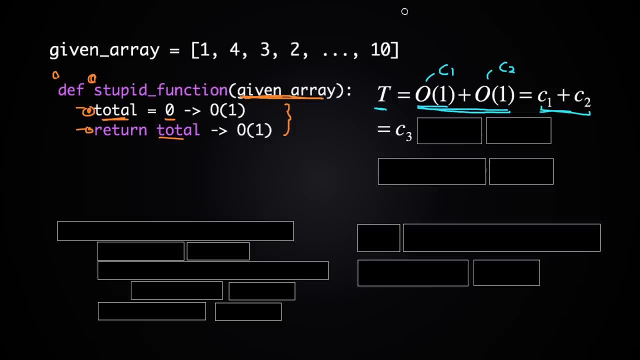 let's just call that C three, And so what we found just here is that T is just a constant, which we're calling C three here, And then, as we saw earlier, we can rewrite C three, a constant, as C three times one, And then we have only one term here. So this is the fastest growing term. 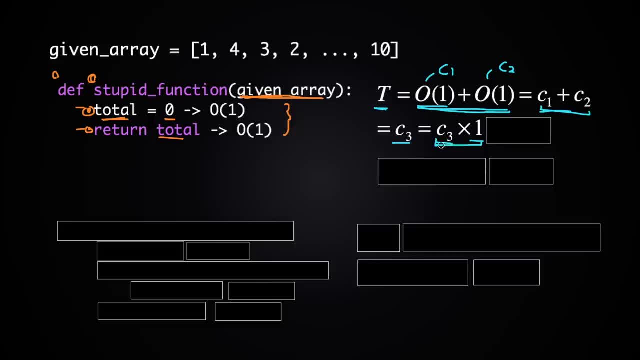 out of this time T, So we can just take out the coefficient C three and what we get is just O of one. So what we just found here is that when you add up two constant time- O of one and O of one- 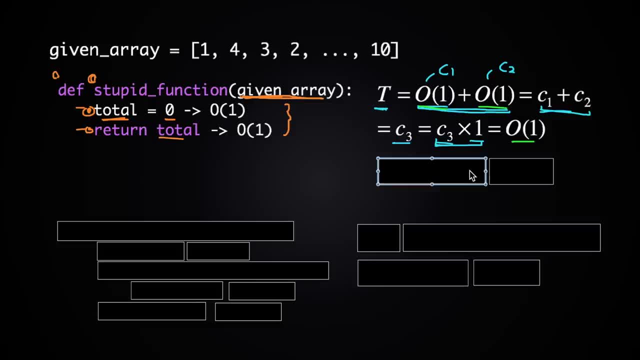 you just get O of one back, And that's generally true as well. So O of one plus O of one is equal to O of one in general. Anyway, let's take a look at another example here. Here we have the first example we saw earlier: find sum, which takes given array as the input And then in the function, 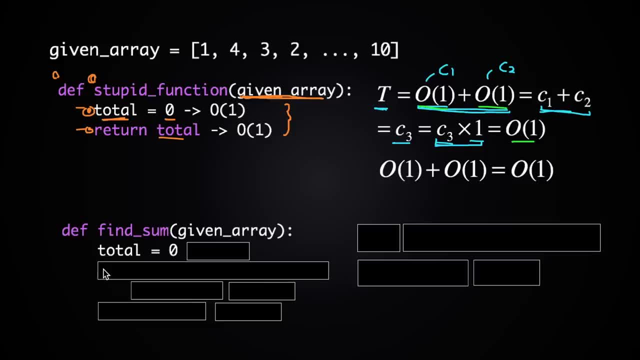 first of all we initialize total to zero And then we run a for loop for each I in given array or for each number in the given array, And then in the for loop we say: add I or each of those numbers to total And at the end of the function we return total. 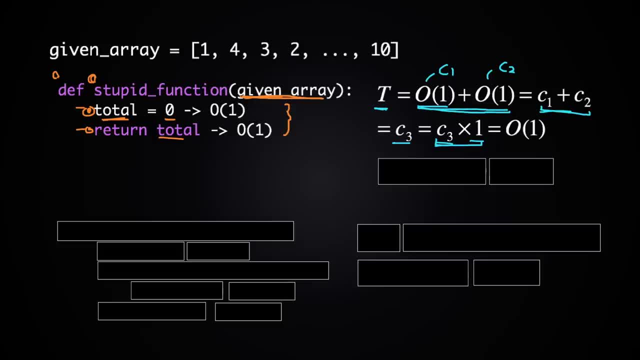 And what we get is just O of one. So what you just found here is that when you add up two constant time- O of one and O of one- you just get O of one back, And that's generally true as well. 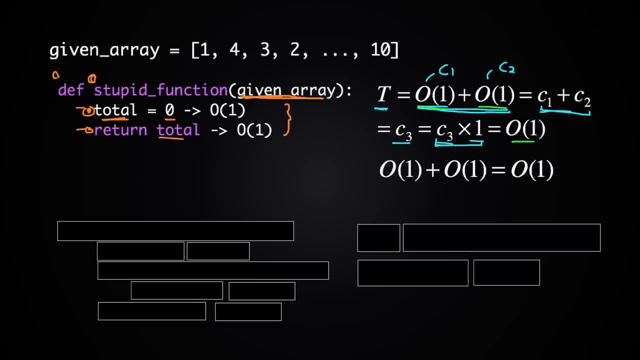 So O of one plus O of one is equal to O of one in general. Anyway, let's take a look at another example here. Here we have the first example we saw earlier, findSum, which takes given array as the input And then in the function, 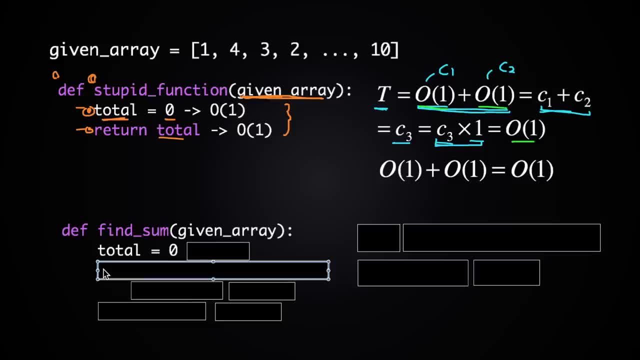 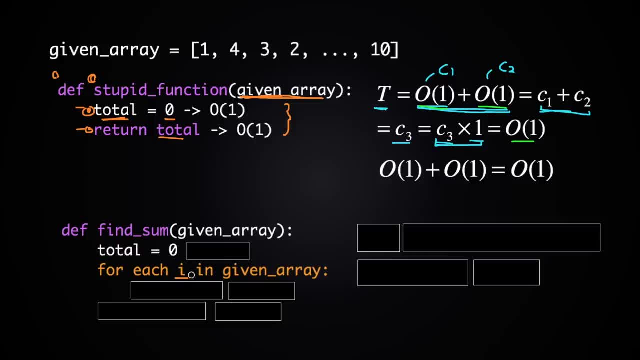 And then we run a for loop for each i in given array, And then we run a for loop for each i in given array Or for each number in the given array, And then in the for loop we say: add i or each of those numbers to total. 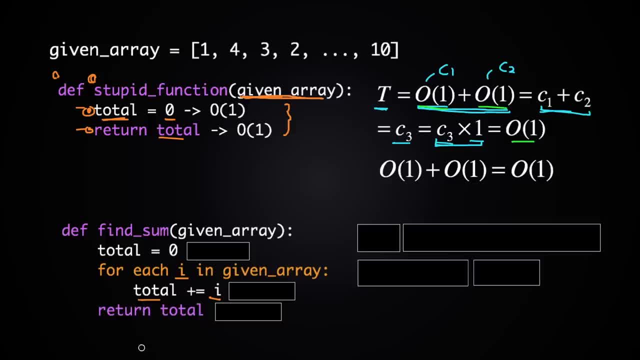 And at the end of the function we return total And that way we can find the sum of all the numbers in the given array. And what if we wanted to find the time, complexity and big O of this function To do that? we can go through the same process. 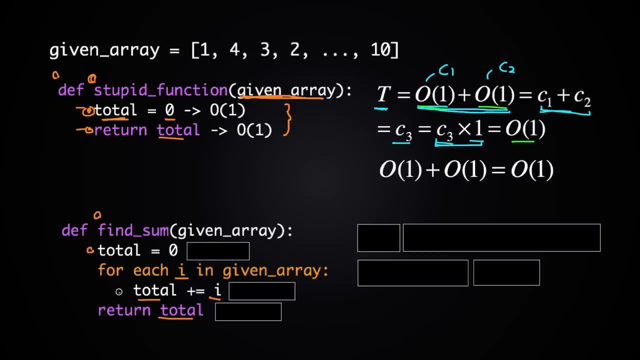 So look at each line and think about how much time it takes to execute each of those lines. So total equals zero. It's the same as before. It only takes a constant amount of time, or just big O of one, And return total. the last line is the same thing. 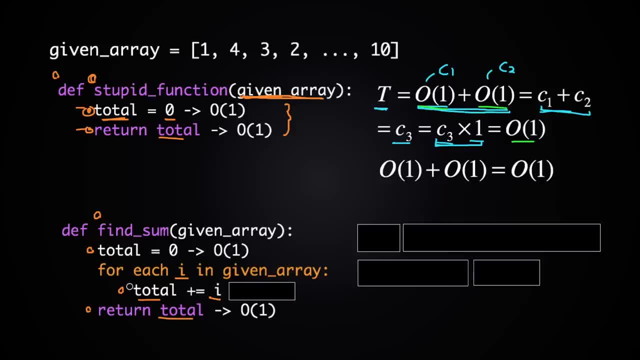 Just O of one. And if you look at inside this for loop, total plus equals i. we're just adding up a number, you know, a single number to total, And, assuming that the range is fairly reasonable, you know, let's say i is always somewhere between. 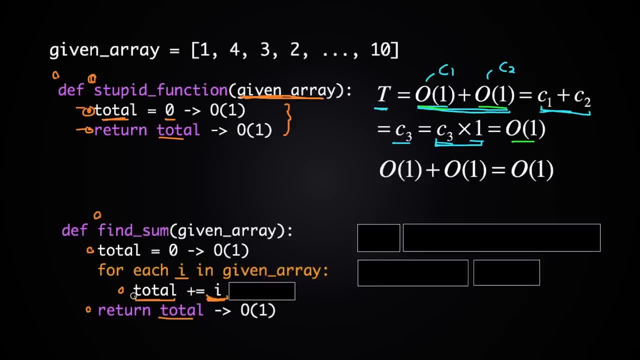 you know, zero to 10, and that's the same as before. So this operation actually takes roughly the same amount of time every time, or a constant amount of time every time, no matter how big or small the given array is. So this line actually only takes big O of one as well. 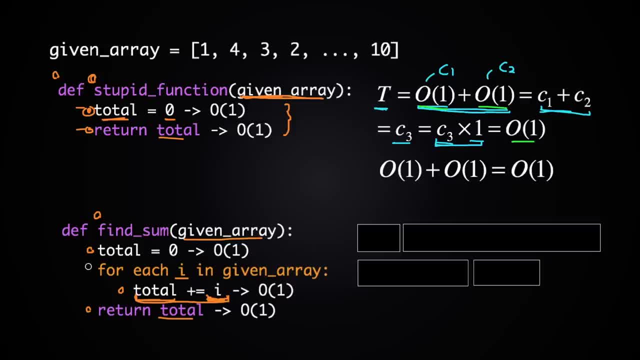 And then, if you want to be a little bit more rigorous about this, you can also think about how much time setting up this for loop takes- and that's actually O of one as well- And once you have all of that, you can just add them up to find the total amount of time. 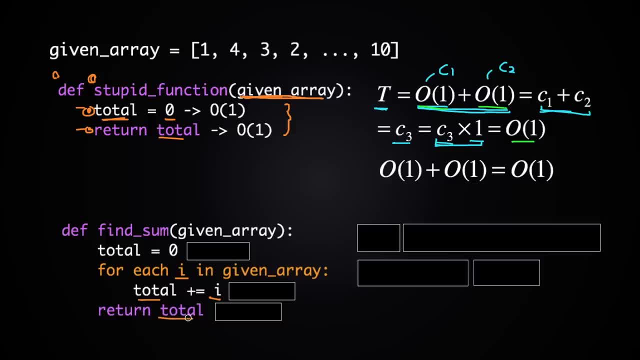 And that way we can find the sum of all the numbers in the given array. And what if we wanted to find the time, complexity and big O of this function? To do that? we can go through the same process. So look at each line and think about how much time it takes to find the sum of all the 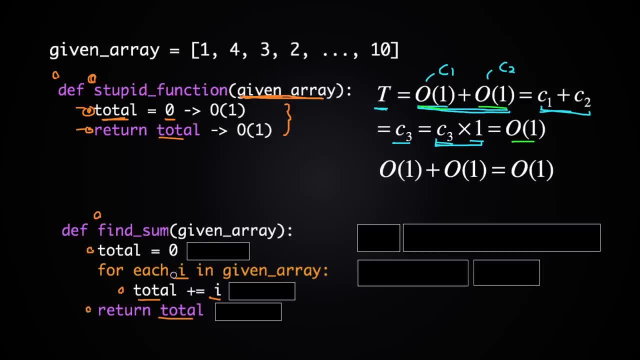 numbers to execute each of those lines. So total equals zero. it's the same as before. it only takes a constant amount of time, or just big O of one And return total. the last line is the same thing, just O of one. And if you look at inside this for loop, total plus equals I. we're just 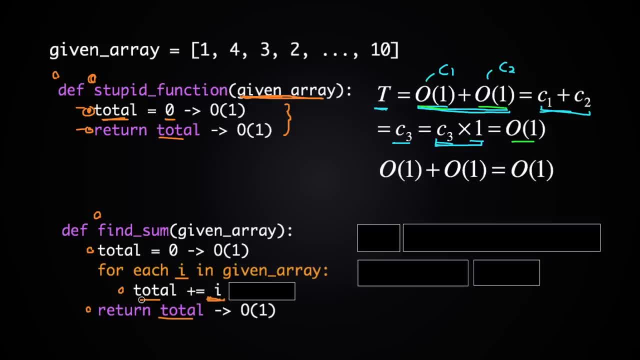 adding up a number. you know a single number to total And assuming that the range is fairly reasonable, you know, let's say, I is always somewhere between. you know one and two. you know zero to 10, this operation actually takes roughly the same amount of time every time. 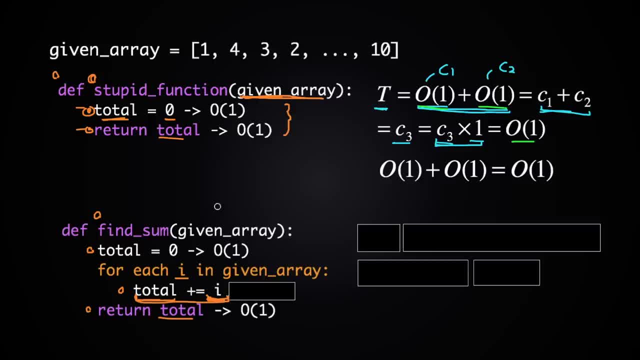 or a constant amount of time every time, no matter how big or small the given array is. So this line actually only takes big O of one as well, And then, if you want to be a little bit more rigorous about this, you can also think about how much time setting up this for loop takes. 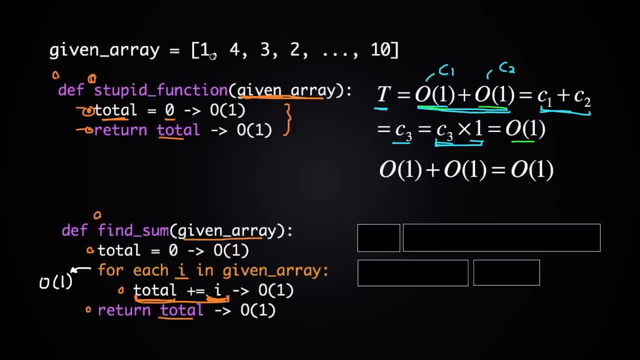 And that's actually O of one as well. And once you have all of that, you can just add them up to find the total amount of time it takes to execute this entire function: find sum. So let's call that time t2.. And that's going to be something like this: O of one plus n times O of one plus O. 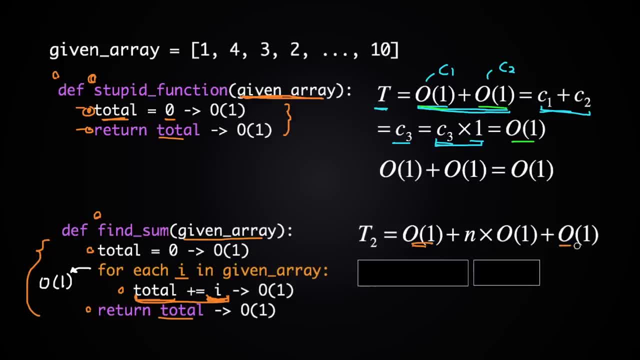 of one. So these two O of ones at the beginning and at the end come from these two lines. you could add another O of one if you want to be a little bit more rigorous for setting up the for loop right here And then between these two lines you can add another O of one if you want to be a 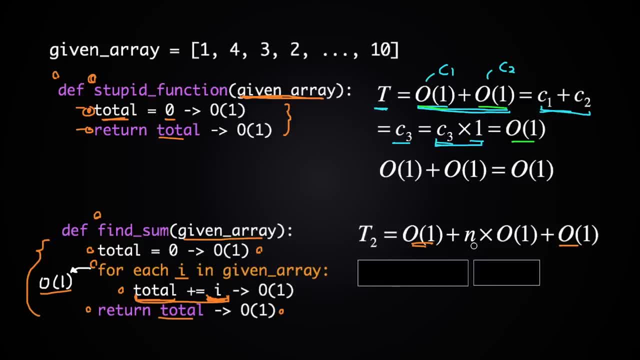 little bit more rigorous for setting up the for loop right here And then between these two lines, these two O of ones. we have N times O of one because we have this line right here which takes O of one and we need to execute this line N times. 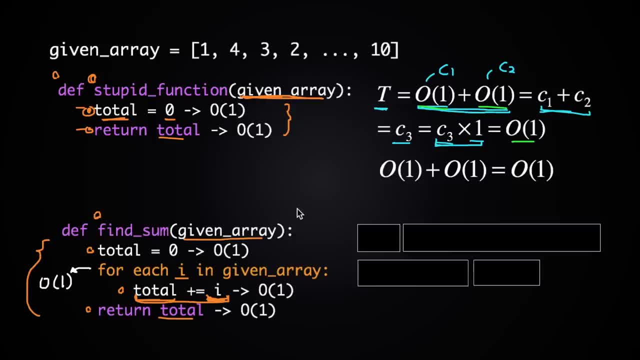 to execute this entire function, find sum. So let's call that time T2.. And that's going to be something like this: O of one plus N times, O of one plus O of one, So these two O of ones at the beginning and at the end. 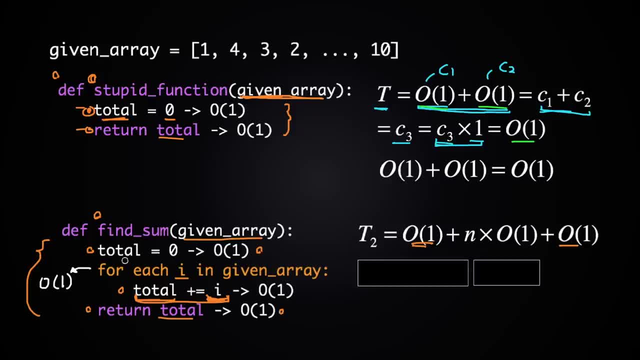 come from these two lines. You could add another O of one if you want to be a little bit more rigorous for setting up the for loop right here, And then between these two O of ones, we have N times O of one because we have this line right here. 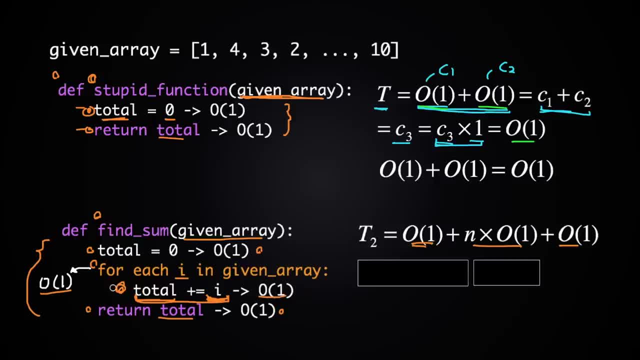 which takes O of one, And we need to execute this line N times because we need to repeat this process, you know, adding I to total N times, where N is the number of items in the given array, And that's why we have N times, big O of one here. 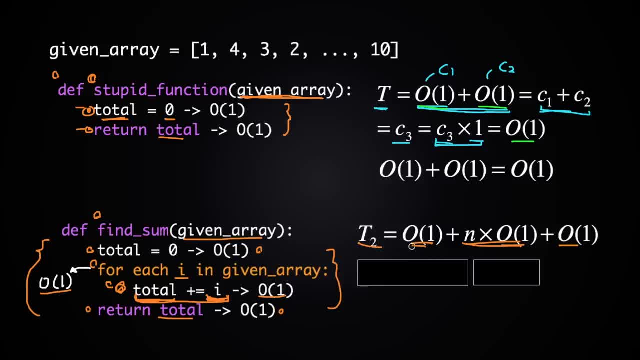 So adding that all up, we get T2 is O of one plus N times O of one plus O of one, And to find what this whole expression should look like it should be in the end, we just need to go back to you know. 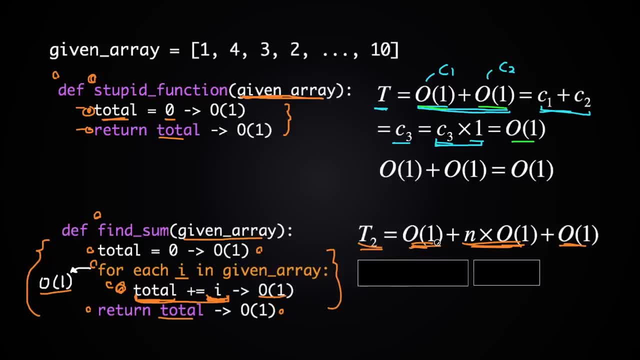 just like before, what O of one stands for? And it stands for a constant. And here we have a bunch of O of ones. you know two or three, depending on how you count them And when you add up a bunch of O of ones. 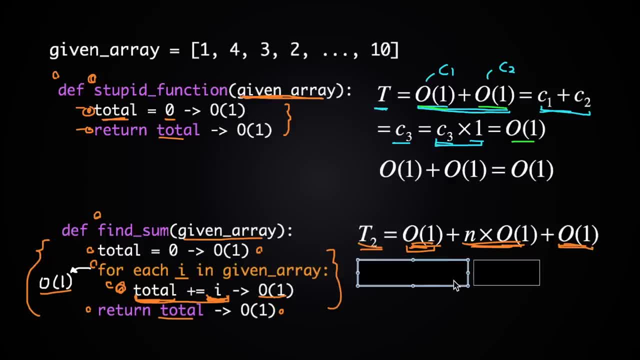 or a bunch of constants. you just get another constant. So let's call that constant C4. And then, for this O of one, let's call this constant C5. So we get this whole expression. T2, is equal to C4, a constant. 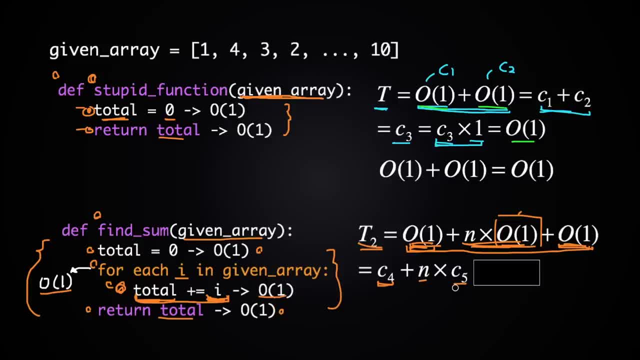 plus N times C5, which is another constant. And to find the big O expression that fits this whole expression, C4 plus N times C5, we can just follow the same steps that we reviewed earlier. So, first of all, find the fastest growing term. 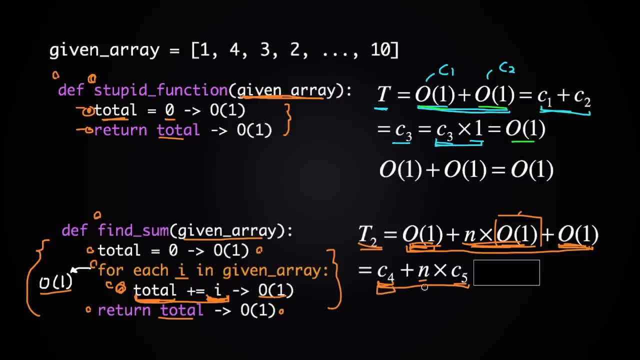 out of these two terms. We only have two terms here: C4 and N times C5.. And the fastest growing term here is N times C5, because that's the fastest growing term. That term actually grows as N grows larger, but C4 doesn't change because it's just a constant. 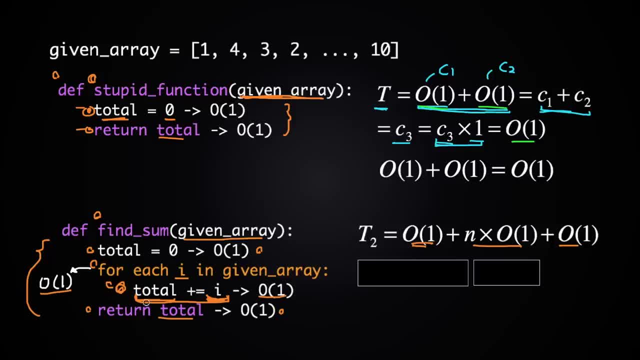 because we need to repeat this process. you know, adding I to total and times, where N is the number of items in the given array And that's why we have N times big O of one here. So adding that all up, we get T2 is O of one. 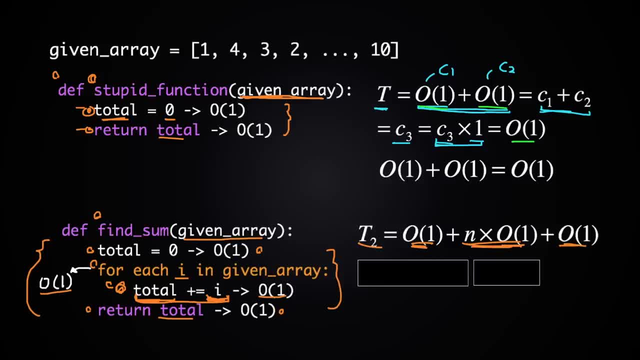 plus N times, O of one plus O of one. And to find what this whole expression should be in the end, we just need to go back to. you know, just like before, what O of one stands for, And it stands for a constant. 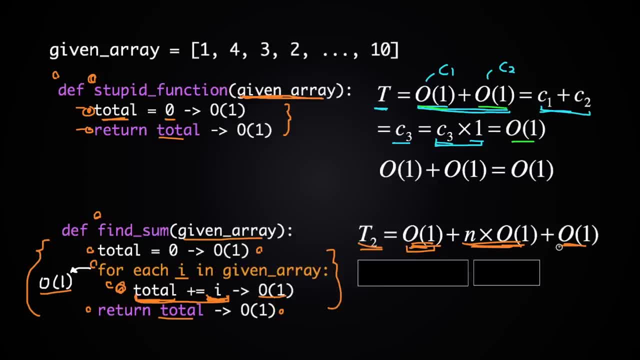 And here we have a bunch of O of ones, you know, two or three, depending on how you count them. And when you add up a bunch of O of ones or a bunch of constants, you just get another constant. So let's call that constant C4.. 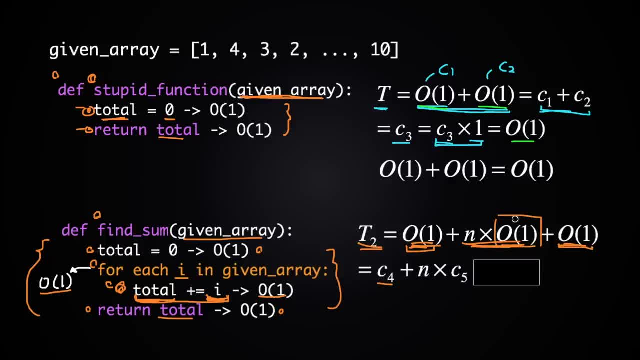 And then for this O of one, let's call this constant C5.. So we get this whole expression: T2 is equal to C4, a constant plus N times C5, which is another constant. And to find the big O expression: 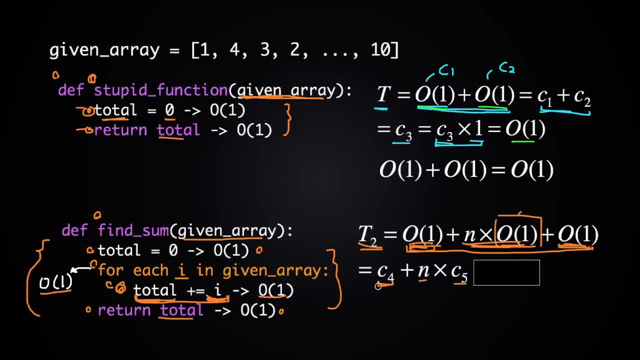 that fits this whole expression, C4 plus N times C5, we can just follow the same steps that we reviewed earlier. So first of all, find the fastest going term out of these two terms. We only have two terms here, C4 and N times C5. 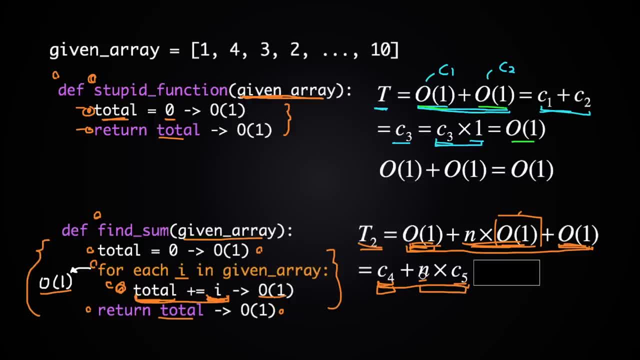 And the fastest growing term here is N times C5, because that term actually grows as N grows larger, but C4 doesn't change because it's just a constant. So the fastest growing term here is N times C5.. And the second step is removing the coefficient. 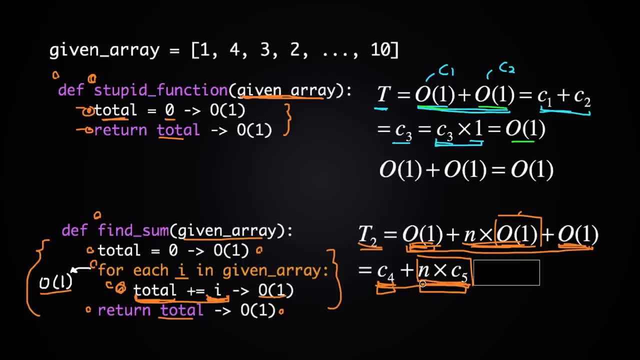 which is C5.. And once we do that, we get N and that's what should go inside the big O expression. So we get this is O of N. So we just found that the time it takes to execute this function find sum. 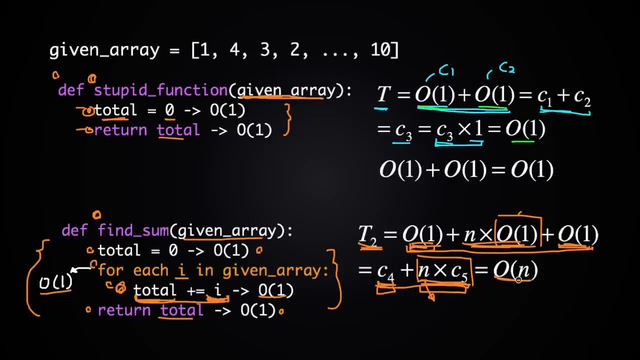 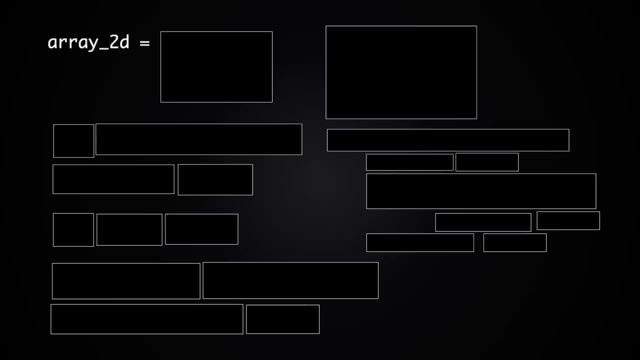 T2 is actually O of N or it's linear time. Okay, let's take a look at another example here, And this time we're given a different kind of input. We're going to call it array 2D and this is going to be a two-dimensional array. 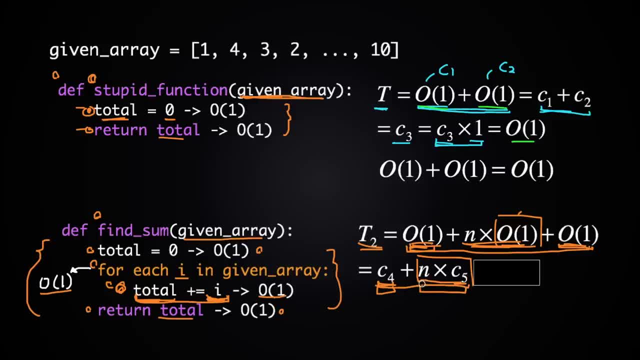 So the fastest growing term here is N times C5. And the second step is removing the coefficient which is C5. And once we do that we get N and that's what should go inside the big O expression. So we get this: is O of N. 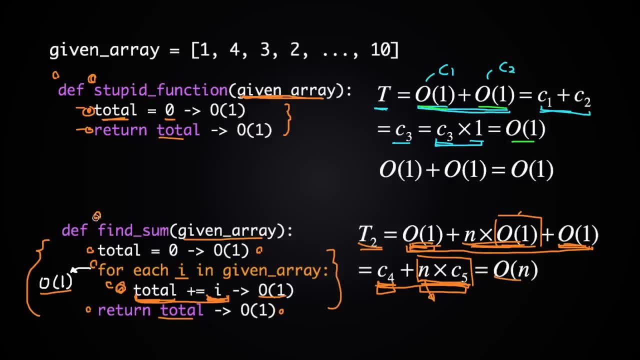 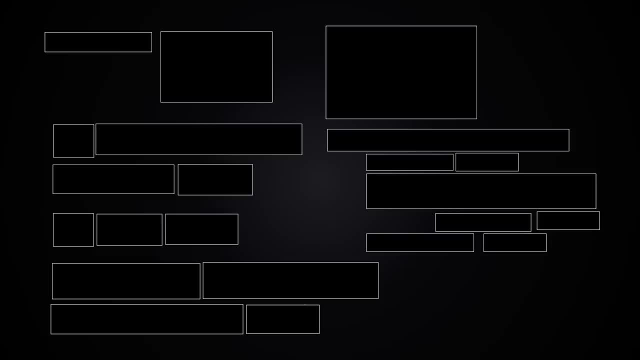 So we just found that the time it takes to execute this function, find sum T2, is actually O of N or it's linear time. Okay, let's take a look at another example here, And this time we're given a different kind of input. 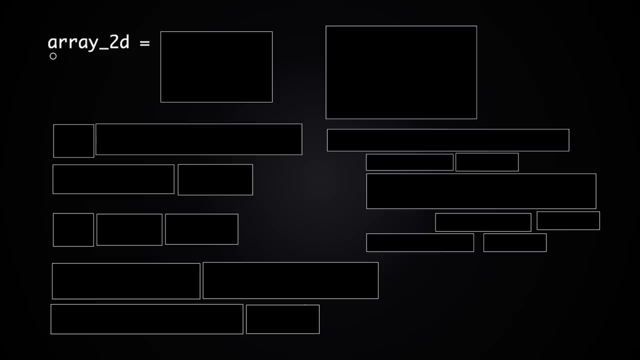 We're going to call it array 2D, and this is going to be a two-dimensional array. A two-dimensional array is basically an array of arrays, and it might look like this, for example: So this is an array of three arrays. 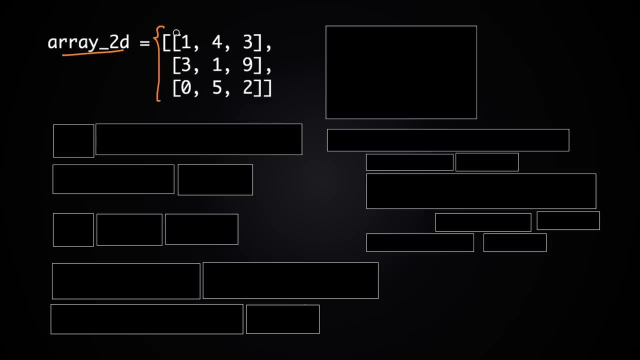 So this is an array, And the first element of this array is this array right here: one, four and three. And then the second element of the outer array is this second array right here: three, one and nine, And then in total we have nine elements. 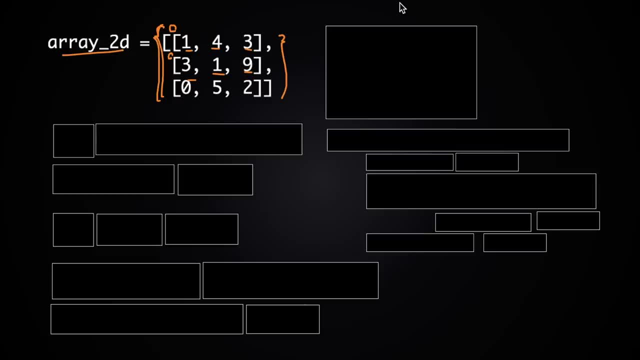 as you can see here, or nine numbers. And another example might look like this. This time this is an array of four arrays, So we have an array here and then the first element of this array is this array right here, with the elements one, four, three. 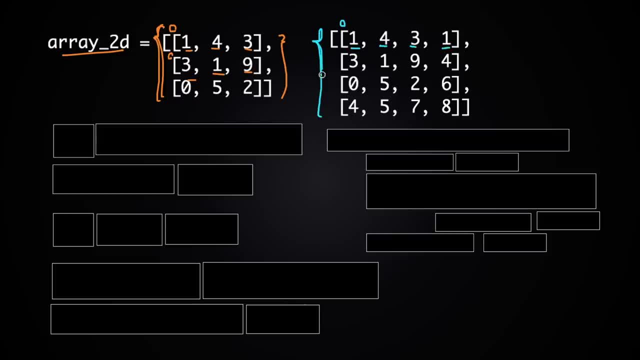 and one, And the second element of this entire array is this array, and the third element is this array, and the fourth element is this array, And then in total we have 16 numbers in this entire array. And then let's say that we are always given. 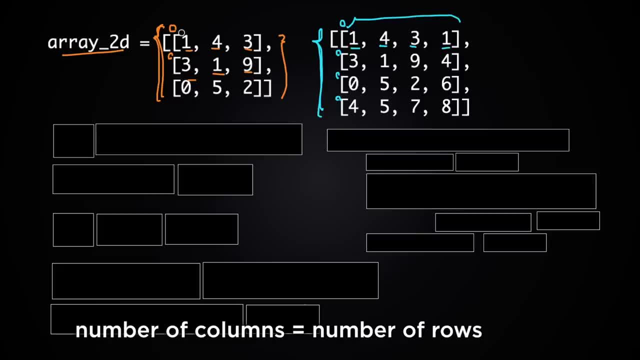 a square two-dimensional array which means that the number of columns is the same as the number of rows, And let's call the number of rows n. So that means that we have n columns and n rows in this given two-dimensional array. So we have n squared elements in the two-dimensional array. 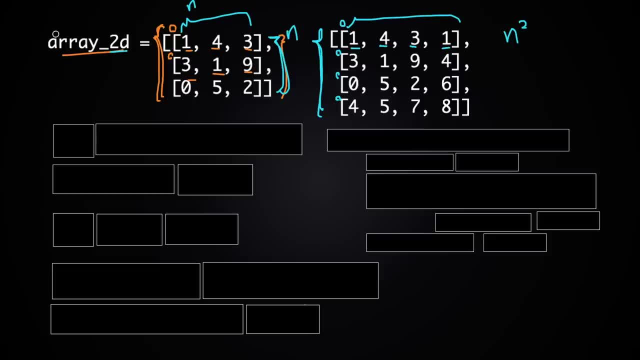 And let's say we want to write a function that takes one of these two-dimensional square arrays and then finds the sum of all the numbers inside the two-dimensional array, And that function might look like this: Let's call this function findSum2D. 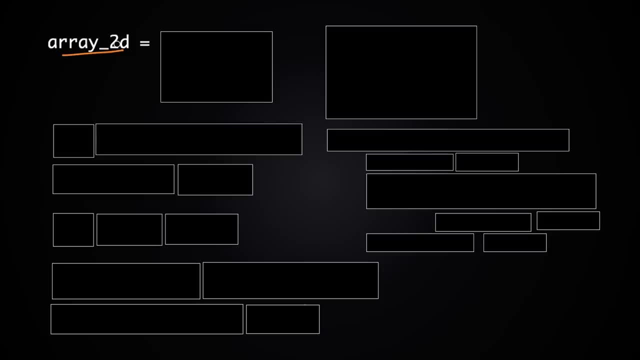 A two-dimensional array is basically an array of arrays and it might look like this, for example: So this is an array of three arrays, So this is an array. The first element of this array is this array right here: one, four and three. 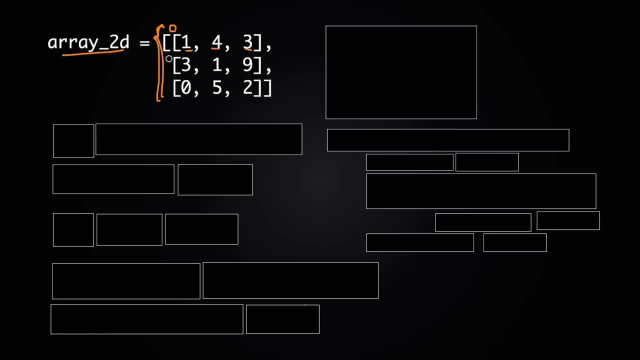 And then the second element of the outer array is this second array right here: three, one and nine, And then in total we have nine elements, as you can see here, or nine numbers, And another example might look like this: 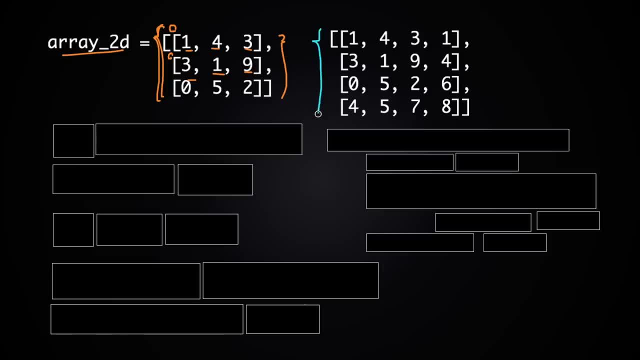 This time this is an array of four arrays. So we have an array here and then the first element of this array is this array, right here, with the elements one, four, three and one, And the second element of this entire array is this array. 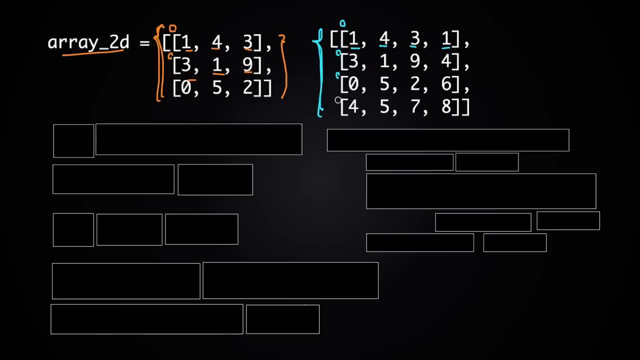 and the third element is this array, and the fourth element is this array, And then in total we have 16 numbers in this entire array. And then let's say that we are always given a square, two-dimensional array, which means that the number of columns 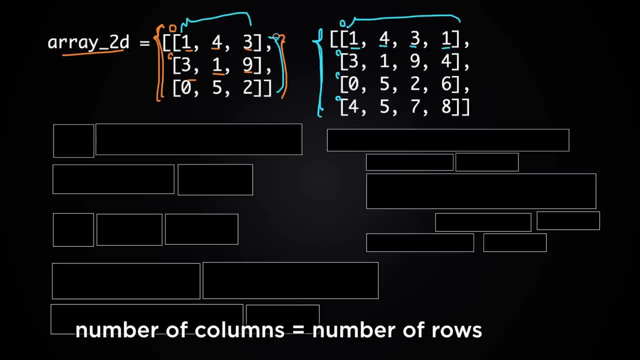 is the same as the number of rows, And so that means that we have n columns and n rows in this given two-dimensional array. So we have n squared elements in the two-dimensional array, And let's say we want to write a function that takes one of these two-dimensional square arrays. 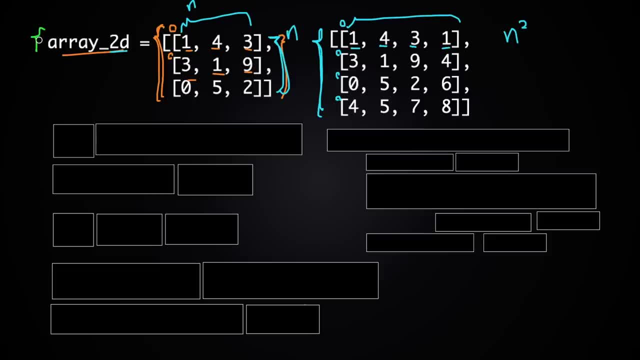 and then finds the sum of all the numbers inside the two-dimensional array. And that function might look like this: Let's call this function findSum2D and then it's going to take the given number, given two-dimensional array as input. 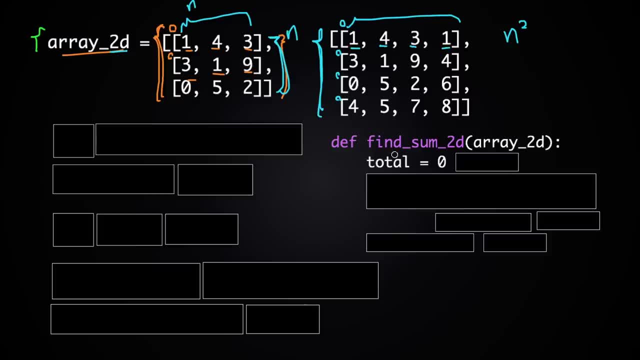 And in this function, first of all we're going to define a new variable called total and then assign number zero to it, And then we're going to run a for loop, actually a double for loop, and we'll say for each row in this two-dimensional array: 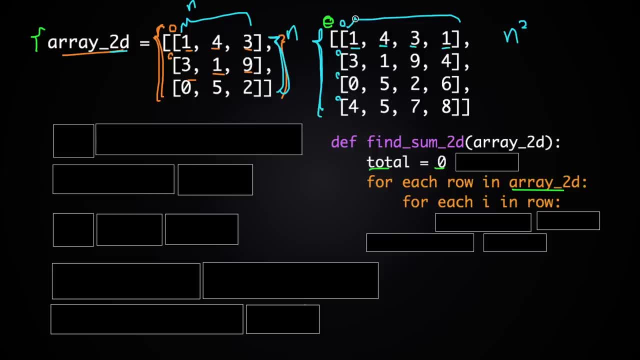 So that's, for example, if you're given this array right here, when I say for each row, I'm referring to this row, this row, this row, and then this row, And then in each of those rows, for each. 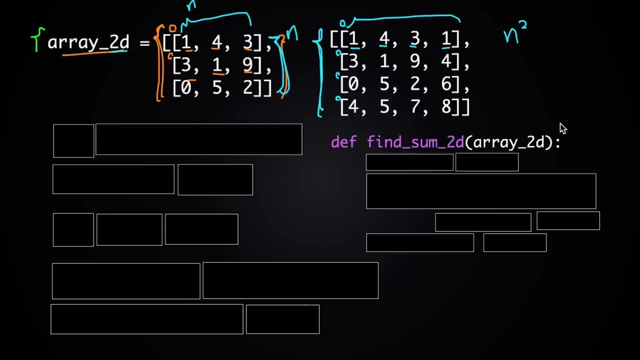 and then it's going to take the given two-dimensional array as input, And in this function, first of all we're going to define a new variable called total and then assign number zero to it, And then we're going to run a for loop. 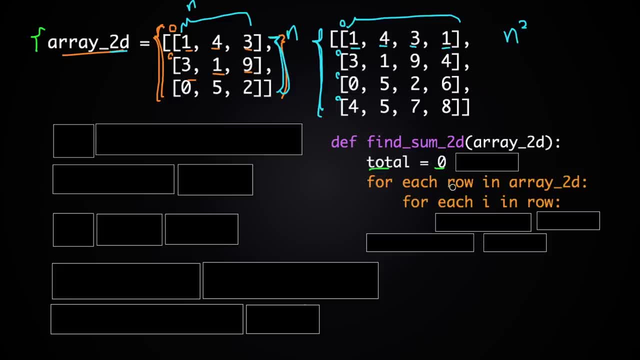 actually a double for loop And we'll say: for each row in this two-dimensional array. So that's, for example, if you're given this array right here, when I say for each row, I'm referring to this row, this row, this row and then this row. 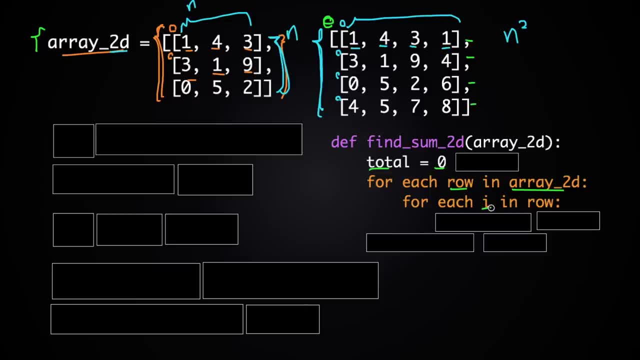 And then in each of those rows, for each i or for each number. So if we're looking at, let's say, this second row right here or the second array right here, each number would be this number, this number, this number and then this number. 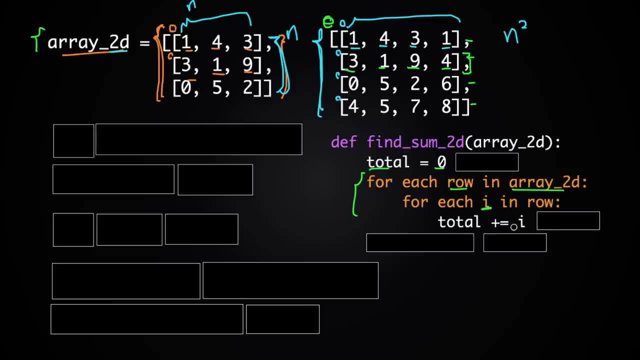 We want to add i or each of those numbers to total. So we just wrote total plus equals i here, And then at the end of this function or after we're done with this double for loop, we're going to return total. 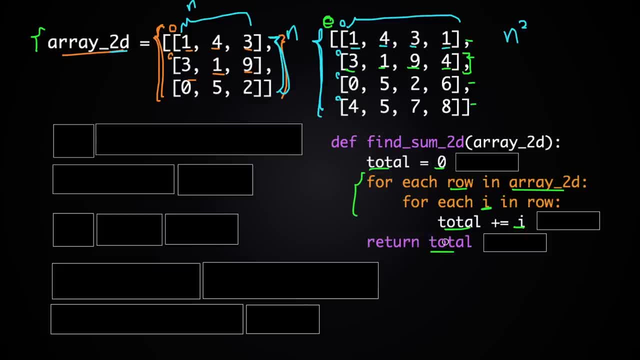 And that way we'll be able to find the sum of all the numbers in the given two-dimensional array and then return that number And here To find the time, complexity and big O notation of this function, findSum2D. we can go through the same process. 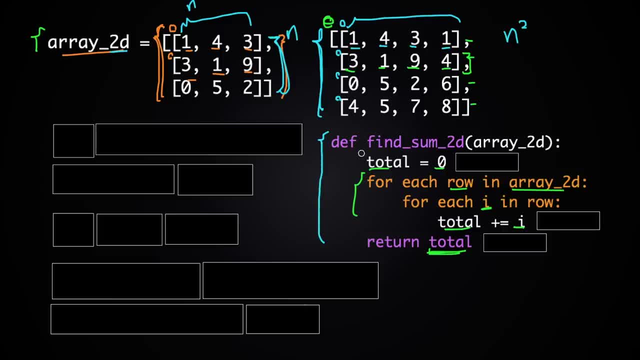 as the one we saw just earlier. So let's take a look at the first line here: total equals zero. defining a new variable called total and then assigning number zero to it. It only takes a constant amount of time. It doesn't depend on the size of the input. 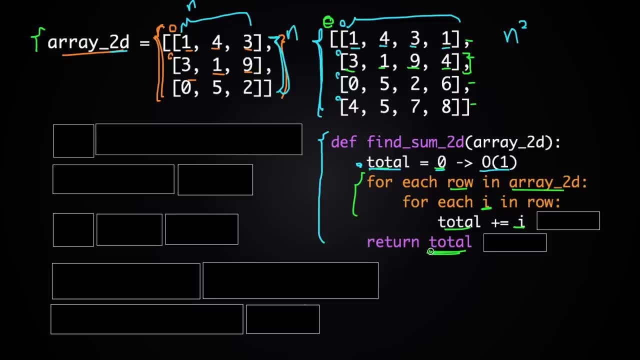 So that's O of one. And then the last line right here returning the total number. this is only gonna take a constant amount of time as well. So that's O of one as well. And this is assuming that the total, the sum of all the numbers in the given array. 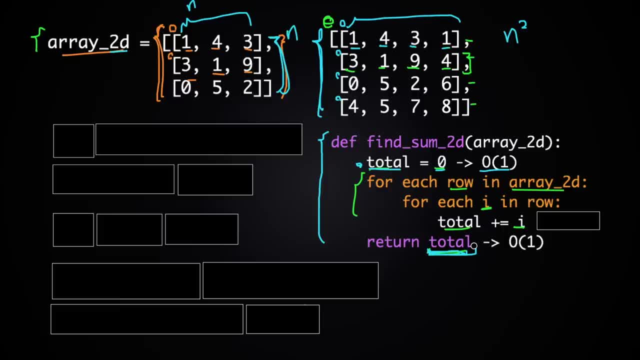 is reasonably small, And what I mean by that is that it's small enough so that it fits in a single integer variable, for example. And then, once you examine this line right here, total plus equals i. that only takes a constant amount of time as well. 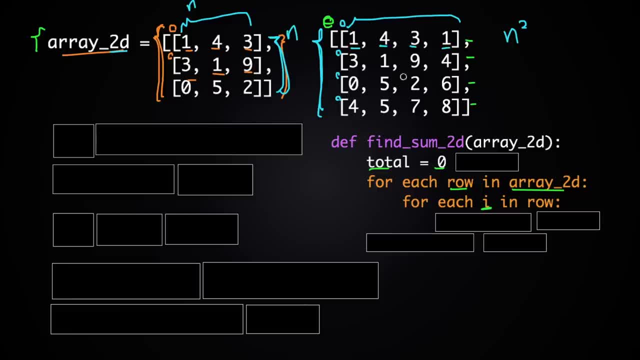 I or for each number. So if we're looking at, let's say, the second row right here or the second array right here, each number would be this number, this number, this number and then this number. We want to add I or each of those numbers to total. 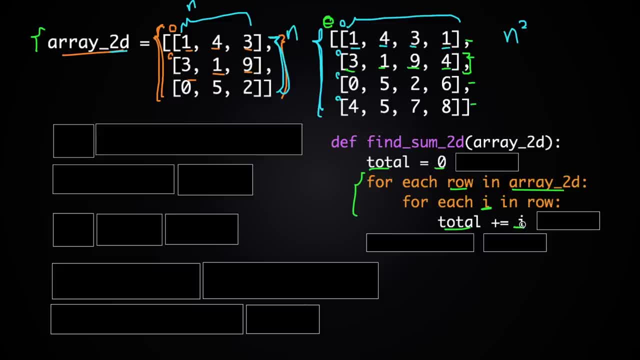 So we just wrote total plus equals I here, And then, at the end of this function or after we're done with this double for loop, we're going to return total, And that way we'll be able to find the sum of all the numbers. 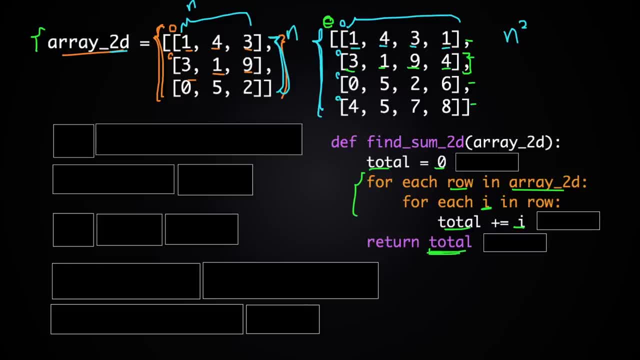 in the given two-dimensional array and then return that number And here to find the time, complexity and Big O notation of this function, findSum2D. we can go through the same process as the one we saw just earlier. So let's take a look at the first line here. 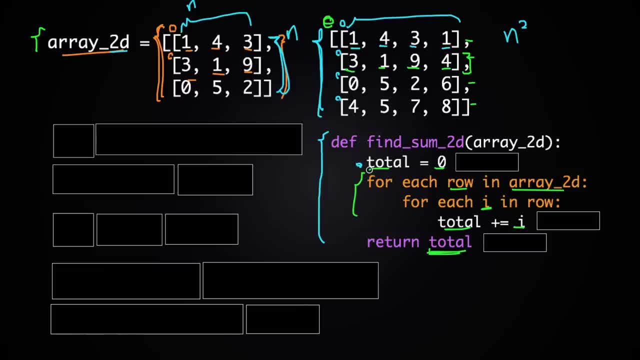 total equals zero. defining a new variable called total and then assigning number zero to it, It only takes a constant amount of time. It doesn't depend on the size of the input. So that's O of one, And then the last line right here. 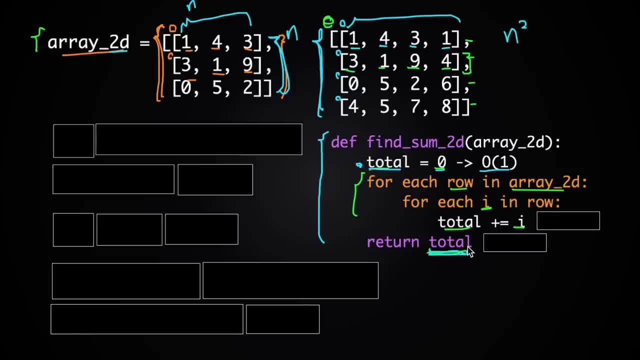 returning the total number. this is only going to take a constant amount of time as well. So that's O of one as well, And this is assuming that the total, the sum of all the numbers in the given array, is reasonably small. 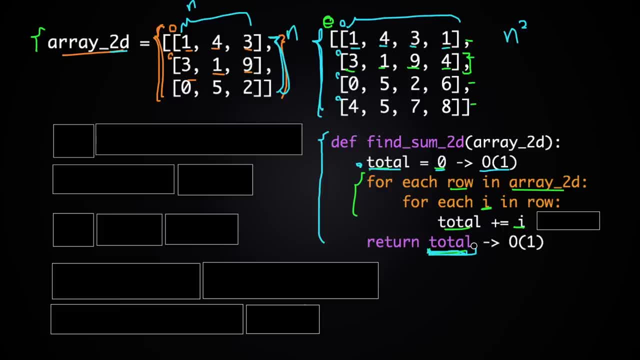 And what I mean by that is that it's small enough so that it fits in a single integer variable, for example. And then, once you examine this line right here, total plus equals I. that only fits into a single integer, only takes a constant amount of time as well. 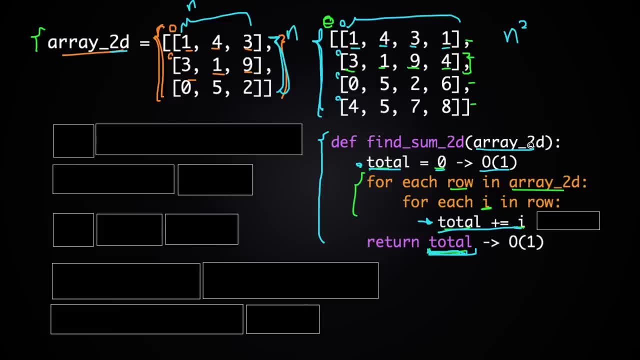 or it doesn't depend on the size of the input. Adding a number each time i to total should take roughly the same amount of time every time, regardless of how big or small the given array is. So that's also big O of one. 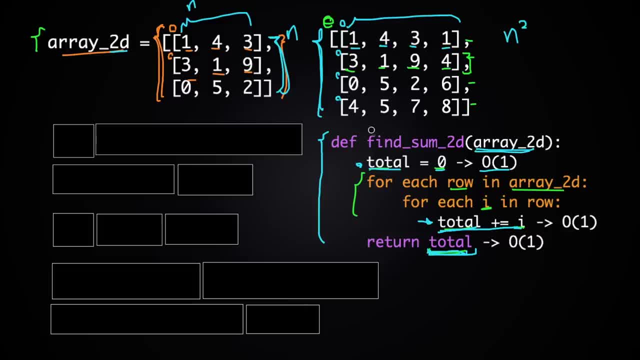 And to find the total amount of time it takes to execute this function, you just need to add all of them up, And I'm simplifying this argument just a little bit here. Anyway, let's call the time it takes to execute this whole function T3.. 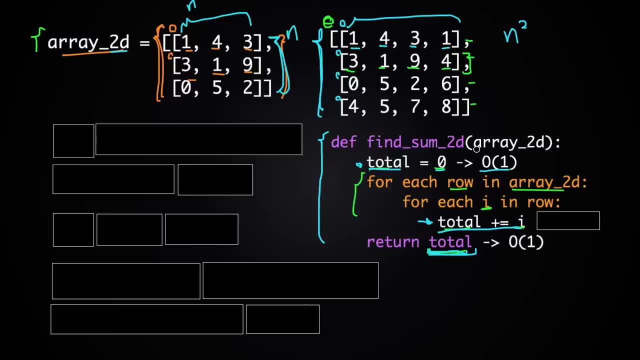 Or it doesn't depend on the size of the input. Adding a number each time i to total should take roughly the same amount of time every time, regardless of how big or small the given array is. So that's also big O of one. 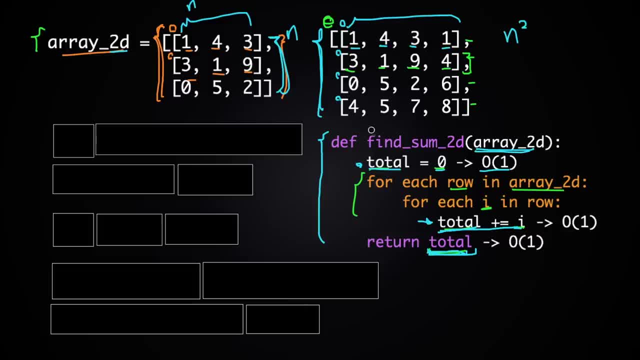 And to find the total amount of time it takes to execute this function, you just need to add all of them up, And I'm simplifying this argument just a little bit here. Anyway, let's call the time it takes to execute this whole function t and i. Let's call the time it takes to execute this whole function t and i. Anyway, let's call the time it takes to execute this whole function t and i. Let's call the time it takes to execute this whole function t and i. 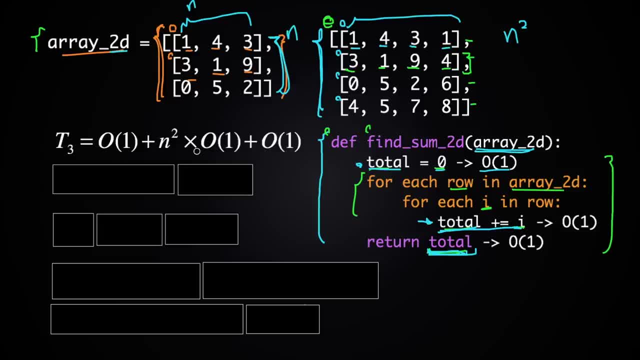 And that's gonna be O of one plus N, squared times O of one plus O of one. These two O of ones at the beginning and at the end come from these two lines at the beginning and at the end of this function. And then this O of one come from this line right here. 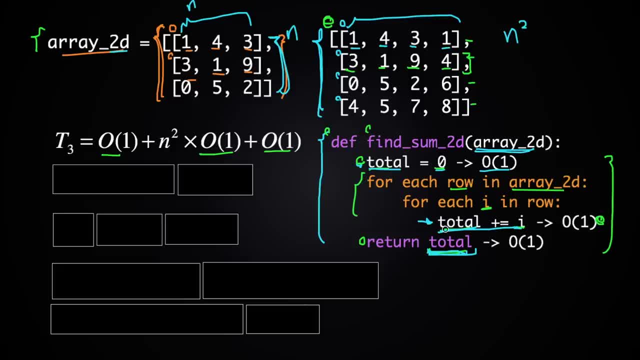 within the double for loop And this line total plus equals i- we need to repeat it- N squared times because there are N squared elements in the given two-dimensional array. So the total amount of time it takes to go through this entire double for loop. 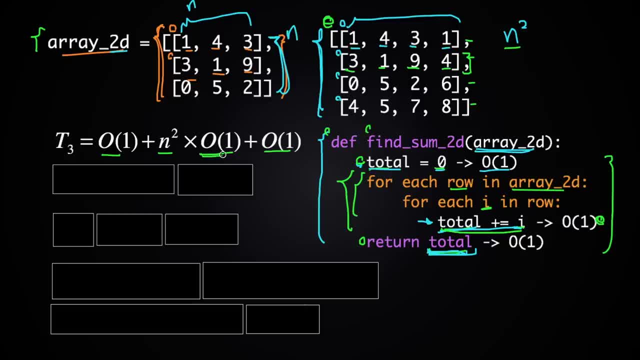 is actually N squared times O of one, And that's actually where I'm simplifying this argument a little bit here, because it takes some overhead to set up each of these for loops And I'm not accounting for that here And that's actually okay here. 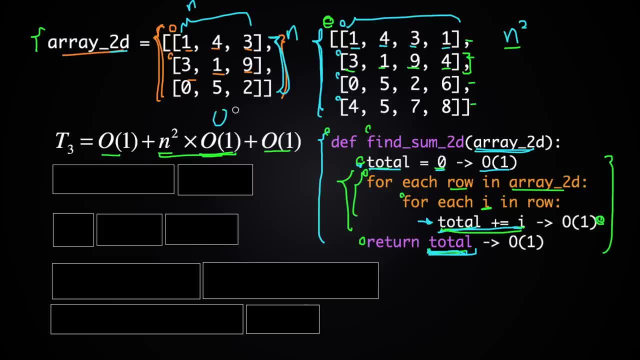 If you wanna account for that, you can add expressions like an extra O of one or N times O of one, And when you do, you will see that the result is gonna be exactly the same. But anyway, let's go with the simplified argument. 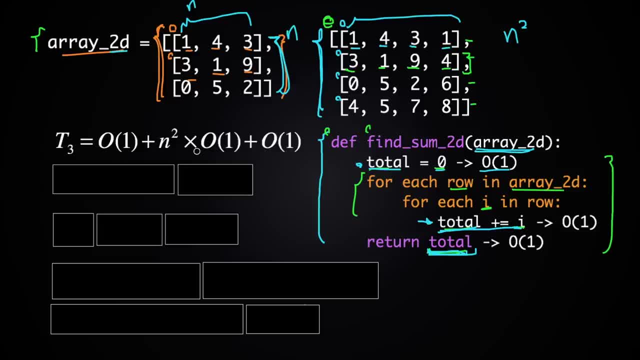 And that's gonna be O of one plus N, squared times O of one plus O of one. These two O of ones at the beginning and at the end come from these two lines at the beginning and at the end of this function. And then this O of one come from this line right here. 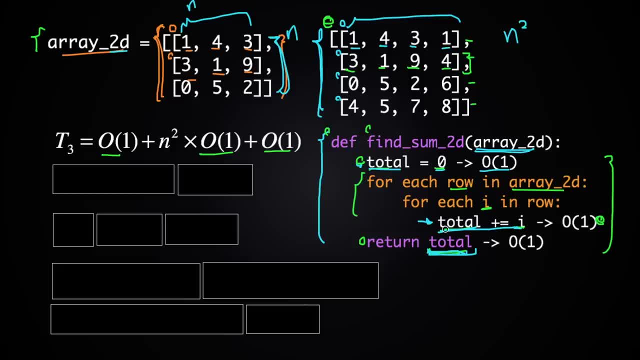 within the double for loop And this line total plus equals i- we need to repeat it- N squared times because there are N squared elements in the given two dimensional array. So the total amount of time it takes to go through this entire double for loop. 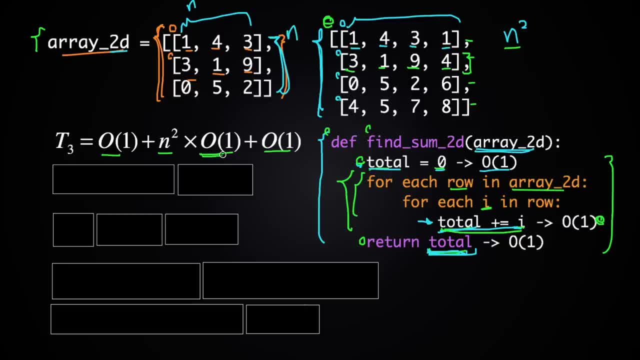 is actually N squared times O of one, And that's actually where I'm simplifying this argument a little bit here, because it takes some overhead to set up each of these for loops And I'm not accounting for that here And that's actually okay here. 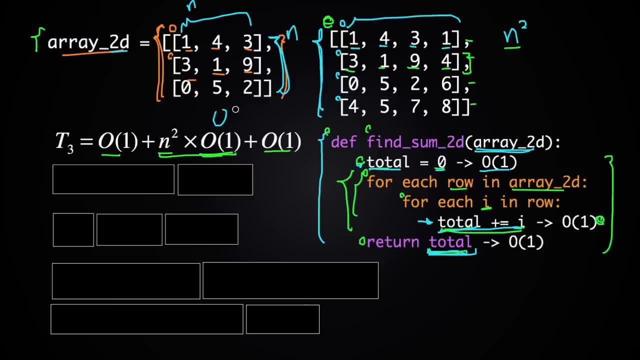 If you wanna account for that, you can add expressions like you know- O of one or N times O of one, And when you do, you will see that the result is gonna be exactly the same. But anyway, let's go with the simplified argument. 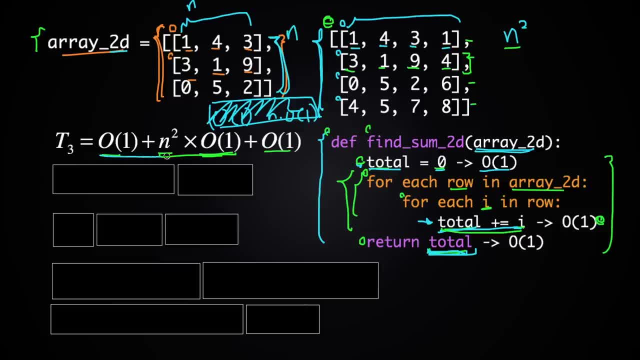 to compute this whole expression. Let's go back to the definition of O, of one. That was just a constant. So we have two constants here. Adding two constants up, we get another constant. Let's call that constant C six, right here. 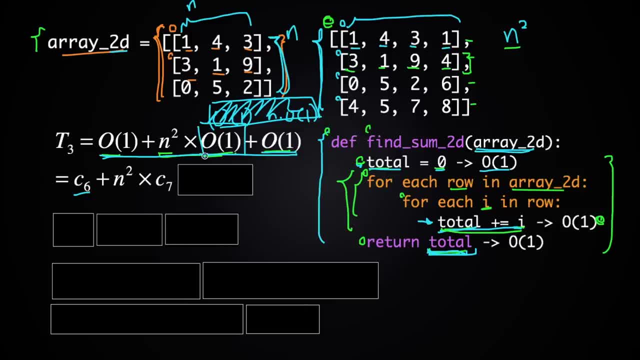 And then let's call this O of one, this constant right here, C seven. So we get T three is C six plus N, squared times C seven, where C six and C seven are constants. And then we can go through the same two-step process. 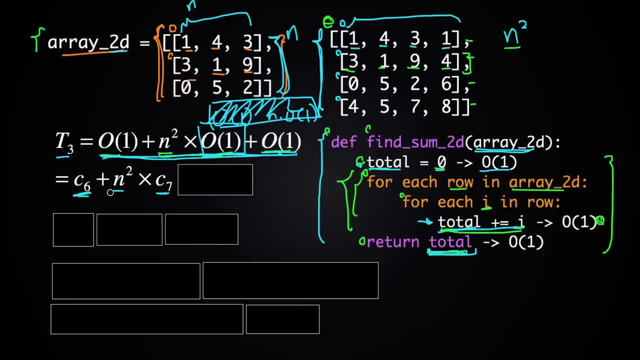 that we used earlier. First find the fastest growing term, That's this term right here: N squared times C seven. And then we need to remove the coefficients, That's C seven. So N squared is what should go inside the big O expression. 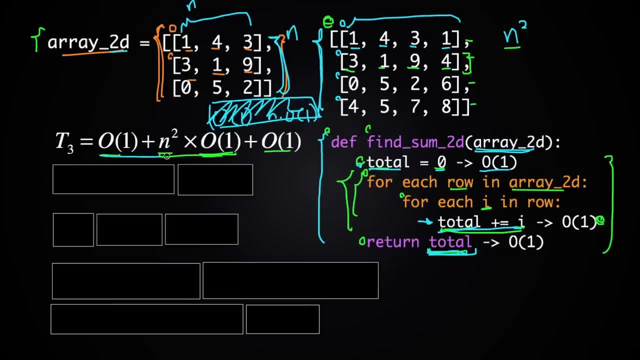 To compute this whole expression. let's go back to the definition of O of one. that was just a constant. So we have two constants here. Adding two constants up, we get another constant. Let's call that constant C six, right here. And then let's call this O of one. 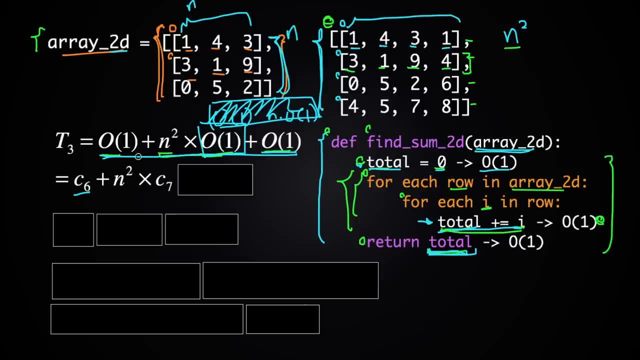 this constant right here, C seven. So we get T three. T three is C six plus N squared times C seven, where C six and C seven are constants. And then we can go through the same two-step process that we used earlier. 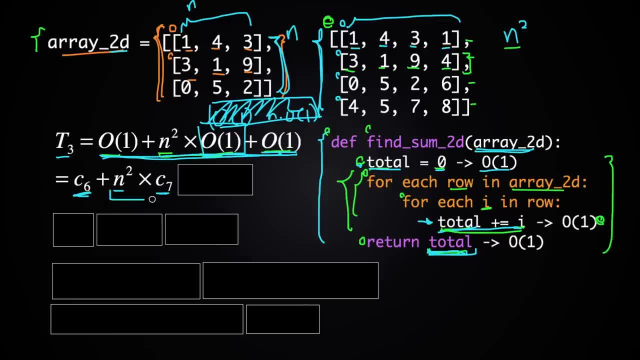 First find the fastest growing term, That's this term right here: N squared times C seven. And then we need to remove the coefficients, That's C seven. So N? squared is what should go inside the big O expression. So we get this is O of N? squared. 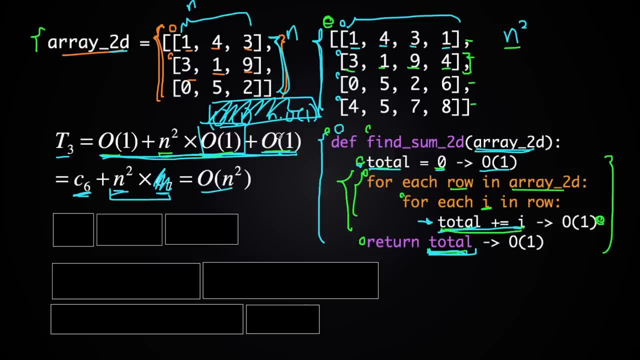 And so the time it takes to execute this entire function. find sum 2D, which is T three, is O of N squared, And that's quadratic time complexity. Okay, so that's basically how you can go about finding the time complexity. 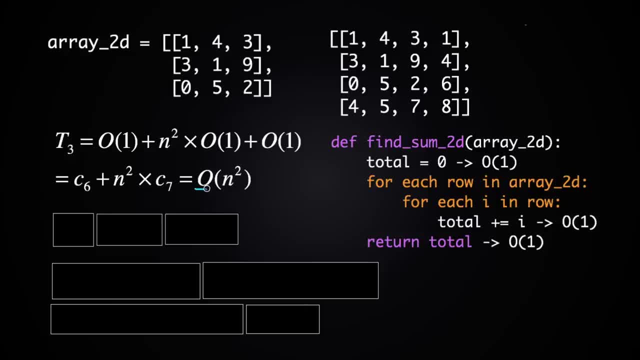 which can be expressed as a big O notation like this one of a somewhat more complex function like this one. Okay, just one more quick example here. What if you had this function right here, find sum 2D, but instead of having just some, you know. some base crop, You multiply by a number just to equal to zero. in other words, find some sum 2D, according to the offer that you have. What if this lambda effectively Sirius frequencies, which gave you one square, just get rid of this is that. 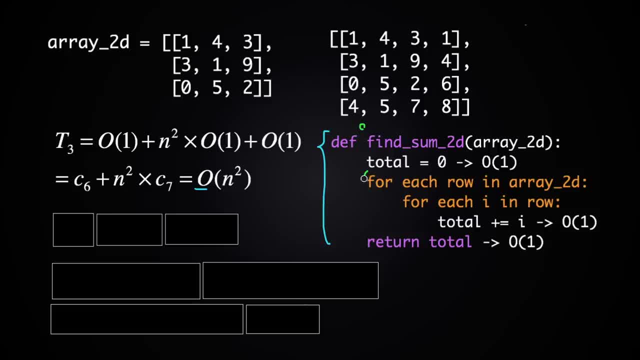 scored down by one day. And then just the next step is what exactly you're able to use to solve this energy and into the real world, having just one double for loop. you had two double for loops And you know those double for loops. let's say, do exactly the same thing. How would that affect the bigger notation? 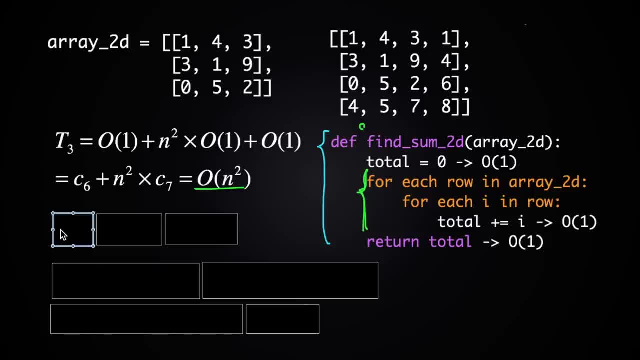 and the time complexity you might say. you know that new time- let's call it t four- is going to be of two n squared, because we need to repeat that double for loop twice, But that's actually equivalent to of n squared. Let's see why that's the case, If we know. 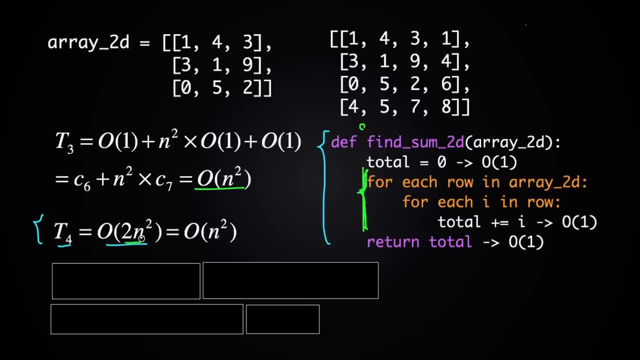 that t four is of two n squared. we can imagine what t four might look like in its full form, And that might look like this: So t four might be equal to something like two n squared times C, which is a constant, and then some other terms. So here what we're saying is that 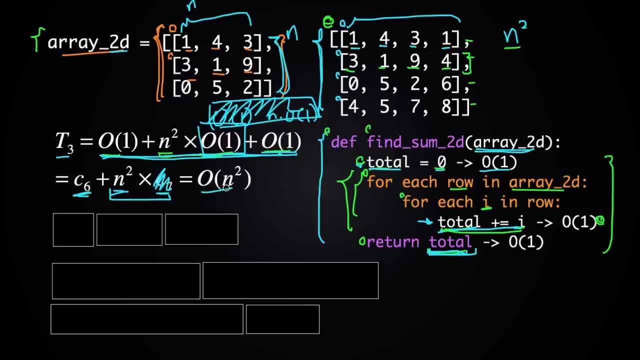 And then we get: this is O of N squared, And so the time it takes to execute this entire function, find some 2D, which is T three is O of N squared, And that's quadratic time complexity. Okay, so that's basically how you can go about. 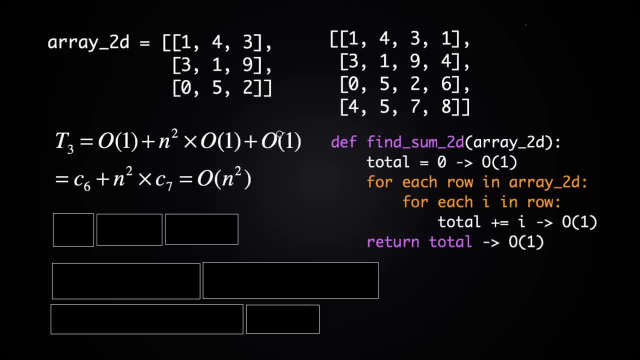 finding the time complexity, which can be expressed as a big O notation like this one of a somewhat more complex function like this one. Okay, just one more quick example here. What if you had this function right here? find some 2D, but instead of having just one, double four loop. 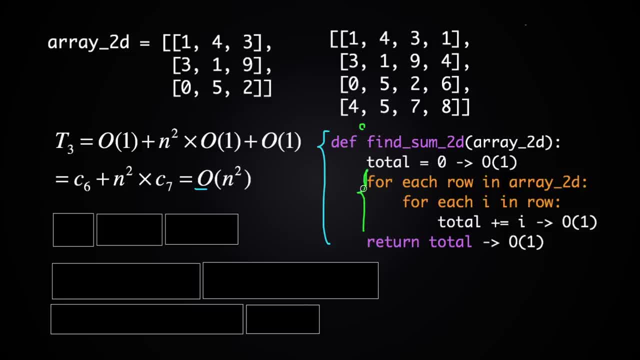 you had two double four loops And you know those double four loops. let's say, do exactly the same thing. How would that affect the big O notation and the time complexity? You might say you know that new time let's call it T four is gonna be O of two N squared. 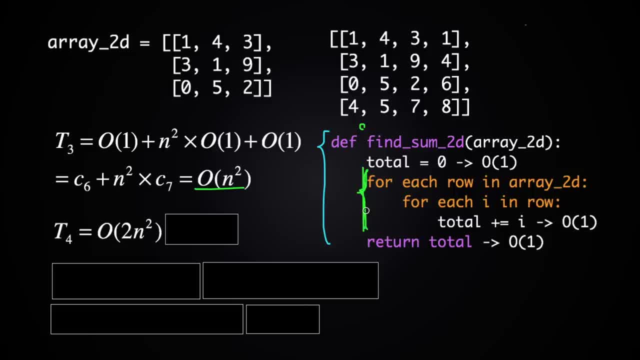 because we need to repeat that double four loop twice, but that's actually equivalent to O of N squared. Let's see why. Here's the case: If we know that T four is O of two N squared, we can imagine what T four might look like in its full form. 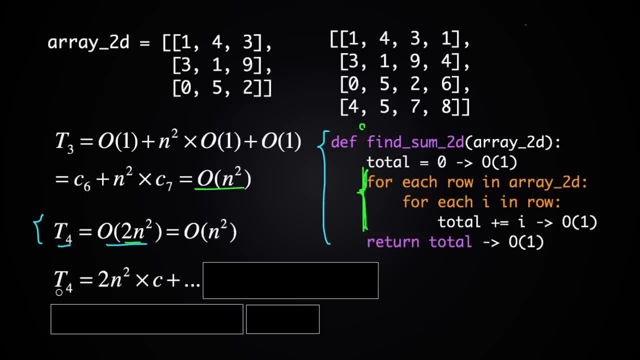 And that might look like this. So T four might be equal to something like two N squared times C, which is a constant, and then some other terms. So here what we are saying is that whoever came up with this big O expression for T four must have said: 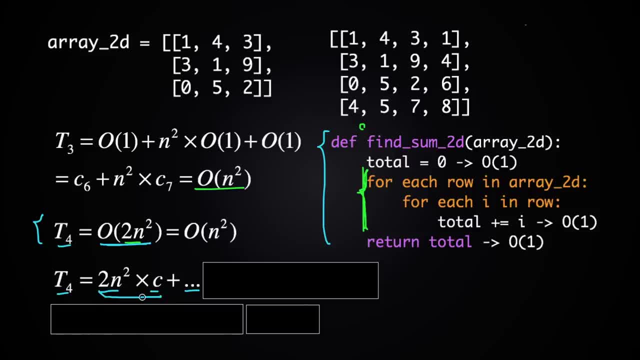 that this term is the fastest growing term: T? N squared times C. And then they must have said: okay, you know, remove the coefficient C. and then we get T? N squared as what should go inside the big O expression And further we might imagine what the rest of the terms. 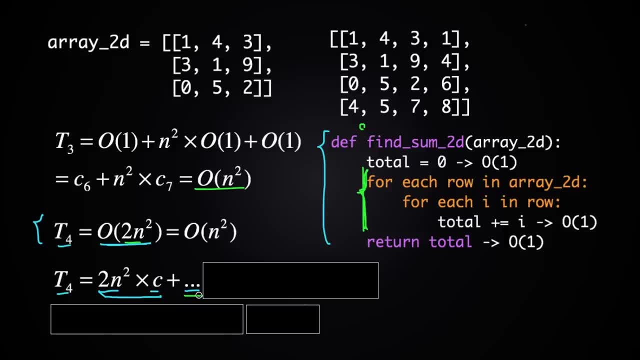 might look like In reality. we don't necessarily know, but as an example they might look like this. So here we have two N squared times C, which is the fastest growing term, And the rest of the terms must be slower growing terms. 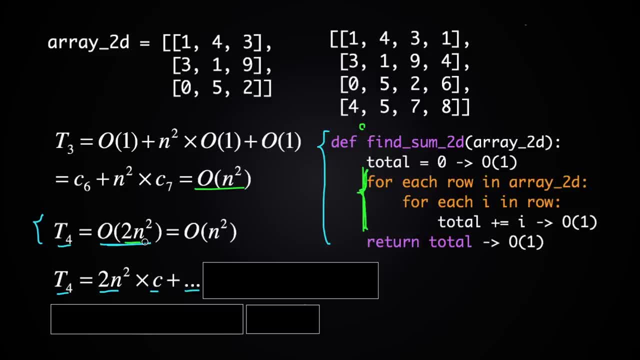 whoever came up with this big O expression for t four must have said that this term is the fastest growing term, t? n squared times C. And then they must have said: okay, you know, remove the coefficient C. and then we get t? n squared as what should go inside the big O expression, And further we might imagine. 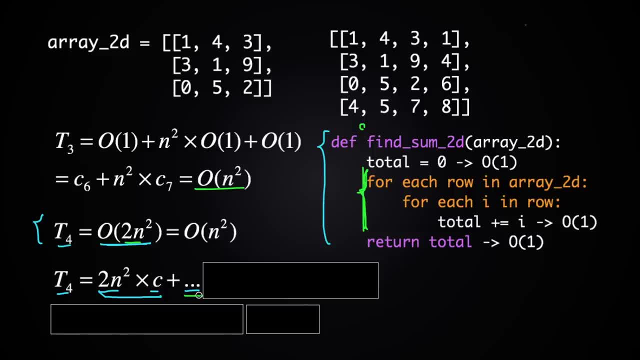 what the rest of the terms might look like In reality, we don't necessarily know, But as an example they might look like this. So here we have two n squared times C, which is the fastest growing term, And the rest of the terms must be slower growing terms. 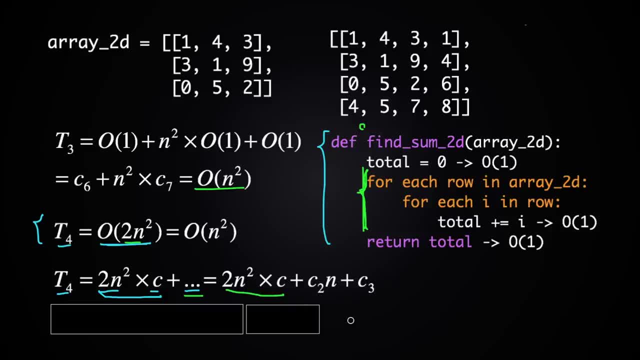 than the fastest growing term. Instead, you know, there might be something like c two, n plus c three, where c two and c three are constants. And if you had something like that, two n squared times C is going to be the fastest growing term, And that means that when n is large enough, this term is 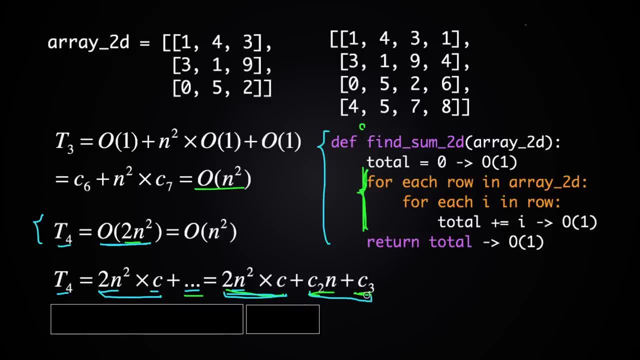 going to be much larger than any of the rest of the terms. But actually here you might notice that you can rewrite two n squared times C this way. So I just rewrote two n squared times C as two C times n squared And looking at this way, the coefficient of 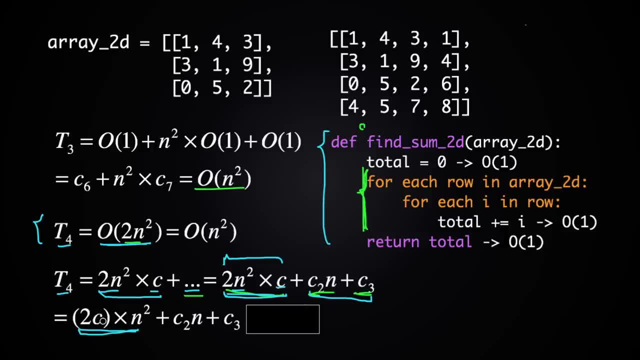 this fastest growing term is not C, but it's actually to see. So taking that off, you can say: well, n? squared is actually what should go inside the big O expression. So t four is actually O of n? squared. So what I showed here is that if we know that t four is O of 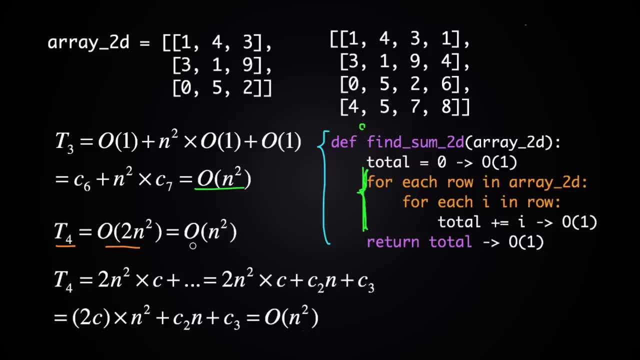 two n squared- it's actually also n squared and actually of 2n squared and of n squared are technically equivalent. so technically you could use either one to show that t4 is quadratic time. but by convention we usually use the one with no coefficients attached to it. so in this particular case that's of n squared and not 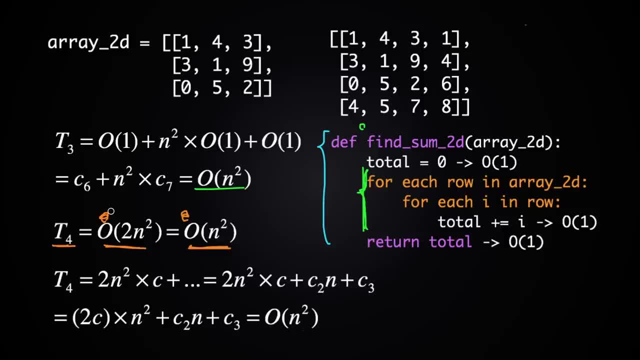 of 2n squared or 3n squared or of 4n squared, even though they're all equivalent. okay, and the argument i used here is not the most mathematically rigorous one, but it's actually good enough for all practical purposes. and that wraps up my introduction to big O notation and time complexity. 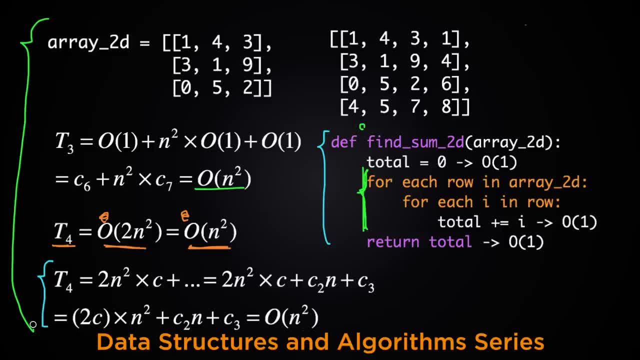 this was actually part of my data structures and algorithm series, so, just in case you want to check it out, i'm going to put a link to the entire series in the description below. now, if you're looking for a more in-depth discussion on big O notation, i'd recommend this video's sponsor's. 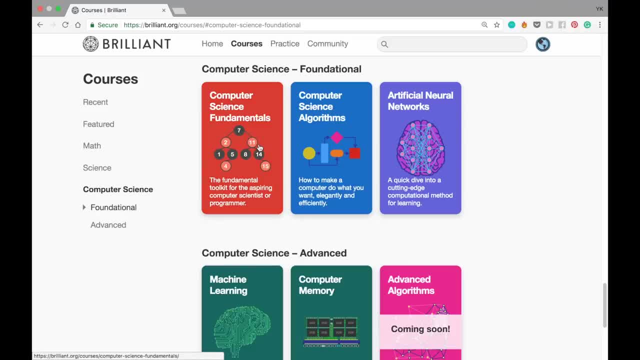 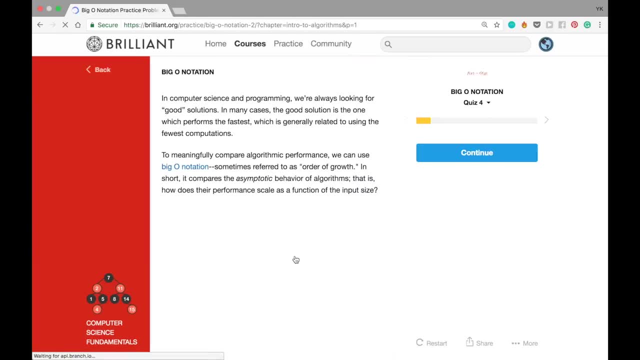 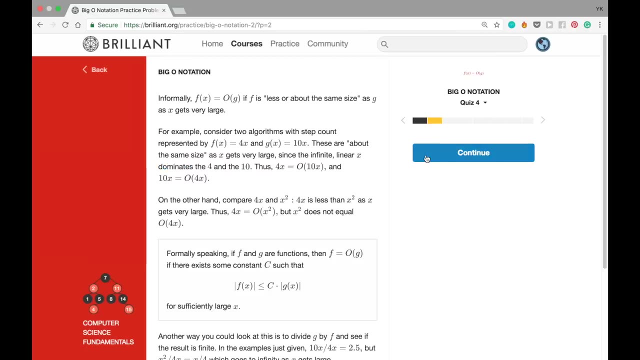 website brilliantcom. in their computer science fundamentals course they have a section about big O notation and it covers some of the mathematical details i skipped over in this video. you know, solving problems is really the best way to solidify the computer science knowledge you've gained from things like books and videos. 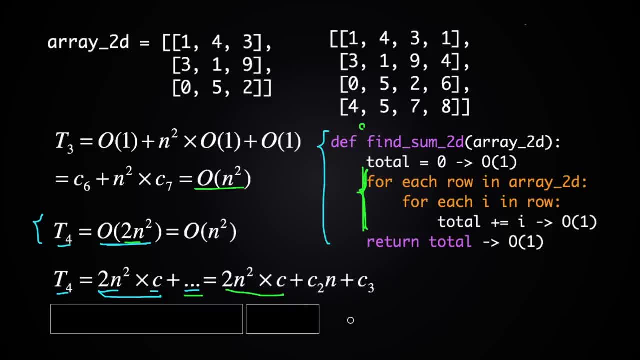 than the fastest growing term. So we said: you know, there might be something like C two, N plus C three, where C two and C three are constants. And if you had something like that, two N squared times C is gonna be the fastest growing term. 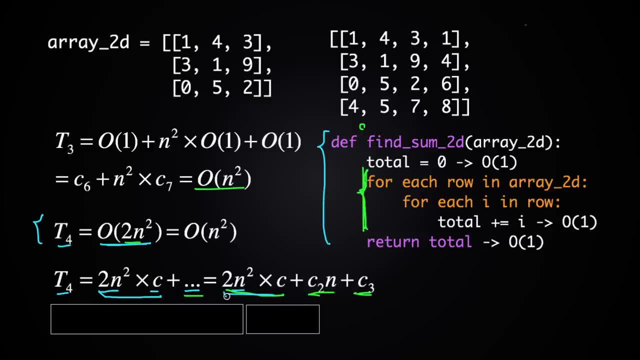 And that means that when N is large enough, this term is gonna be much larger than any of the rest of the terms. But actually here you might notice that you can rewrite two N squared times C this way. So I just rewrote two N squared times C as two C times N squared. 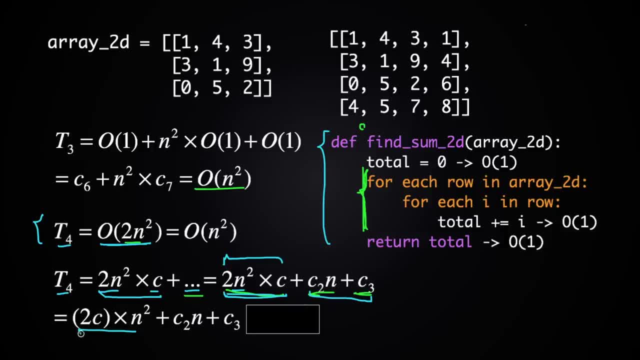 And looking at this way, the coefficient of this fastest growing term is not C, but it's actually two C. So taking that off, you can say: well, N squared is actually what should go inside the big O expression. So T four is actually O of N squared. 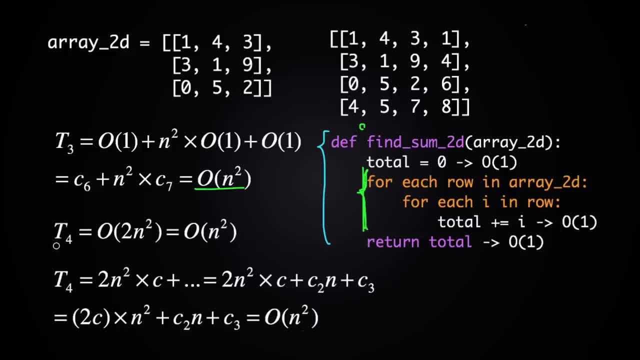 So what I showed here is that if we know that T four is O of two N squared, it's actually also O of N squared, And actually O of two N squared and O of N squared are technically equivalent. So technically you could use either one to show that T four. 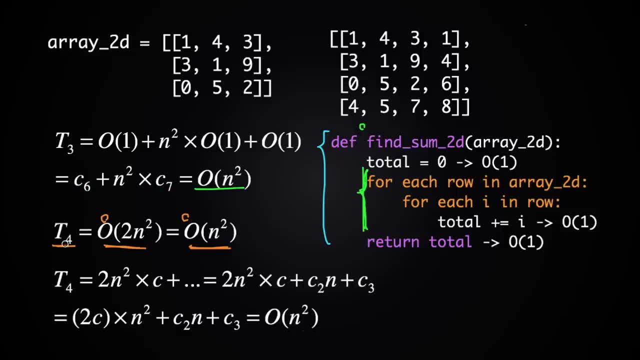 is quadratic time, but by convention we usually use the one with no coefficients attached to it. So in this particular case that's O of N squared and not O of two N squared, O of three N squared or O of four N squared, even though they're all equivalent. 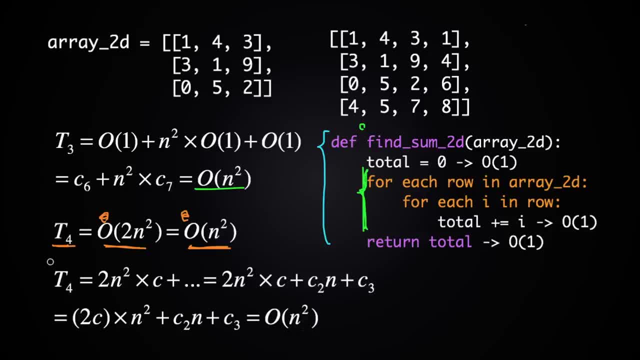 Okay, and the argument I used here is not the most mathematically rigorous one, but it's actually good enough for all practical purposes. And that wraps up my introduction to big O notation and time complexity. This was actually part of my data structures. 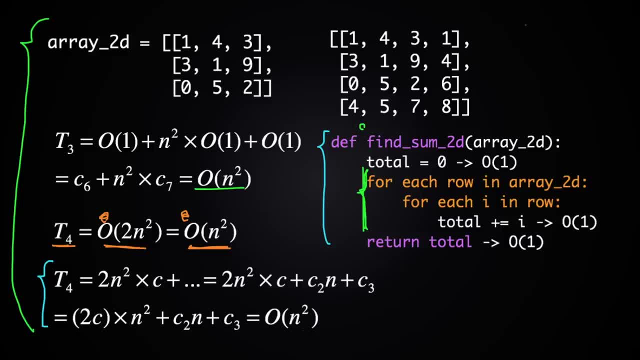 and algorithm series. So just in case you want to check it out, I'm going to put a link to the entire series in the description below. Now, if you're looking for a more in-depth discussion on big O notation, I'd recommend this video's sponsor. 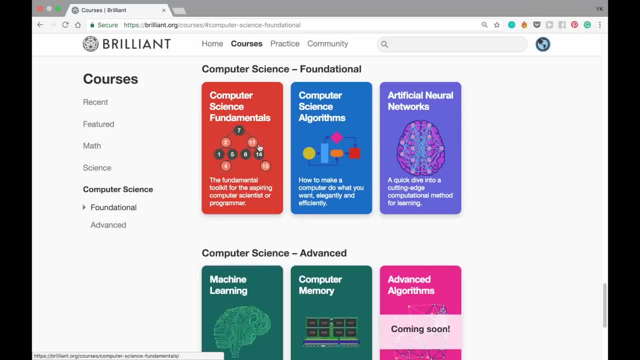 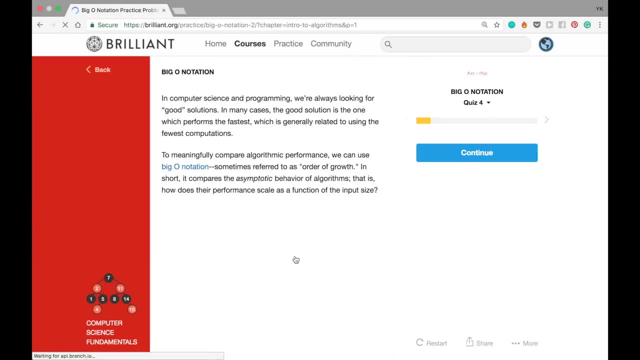 their website, brilliantorg. In their computer science fundamentals course they have a section about big O notation and it covers some of the mathematical details I skipped over in this video. You know, solving problems is really the best way to solidify the computer science knowledge. 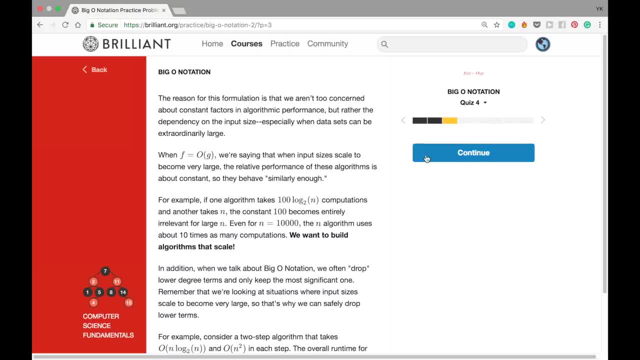 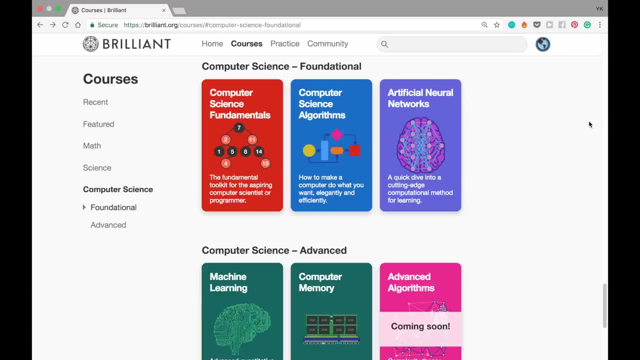 you've gained from things like books and videos, And I would say Brilliant is one of the best resources out there for doing exactly that. So if you want to check out their courses on topics like computer science, fundamentals computer science and the like, you can check it out here. 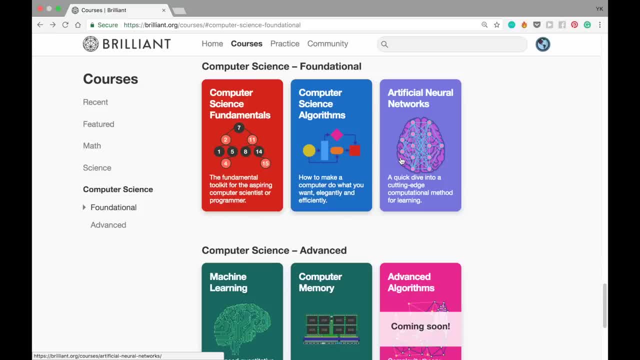 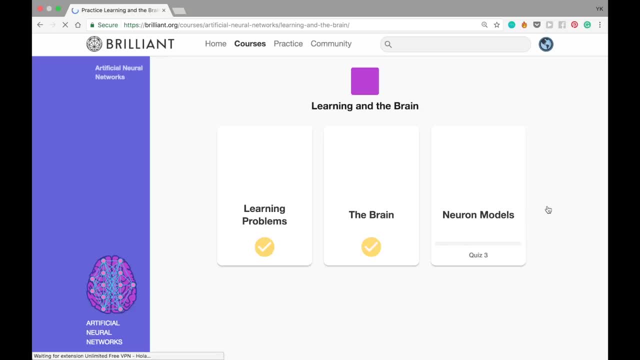 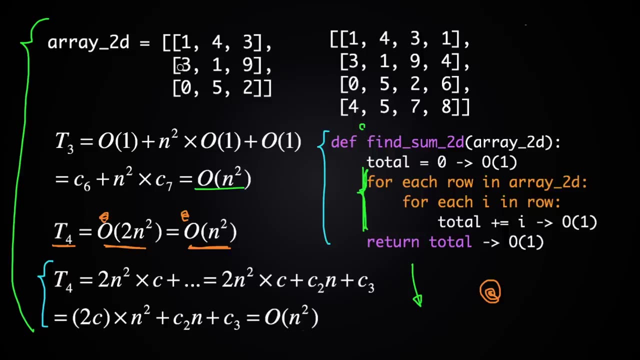 Fundamentals, algorithms and even artificial neural networks. Just go to brilliant org slash CS dojo. Going through that link will let them know that you came from here and the first 200 people can get 20% off their annual subscription through that link as well. Okay, thanks as always for watching and so sorry for the delay on this video, but hopefully I'll see you in the next video.